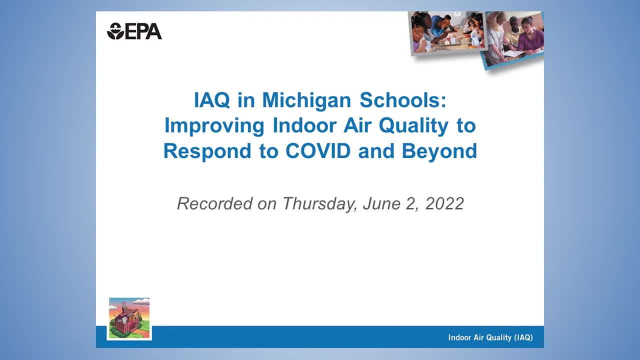 planned this session alongside experts in Michigan, including representatives from Michigan's governmental agencies, school districts and non-governmental organizations. I'm going to get into the goals for the session in just a moment, but first I want to point out that my indoor air quality team here in Chicago 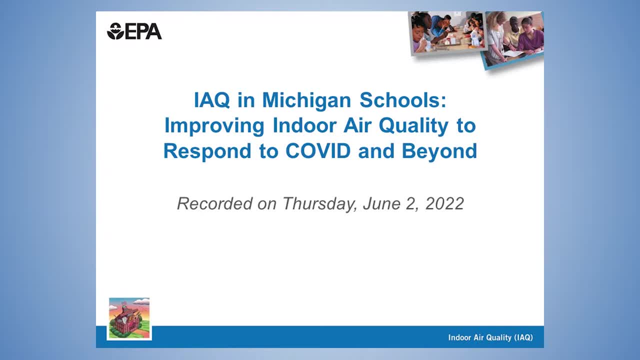 which includes Jeanette Marrero, who will be speaking later in the webinar, Sheila Batka and Monica Paglia. they are a resource for you. in addition to other things we cover today, My experience team has been supporting Michigan partners to address school. 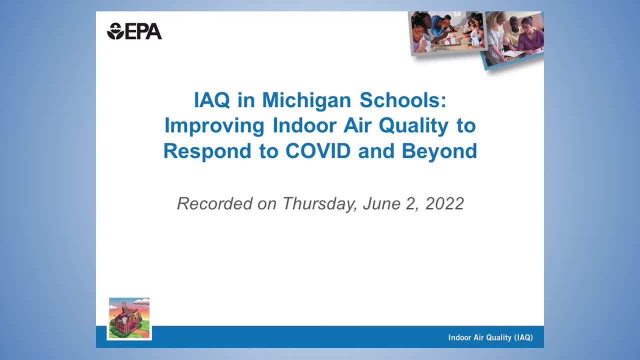 indoor air quality concerns since the 90s, shortly after our Indoor Air Quality Tools for Schools program was launched, So we have very deep experience. here in the regional office We've conducted non-regulatory indoor air quality school assessments and have helped schools identify key indoor air quality. 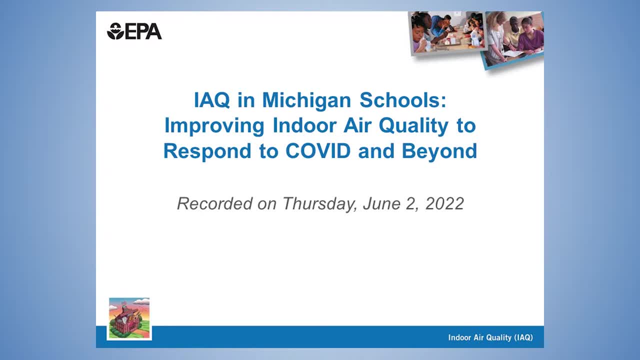 elements in their sustainability, health, safety and facility management plans. And in fact we just returned from Michigan. last week We were in Flint where we did IAQ assessments in three of the schools in Flint with Pete Medore, who will also be speaking later. 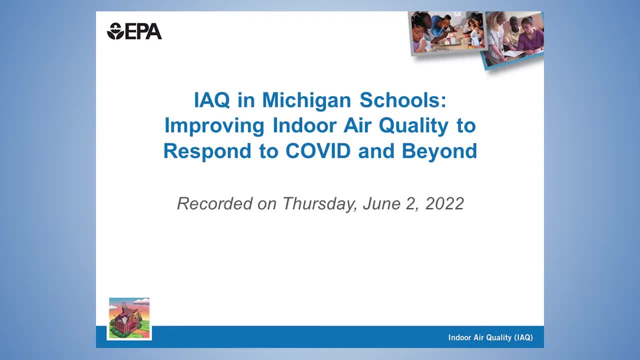 So I just want to point out we have great folks here and we want to be able to help you. One way that you can get in touch with us is filling out the evaluation questions at the end. That's where you're able to tell us where you are with regards to IAQ management and if you're. 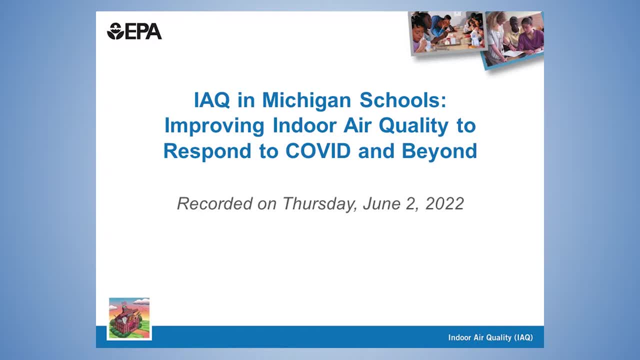 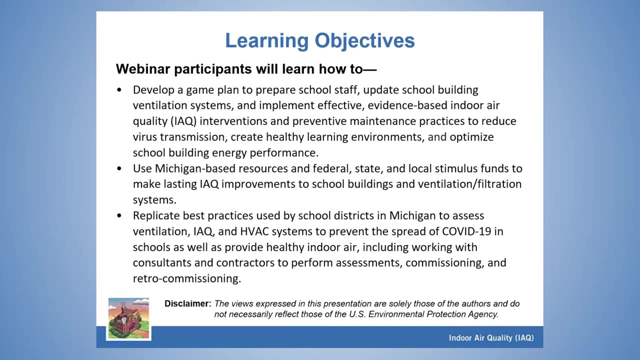 interested in our help And, in addition, our contact information will be included in a follow up material sent after the webinar. So let's get into the objectives. So during the next hour and a half we're going to cover these objectives. First, how to develop a game plan to improve IAQ in your school or district to reduce virus. 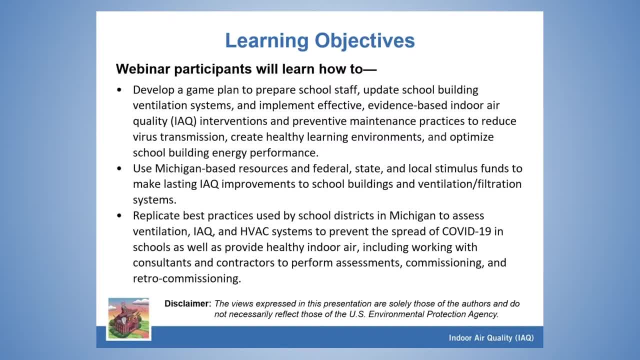 transmission, create healthy learning environments and, as an important co-benefit, optimizing energy performance. We're going to point you to some Michigan specific and federal resources, like funding and assistance, to help you make these improvements to your buildings. Thank you, You guys are welcome to email us. 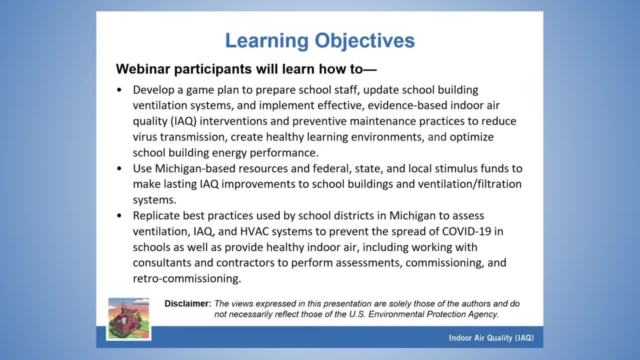 See you in a few minutes. That's really veryn, Aww, Thank you. Bye, bye too. What a day. Bye, bye, Bye and ventilation systems. And finally, the best way to learn is to learn from others' successes and lessons learned. 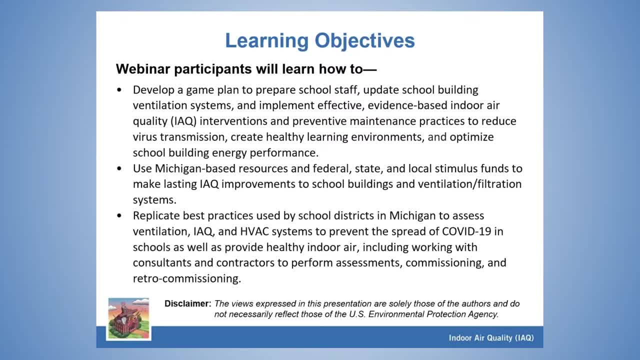 So our speakers will be sharing best practices used by school districts in Michigan, including knowing when it's best to get consultants help to perform assessments, commissioning and retro commissioning. So now we will be talking about our amazing set of speakers, So I'm leaving off. 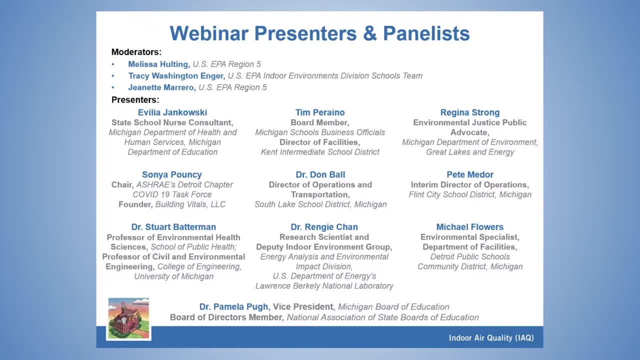 I will be joined shortly by my co-facilitator, Tracy Washington Enger. She is on the Indoor Environments team at EPA headquarters and leads the school's work And, like I said, Jeanette of my team will be speaking later. 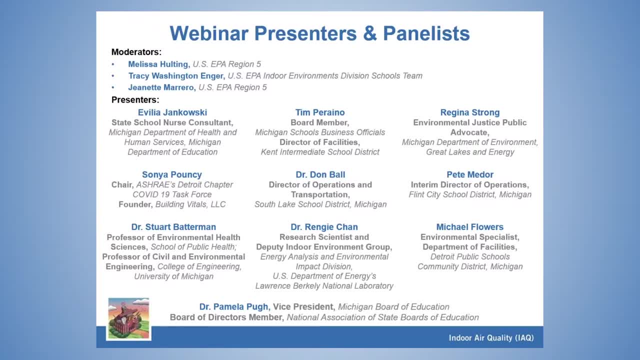 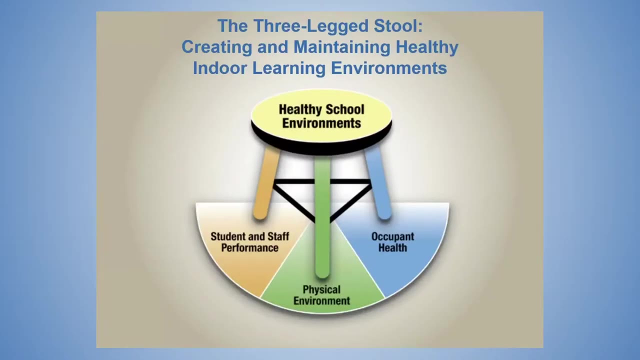 We are so pleased to have this amazing crew of folks who are willing to share their time and perspectives with us today. I'm not gonna read all these names now, but I will introduce them as they speak. So next I'm gonna turn it over to Tracy. 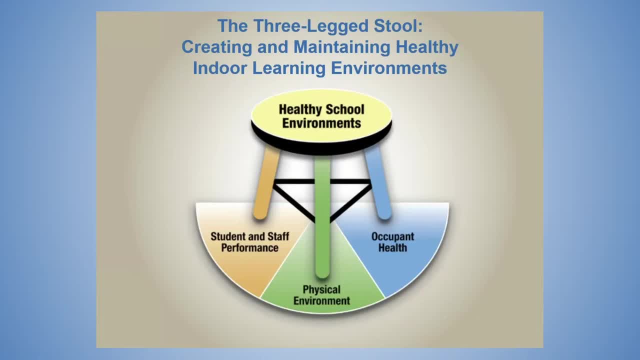 who's gonna give an overview of some of the federal resources and information available. Tracy over to you, Terrific Melissa. thank you so much, and thank you for the opportunity to share with this audience some of the national resources that we have. 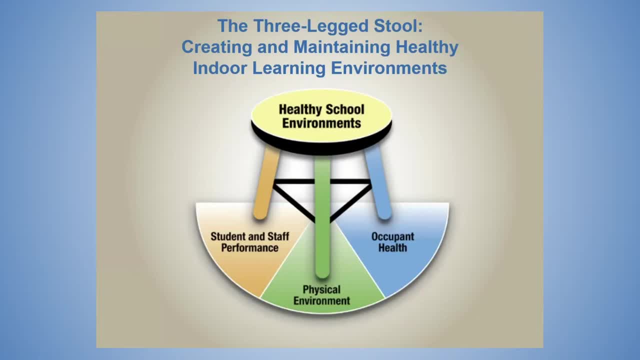 but also, you know so, I'm Tracy Washington Enger. I'm with the indoor environments division at HETCore at EPA and I've been at this work for nearly 30 years and, you know, certainly since we, you know, started the Tools for Schools program and this particular 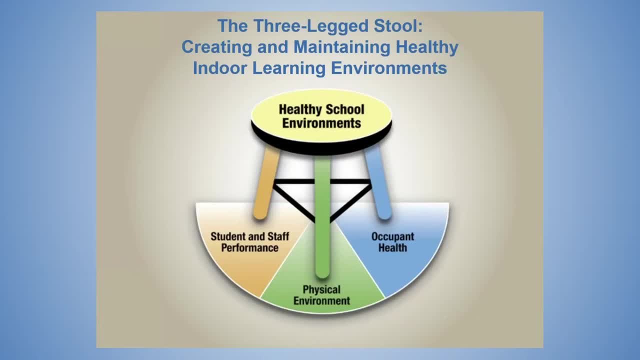 webinar that is really focused on advancing and accelerating the, the efforts within a particular state is something that we have always, you know, been focused on trying to do more, and we in Michigan and region 5, with the partnerships that you have and the strengths of assets, it is just a really 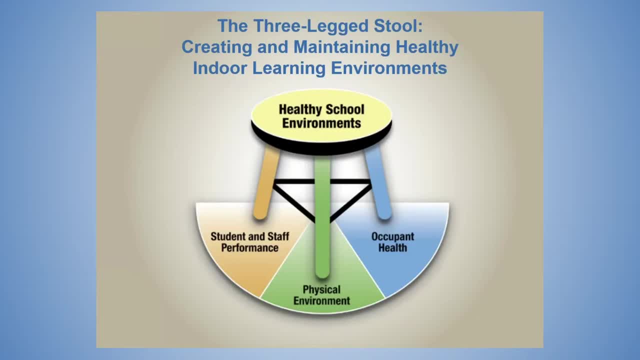 exciting time for us to be engaging and partnering in this way, because you know all of us, those of us who work in with and for our schools. we know that they do much more than just deliver. you know an adequate curriculum for education. we know that where students learn is just as important as what they learn, and a 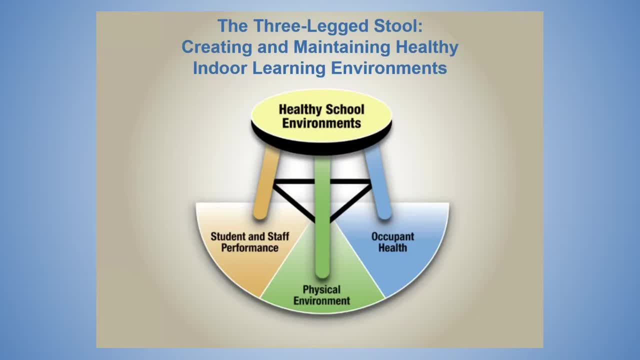 healthy indoor learning environment is really supported by this three-legged stool that you see here of occupant health, student performance and a well-managed physical environment. all of that is essential to schools for them to achieve their primary academic missions, and so our schools, we know over. 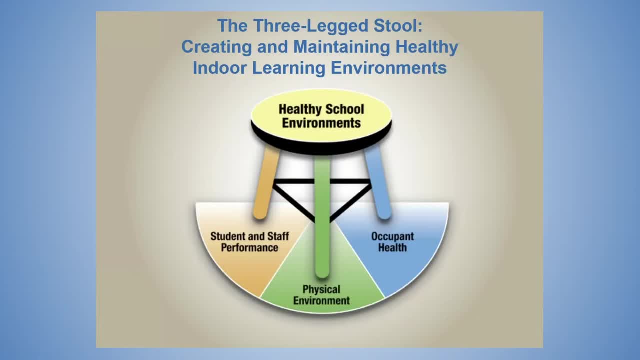 time our schools have really become a social safety net for our communities and providing everything from meals- it's a real- to primary health care when we see, you know, with a school-based health centers. so for many students we know that their school is going to be the cleanest, healthiest, safest place in. 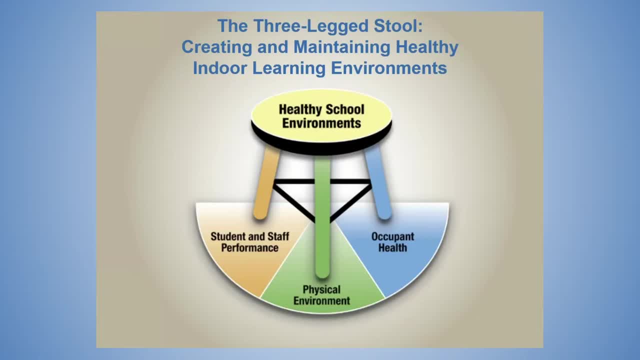 their lives really, and COVID has been really a stark reminder to us of the importance of understanding the connection between the physical environment, health and academic performance in our schools. so you know, even before COVID, students and staff were missing school due to any number of health impacts associated with poor indoor air quality, but especially you. 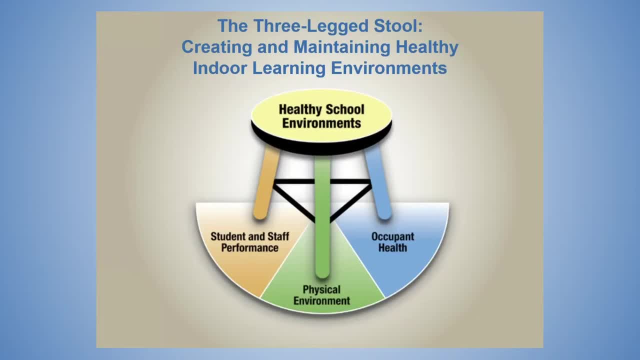 know we, when we look at something like asthma, you know which has is impacted directly by indoor quality. it's the leading cause of school absenteeism due to a chronic condition and it accounts for more than 10 million school school days a year. and when kids are missing that, that that. 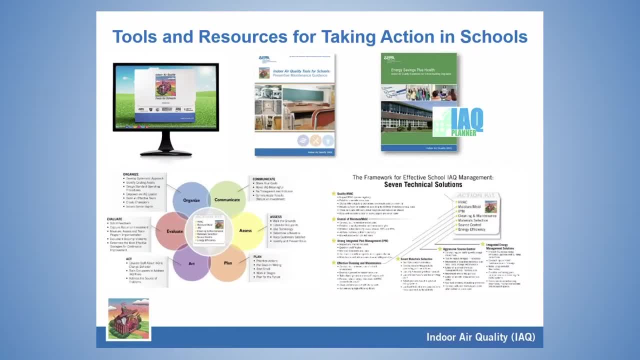 learning. that is not something that they are going to recoup, and so for us it is really important to have resources in place to address that. so at EPA, we do have a wide range of resources to help schools implement comprehensive IAQ management plans that create safer learning environments with using 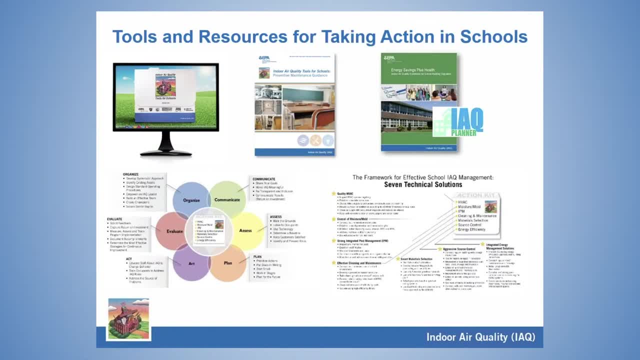 proactive measures while balancing energy efficiency. so the IAQ tools for schools action kit, which you'll hear a lot more about from our from our speakers, was designed to help schools acquire the skills needed to really identify, assess and address and prevent the environmental health issues that negatively impact their school life. 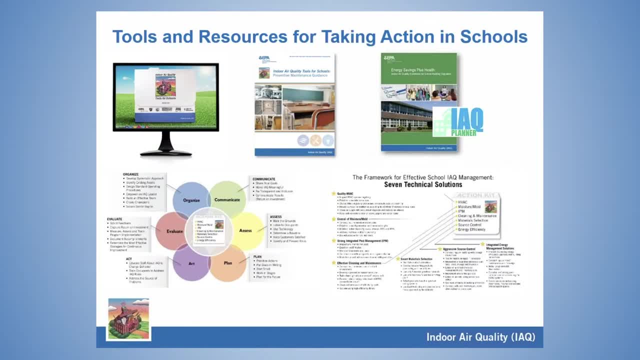 The kit was designed with all kinds of checklists and supporting materials to address the IAQ issues that we find across the, across the nation, in all of our schools, and then for long-term planning and sustained success. we have the. we know that preventive maintenance is essential, taking proactive measures so the indoor quality 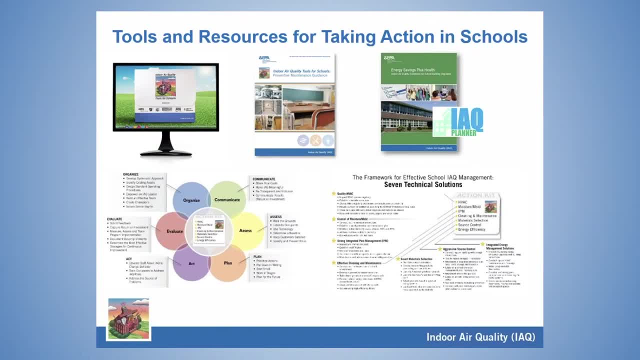 tools for schools. preventive maintenance guidance provides customizable Excel spreadsheets and checklists for all of the technical solutions that we provide, including HVAC source control, cleaning and maintenance, along with inventory sheets, model programs- just everything that you need really to operationalize the recommended activities for really ongoing support throughout the academic. 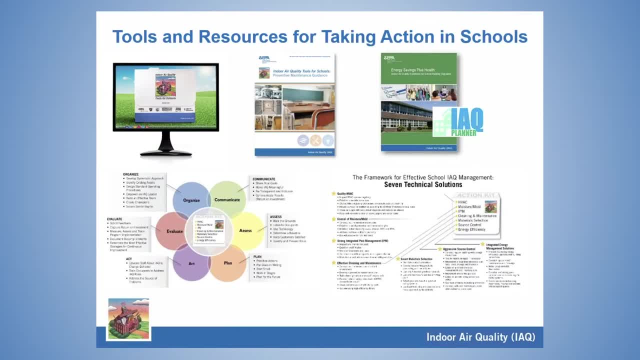 year. but we also know it's important to be addressing energy efficiency as well and how we are, how we're managing energy expenditures in our schools too. so the energy savings plus God plus health guidance document is with this checklist and customizable checklist generator is really a step-by-step guide to repairing and renovating your schools. 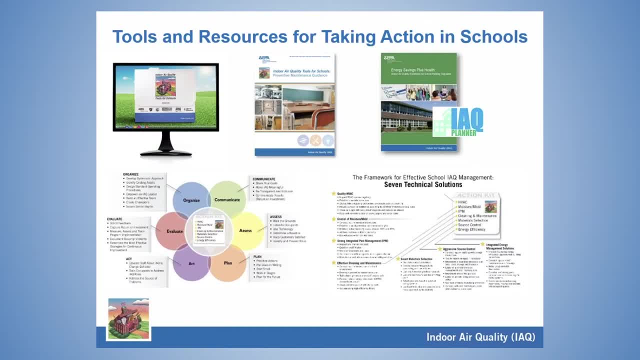 in a way that protects and improves IAQ while maximizing energy efficiency and minimizing costs as well. so all of these are underpinned by our tools for schools framework for effective IAQ school management. and that is six key drivers and successful strategies for continuous improvement. 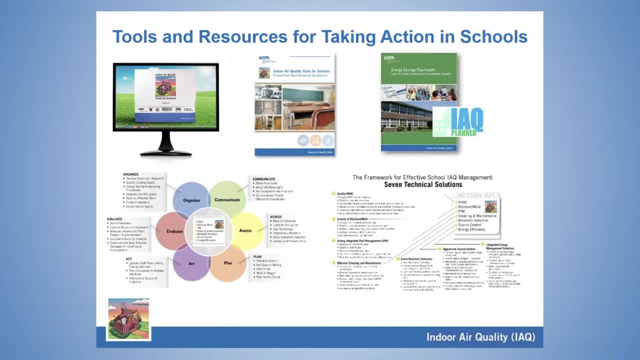 so this framework is especially useful, as we are to help you organize and operationalize all of the different guidance that is coming from various sources right now, especially as it relates to COVID. so this flexible framework can be applied to help you take action on the guidance and you'll be 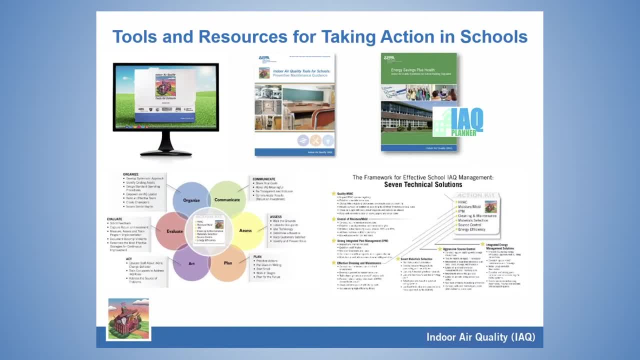 hearing a lot about the strategies under the assessed driver today to help you develop effective and sustainable IAQ plans for your school. in addition to the the key drivers, the kit also offers seven technical solutions, and these are the IAQ issues that the kitten framework are can be used to address in order. 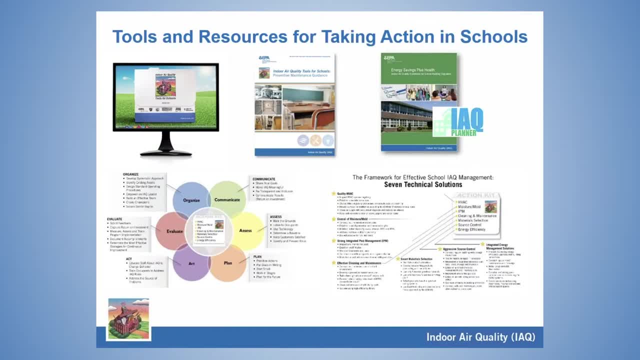 to achieve reliable, clean, efficient and healthy school environments in your schools. so this webinar we're going to take a really deep dive into quality HVAC technical solutions, but you'll also hear from our speakers the importance of you know. in addition to it goes to optimizing ventilation practices. but all of the technical solutions working together concurrently. 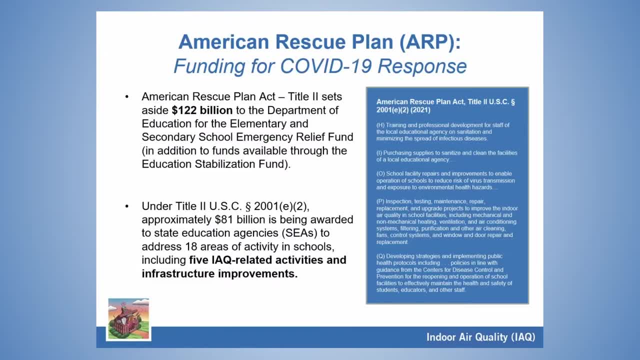 so, especially during this, you know, in response to the COVID, knowing which interventions work best has become even more critical for school districts to capitalize on the increased funding resources that have become available to schools from for COVID response to implement building upgrades, to assess your school facilities and to institutionalize really the most effective IAQ practices. so the 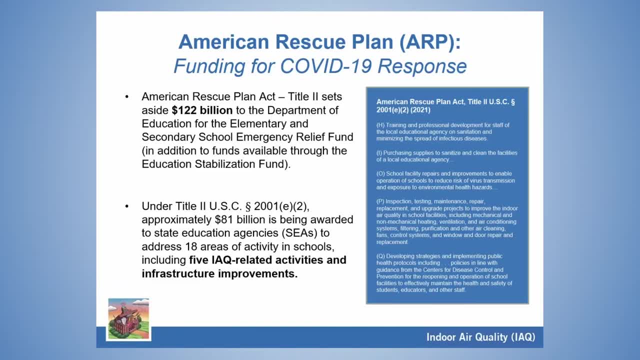 COVID pandemic has been a catalyst for the department of Ed to direct unprecedented levels of funding towards addressing school facilities. I'm sure that some of you have already seen that coming into your school districts. so the American rescue plan provided 81 billion dollars to state educational facilities to address 18 areas of activities. 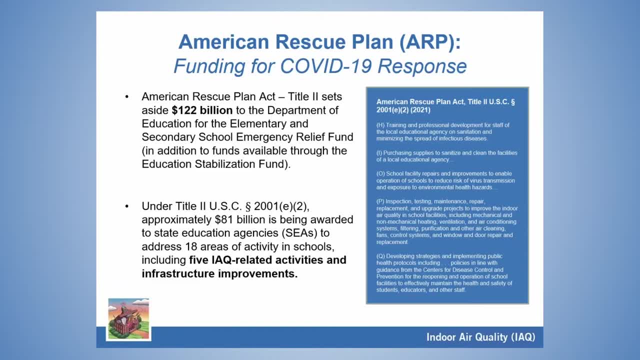 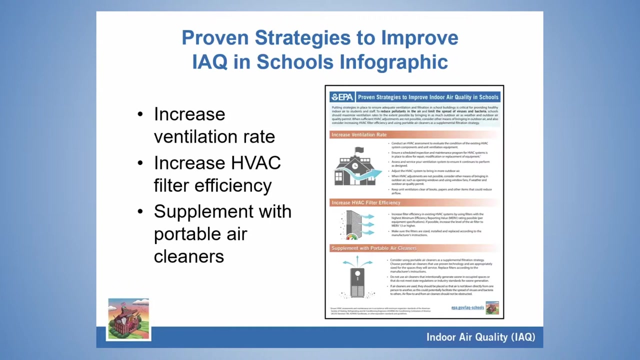 including, really for the first time that we've seen five IAQ related activities and infrastructure improvements, and so this is really a a great opportunity for us to capitalize on on on these funds as we create, as we address building performance and results for for our building occupants. so in, you know, so we at EPA, you know, looking at COVID specifically, so 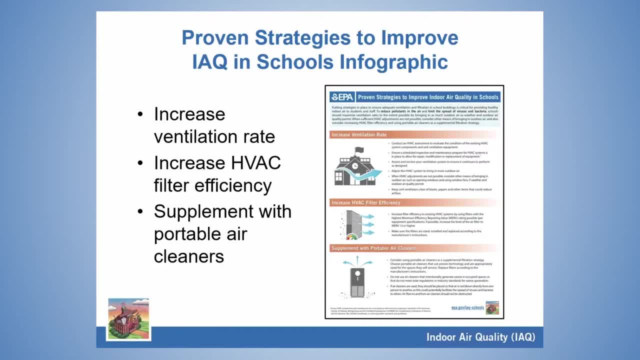 when responding to COVID specifically, school districts have really relied very heavily on the guidance for health and the environment and from building sciences and experts at places like ABC, and most of that guidance really hinges on proven, on three proven approaches for that are increasing ventilation rates, enhanced filtration and supplemental ventilation with portable air. 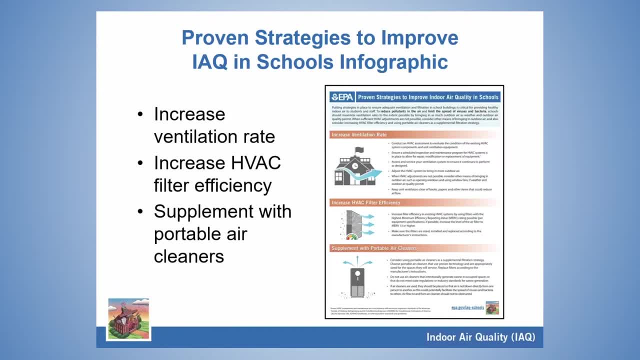 cleaners when needed. so at EPA we developed this technical guidance infographic to help schools operationalize that guidance by providing simple strategies to kind of jump start your IAQ programs and address issues quickly and respond to them, no matter kind of how simple or how complicated they may be. but we know that those are just the beginning and the data that 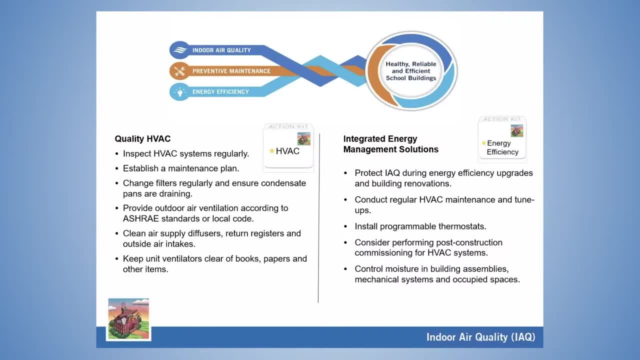 you collect during your assessments is valuable for creating a plan to prioritize action and really applying the technical solutions. so you know, when we look at it, we recognize the the importance of preventive maintenance as well, for addressing deferred issues, as well as energy efficiency and energy management being one of the most lucrative places where 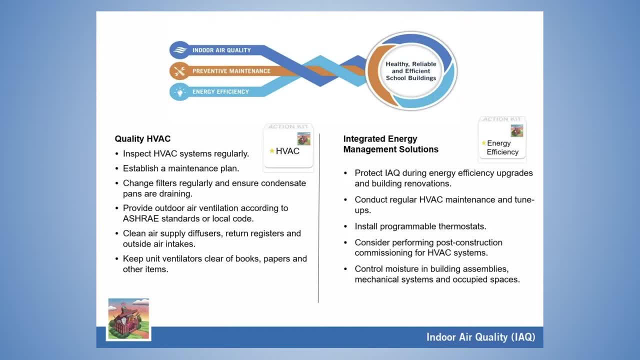 addressing IAQ and deferred maintenance can really pay off. so preventive maintenance has a tremendous range of benefits and our focus really is on that dynamic interconnection of indoor air quality, preventive maintenance and energy efficiency, because one of the things that we know is that you know they're making that connection between health, quality HVAC and 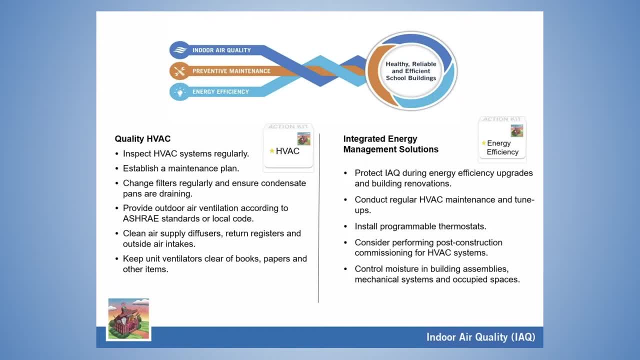 energy efficiency, those technical solutions, is how we begin to debunk this false dichotomy between energy efficiency and good indoor air quality. they really are two sides of the same coin, and that coin is creating healthy school environments. so we're going to be talking. you're going to be hearing our speakers talk a lot about you know. 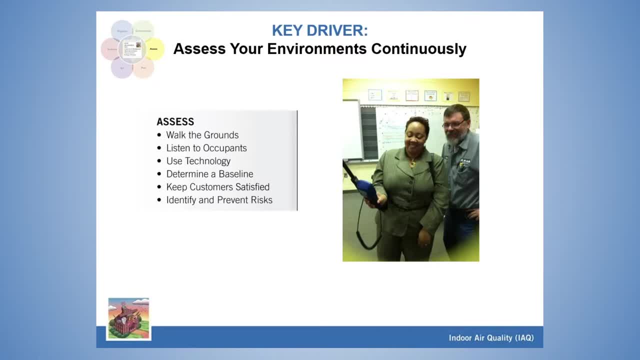 how you really put in place the strategies associated with the assessed driver key driver, and it's also how you can validate your program efforts and where you conduct one of the most important actions for your IAQ management plan, which is the tools for which- is the school assessment walkthrough. and during these walkthroughs, you 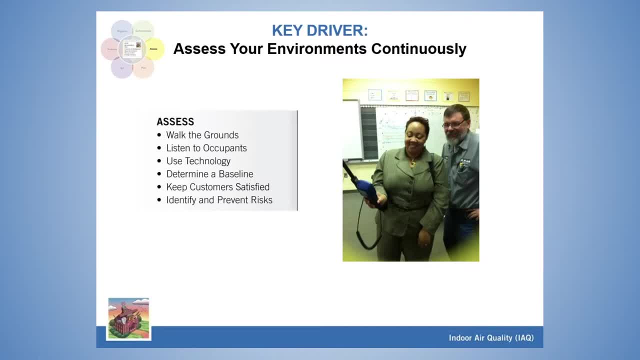 can collect data and identify needs and really prioritize your program. and you're also kind of being assessed by your- by your occupants- while you're doing it as well. so it's a great opportunity to hear directly from your occupants and to support them- to support them and build your. 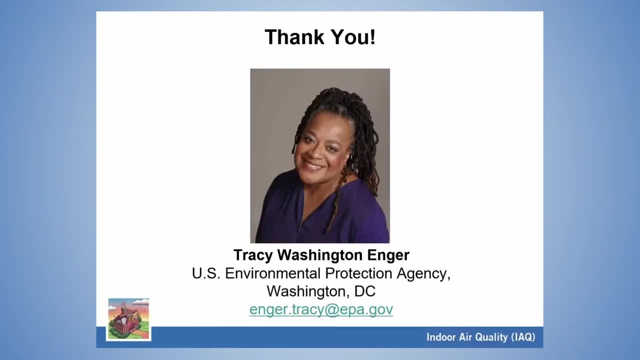 program. so that's just, you know, a beginning to, to give you an idea of of what we at the national staff provided and what is being tailored specifically by your regional, by your region 5 staff, as they interact with school districts directly in Michigan, who you're going to be. 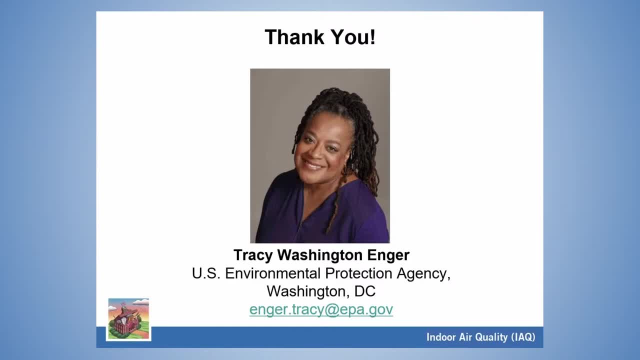 hearing from and how they are applying all of these key drivers, addressing these technical Solutions and getting and getting great results. so it is my pleasure to be with you here today. I will see you again on the other end, at the Q a and, in the meantime, at put your questions. 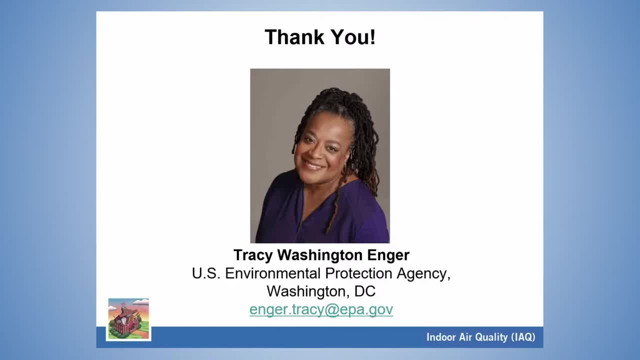 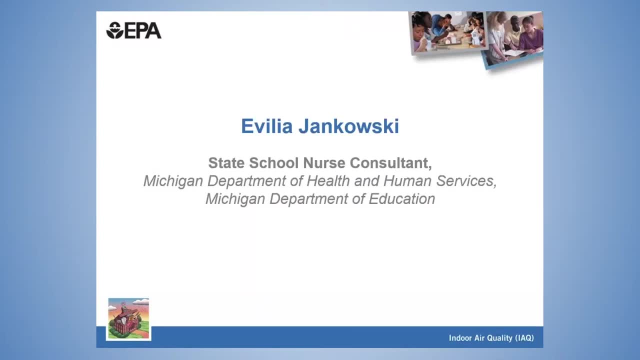 into the, into the chat function, and we'll be excited to respond to them as at the at the end of the webinar. but thank you so much, Melissa. I'll turn it back over to you all, right, so we will now get into it and I'm gonna transition now to our first. 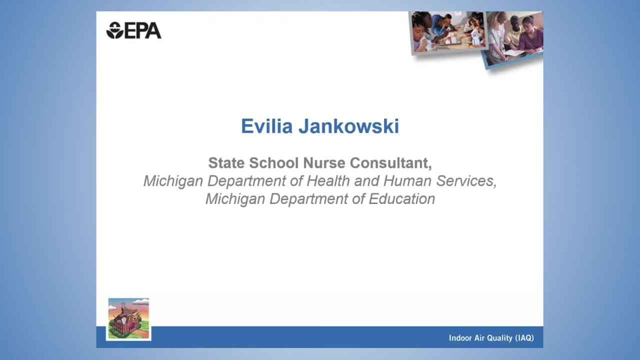 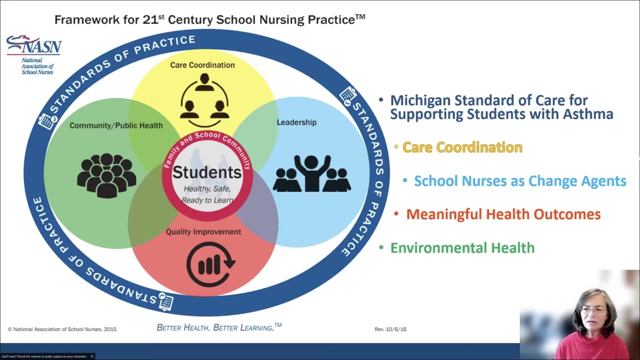 speaker Avelia jankowski. she is the state school nurse consultant for both the Michigan Department of Health and Human Services and the Michigan Department of Education. hello, my name is Avelia jankowski. I am the state school nurse consultant for Michigan. I spent the last 30 years of my 42. 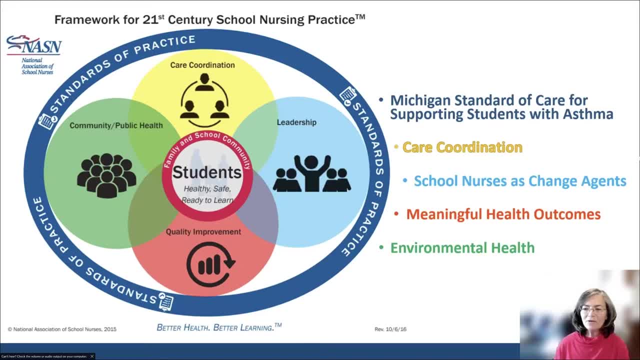 year nursing career as a school nurse. you may wonder how school nurses fit into this important topic. the National Association of school nurses framework for the 21st century school nurse practice provides a graphic illustration of the key principles of professional school nursing practice. the framework provides guidance for the practicing school nurse to reach the goal of 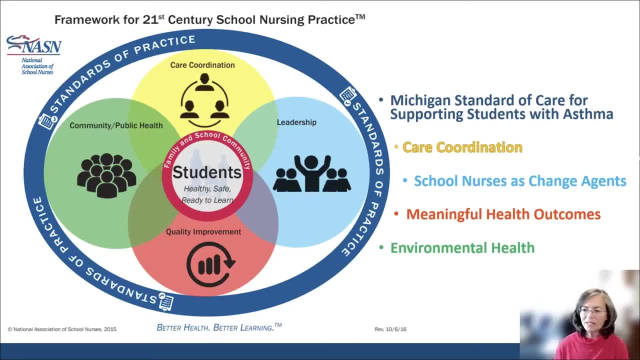 student success and academic success by contributing to a healthy and safe school environment. you can see the student is at the center of our model. our goal is for that student to be healthy, safe and ready to learn. family and school community surrounding the student influenced the students ability for academic success. surrounding the family and the student. and 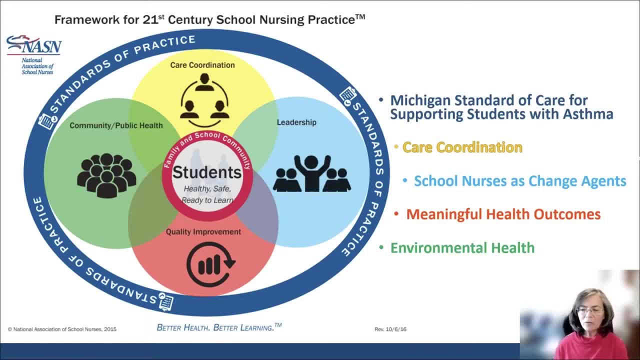 the school community are overlapping key principles of care, coordination, leadership, quality improvement, community and public health. These principles are guided by the fifth principle overarching, which is the foundational for evidence-based, clinically competent, quality care, the standards of practice. School nurses use the skills outlined in each of these principles to help students. 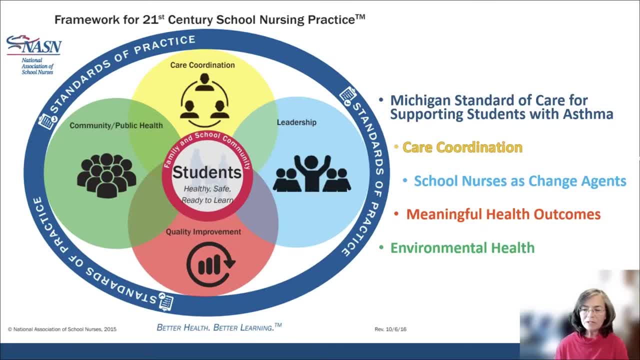 to be healthy, safe and ready to learn throughout their workday. The standard of practice that reflects best practice when we are supporting students with asthma comes from a variety of professional resources: The EPR-3, or expert panel review updates that were released last. 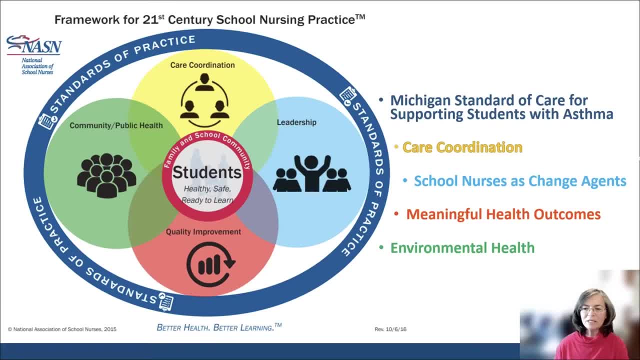 year promote more attention than ever at addressing asthma triggers in the environments where individuals with asthma live, work and learn. The SAMPRO, or School Asthma, Allergy and Anaphylaxis Management Program, also calls for addressing asthma triggers. 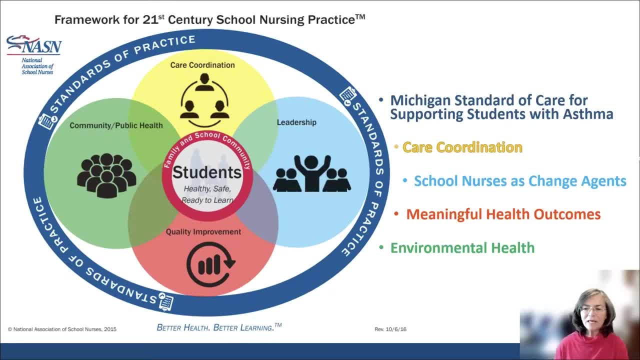 Michigan's Department of Education has taken the cue from these evidence-based resources to update the model policy for supporting students with asthma to include more attention to mitigating asthma triggers. In fact, the school nurses' standards of care for supporting students with asthma in Michigan closely follow the MDE policy and will promote a more concerted 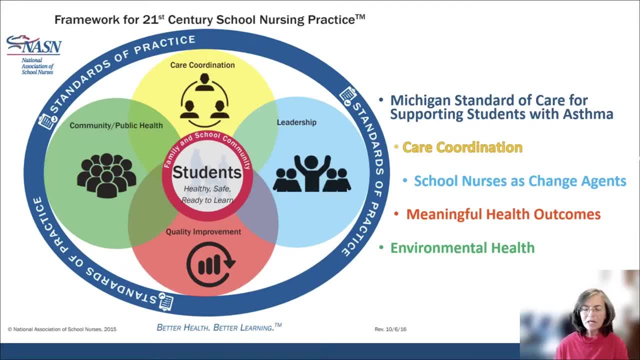 effort to addressing asthma triggers. To improve health and academic outcomes for students with asthma, they must first be identified. In Michigan we generally see three students with asthma in a class of 30. Once we know who the students are with asthma and what their triggers, 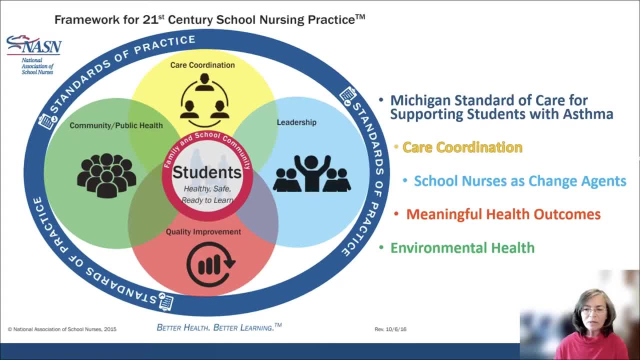 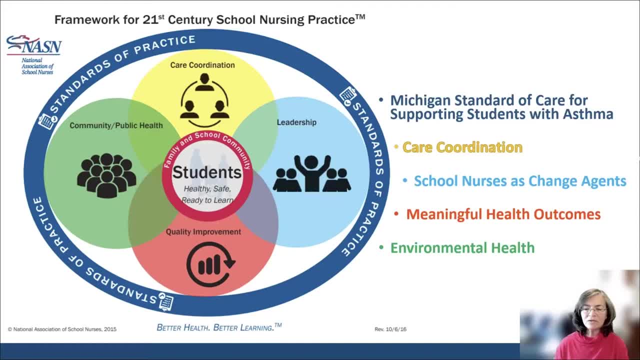 provide care coordination for students with health needs in school Care coordination interventions for students with asthma include decreasing opportunities for exposure to triggers by actually mitigating those triggers. This means that the school nurse often provides leadership, as they are the change agents who bring school colleagues together. 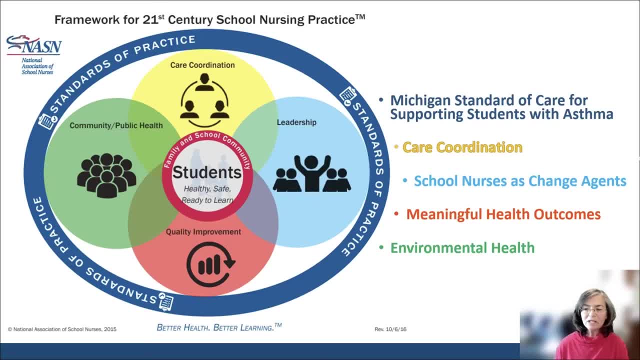 from the administration to teachers, to custodial staff, to identify strategies and resources to mitigate triggers. COVID has actually been quite helpful in making everyone aware of the need for good air quality. This framework supports the school nurse to lead or join in the efforts to 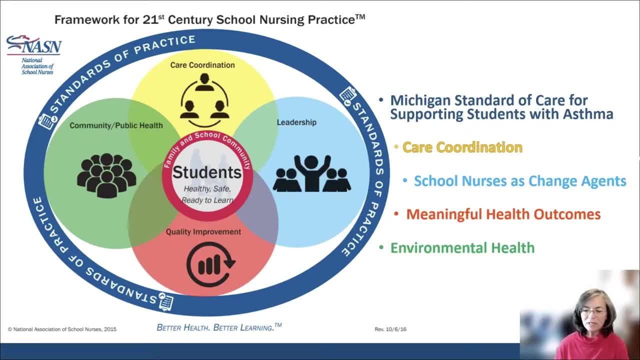 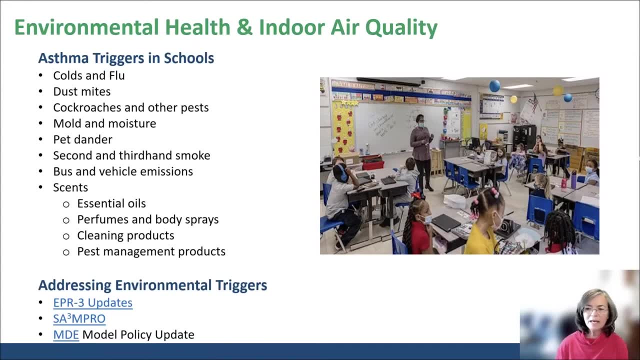 address environmental health efforts like integrated pest management, promoting electric school buses and no idling policies. There are many asthma triggers that affect the environmental health and air quality in our schools. Triggers like exposure to colds and flu virus, dust mites, second and third hand smoke. 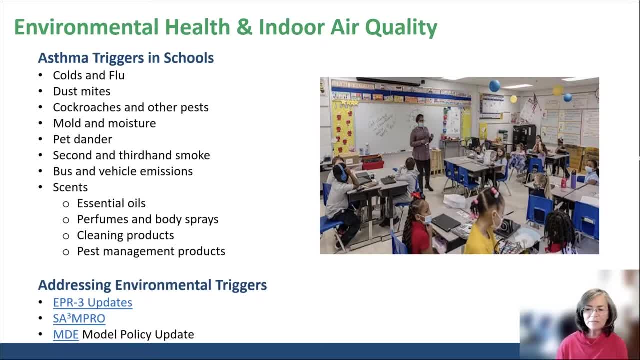 and vehicle emissions can become barriers for students with asthma to be healthy in school and ready to learn. The good news is that now more than ever, we have low or no cost solutions to address environmental asthma triggers in schools, such as outlined in the EPR-3 updates SAMPRO. 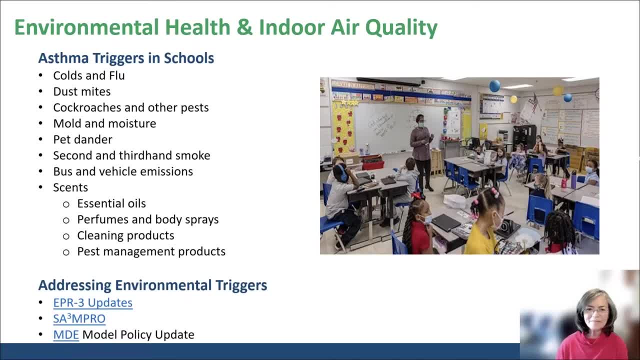 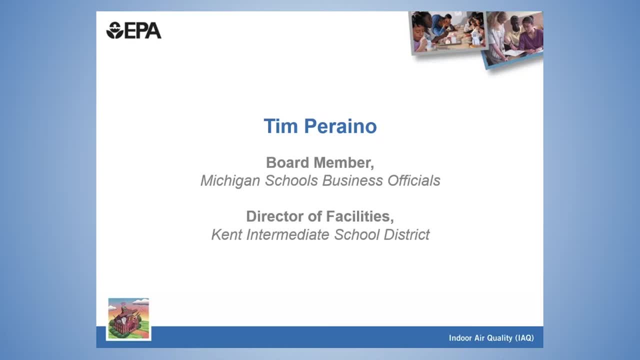 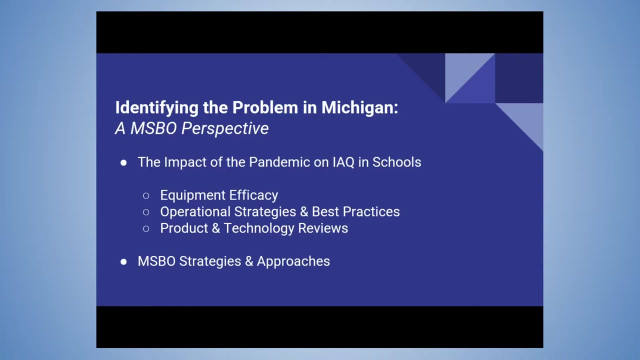 and our MDE model policy. Thank you All right. next up we have Tim Pereno, a board member of the Michigan School Business Officials, or MSBO, and the Director of Facilities for Kent Intermediate School District, Tim. Yes, good afternoon everyone. As was mentioned, I am Director of Facilities at 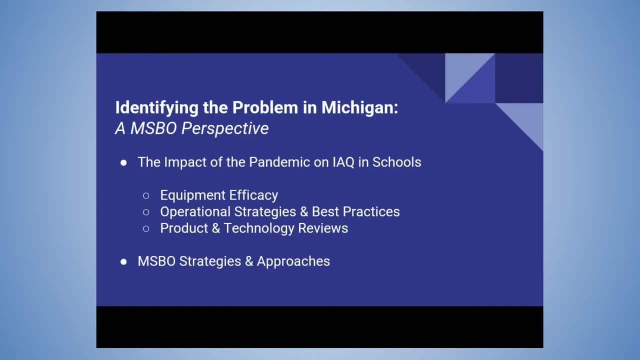 Kent Intermediate School District here in Grand Rapids. Kent ISD has been the fourth largest ISD in the state of Michigan. We serve over 100,000 students and I'm actively involved with districts all around the county, both public and private. 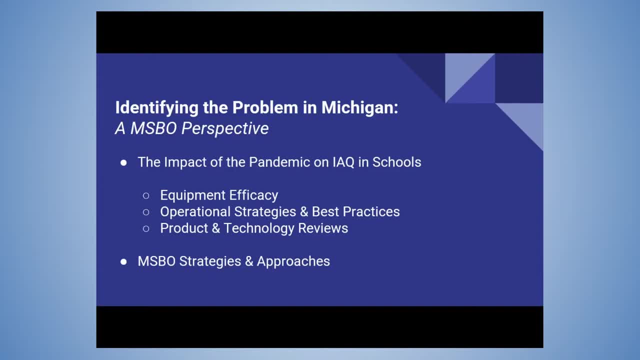 and have been dealing with indoor air quality issues with them for quite some time. Also, as a board member for the Michigan School Business Officials, or MSBO, I've been involved in school facility committees at a statewide level for over 25 years. 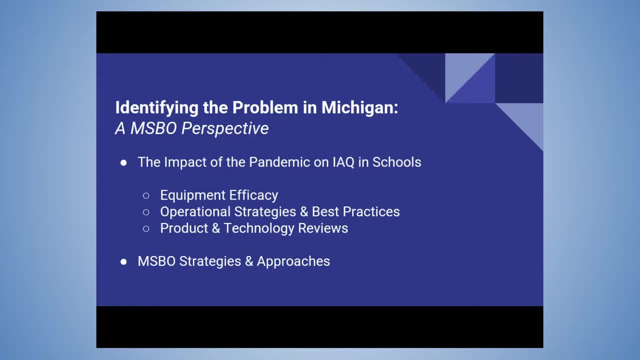 I've been a member of the Board of Directors for over 30 years and I've been involved in the public health department and the public health department and the public health department for over 30 years, So we've been very involved in this issue. I think it's important to note. 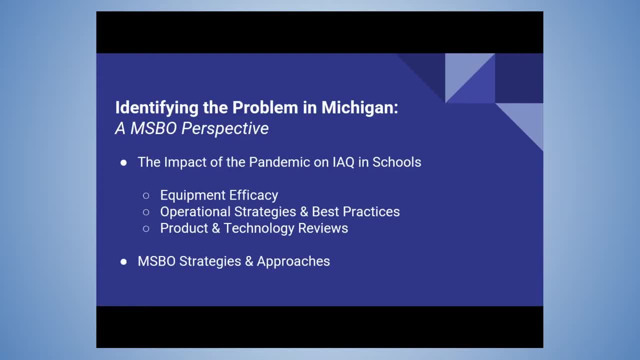 that indoor air quality has been an important issue for schools for quite some time. We've routinely monitored indoor spaces to ensure proper ventilation and address occupant concerns. In many cases, this involves verifying that the proper preventative maintenance has taken place on air handling equipment, that filters were replaced in a regular schedule and that contaminants did not exist within the space. 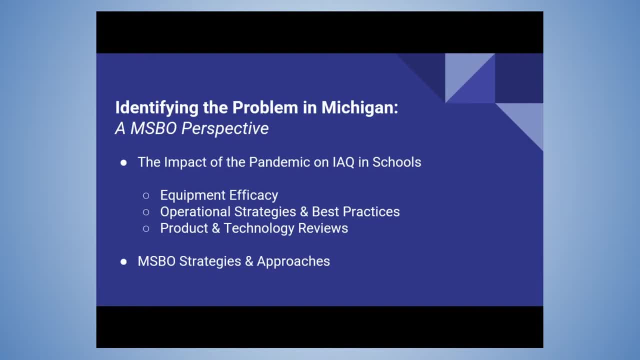 of products that contain high levels of volatile organic compounds, or VOCs, and an emphasis on cleaning and sanitation were all commonplace and continue to be so. It was with the onset of the COVID pandemic, however, that the importance of IAQ and the proper functioning of heating, ventilation and air conditioning equipment has been elevated. 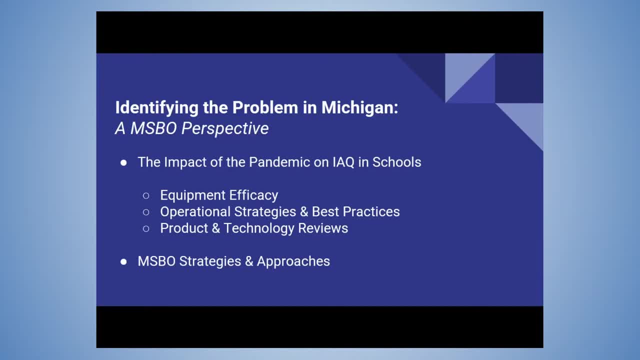 to a much higher level of concern. As more and more evidence pointed to the airborne nature of the virus, school districts throughout the state shifted their operating protocols and focused their attention on how to best mitigate the transmission of the virus. MSBO began offering virtual town hall meetings shortly after the onset of the pandemic. when 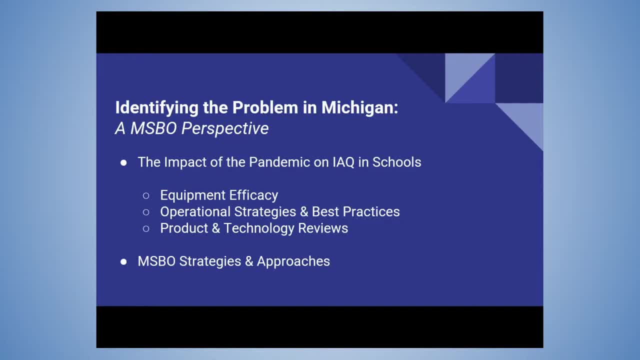 schools were shut down and have continued holding these town halls up to this day. The discussion topics in these meetings were varied- at the beginning of the pandemic, for sure, and dealt with things like cleaning and information that we really didn't know good details on. But over the course of the pandemic we've been able to get a lot of information from. 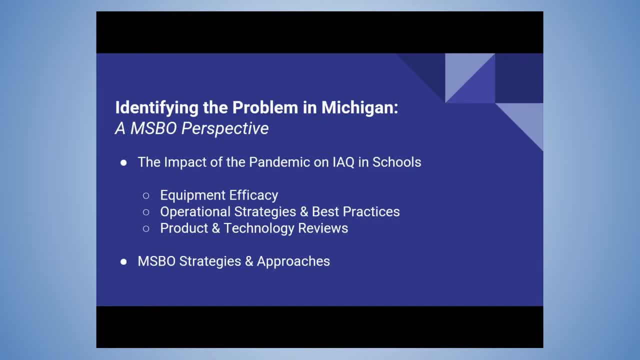 the public. Last 18 months to two years have been much more focused on IAQ issues and strategies that schools can implement to protect students and staff. School personnel, especially those in facilities and operations, have been inundated with recommendations about operational protocols, new technologies, new products and enhanced monitoring services. 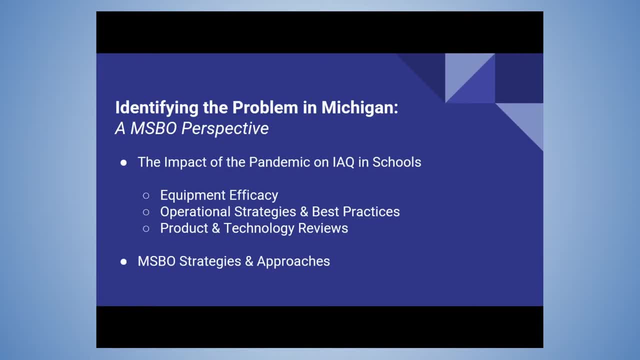 The struggle for these folks is to be able to evaluate the efficacy of these recommendations, make informed decisions that will not only positively impact the health of the students and staff in their district, but will be operationally and fiscally sustainable, and I think that is a very important message is that there is just 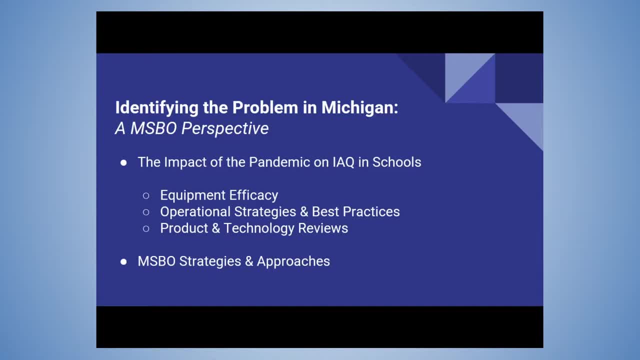 a lot of information for folks to take in and to understand what is viable and what is not. now more than ever, there's also an increased scrutiny from not just the staff and students within the buildings, but also from parents and community members, and so there is a greater emphasis on districts. 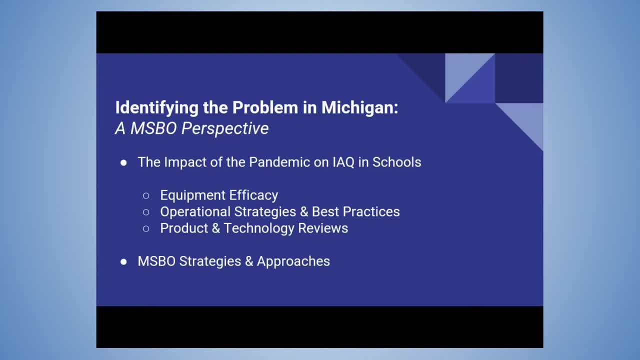 implementing best practices and operational strategies that improve indoor air quality and then reduce health risk to to all occupants. it is also important to note that most districts throughout the state are receiving these, you know, the emergency relief funds, as was mentioned earlier, and with the influx of this money it seems critical they understand how best. 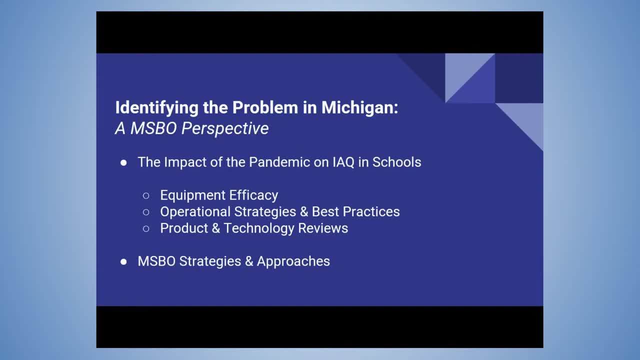 to utilize these funds to make the biggest impact on the health and safety of staff and students and on indoor air quality. they need to be informed consumers and it is imperative that in districts understand how new technologies work and how new products operate and which ones are best for them. 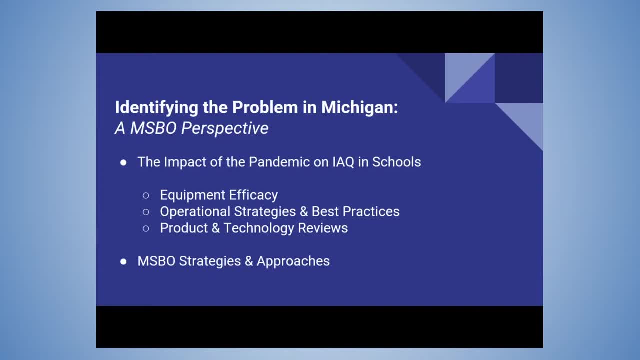 in their given situation. they need to understand how these new approaches will provide the biggest impact to their district. msbo, as an organization, really has taken the lead in providing training in the form of webinars, conference sessions and virtual town hall meetings, as i mentioned before. surrounding these issues, indoor air quality and 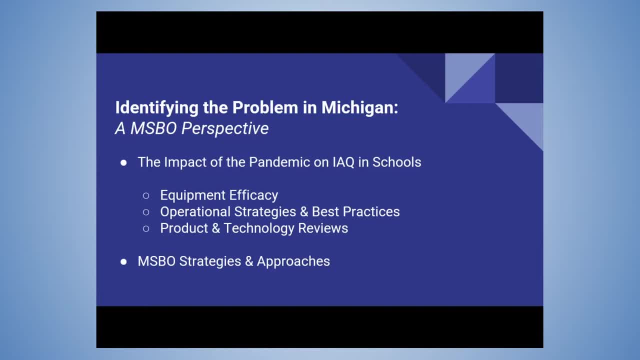 code response. planning sessions such as this one are especially critical for school personnel, who are attempting to stay up on the most current information, especially as they plan for future facility improvements, and that is happening quite frequently across the state, so i'm looking forward to information being shared in today's webinar because of its critical importance. msbo as an 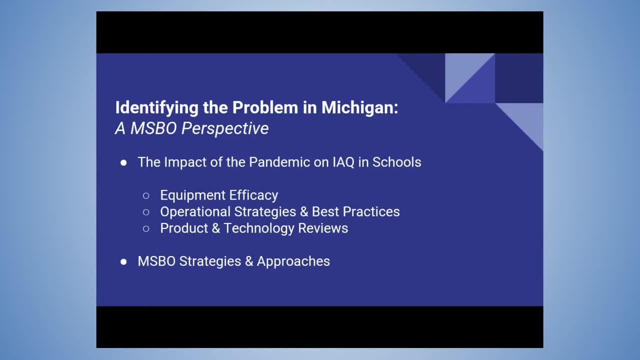 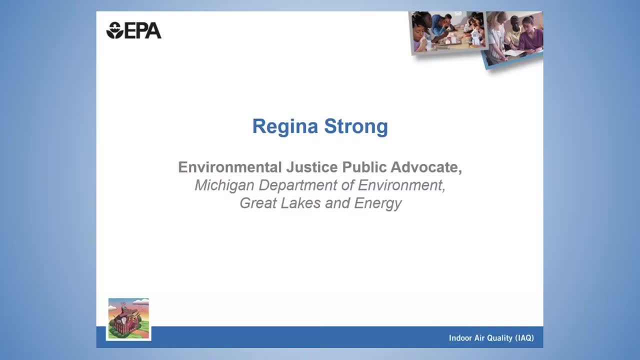 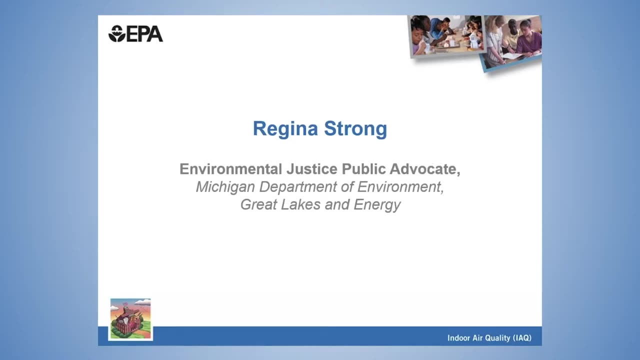 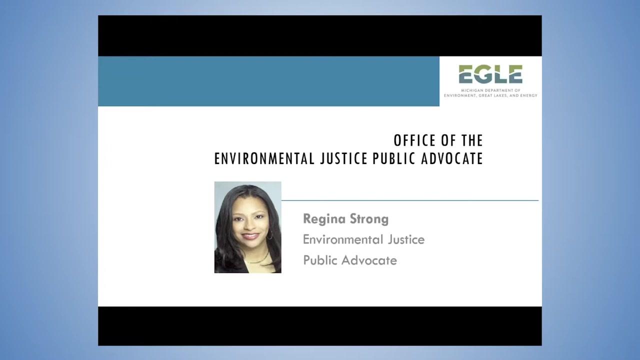 organization will continue to serve as a resource for these issues, so please look for opportunities and information coming out in the near future. thank you very much. all right. next up we have regina strong. she is the environmental justice public advocate for the michigan department of environment, great lakes and energy. hi, regina, take it away. good afternoon, good. 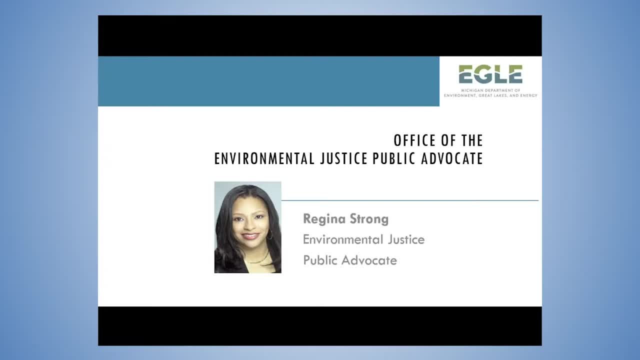 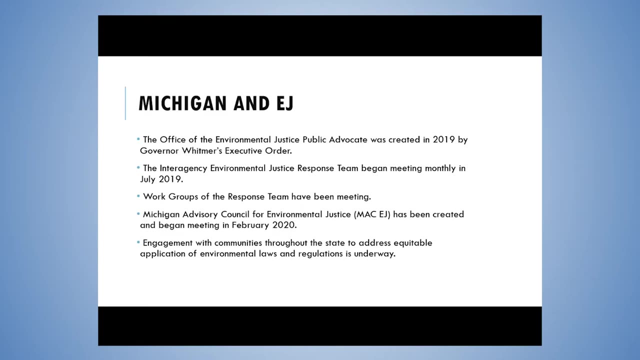 afternoon. thank you so much. um, i really wanted to share kind of the genesis of a michigan program that i'm hopeful many of you are familiar with already. so my office, the office of the environmental justice public advocate, was created in 2019 by governor whitmer to really focus on what many communities faced across the state. 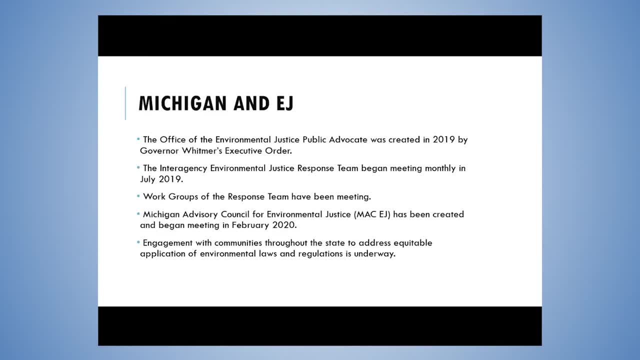 in addition, there was an interagency environmental justice team that was formed at the same time to really bring all state departments to the table to really have discussions about the ways to address environmental justice across the state. one of the uh areas of the work of the response team was to create work groups to really focus on different 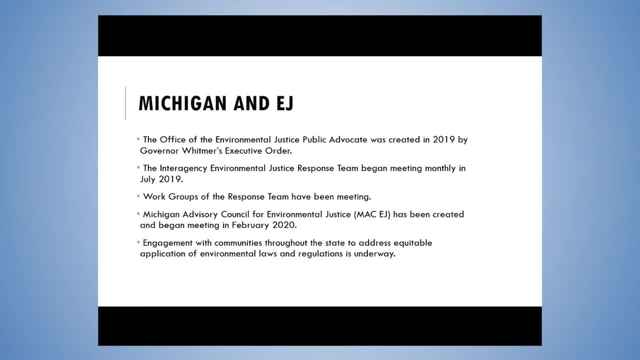 areas and ultimately, we also created, from our office, the michigan advisory council for environmental justice, or the mackie j, as i like to call it, um, which began meeting in february of 2020 and today has only had one in-person meeting, given um the covet reality that we live in right now, and so 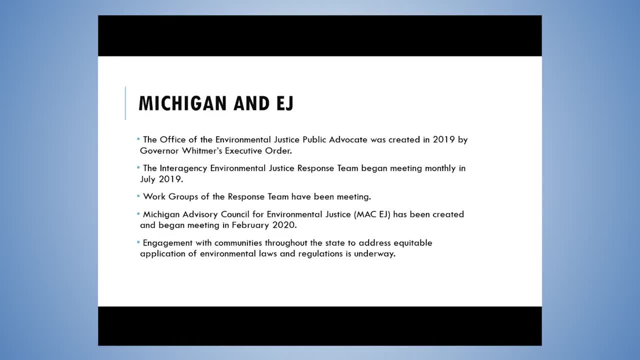 the goal of the office is really to engage with communities across the state and one of the things that um has been challenging for our communities- particularly those who you know live in areas with um potential impact from industrial sites and other things that impact their quality um was the concern about schools. 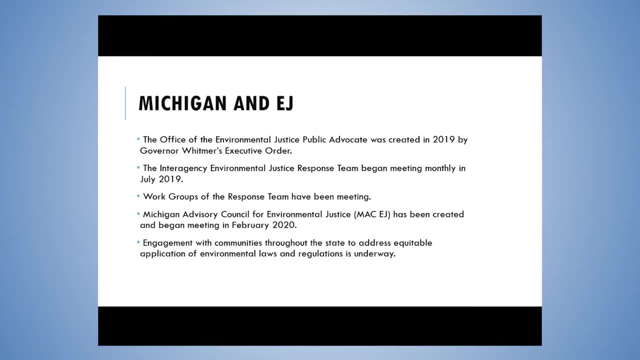 in close proximity um to those sites and so, pre um pandemic and pre our concerns around covet 19, there was really a desire to address that authority that i had been sketching a long time ago, getting good care of it and reducing pandfish and having an. 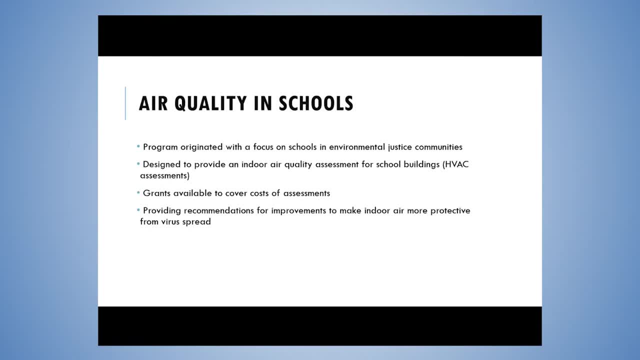 economy that had never approached, закры things that were designed to affect our public right and yet social, authentic and um, we just have to re-wyn that there's so many requirements, um, and i think obviously it depends on our community air quality in schools And you've heard, you know, from the two previous speakers about 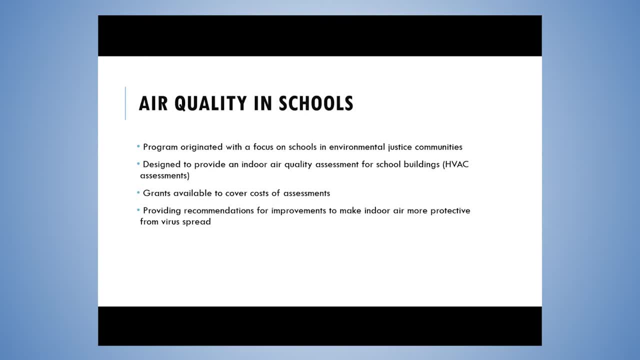 just concerns around asthma and other things that impact the respiratory health of students external to the school and internal to the school And so really thinking about how do we address that. So the initial genesis of looking at ways to support HVAC assessments in schools really came. 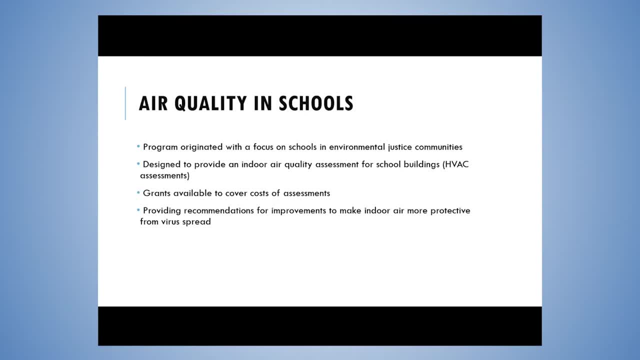 from that desire to address asthma and other issues that could impact schools in certain communities. Once the pandemic took hold, it was really evident that communities, in particular environmental justice communities, often lower income communities, were particularly hard hit by the pandemic in the early stages And our advisory council really wanted us to look at a way. 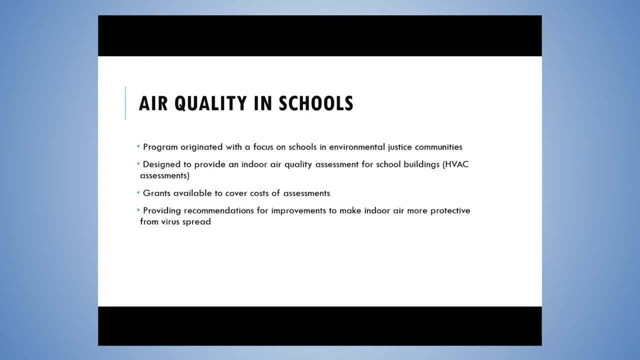 to address that. So the beginnings of the program to assess HVAC systems in schools was very focused on looking at that air quality in schools in EJ communities. However, as the pandemic continued, what we realized is that all schools across the state. 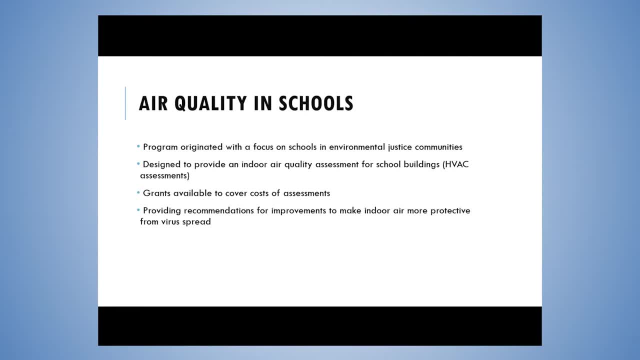 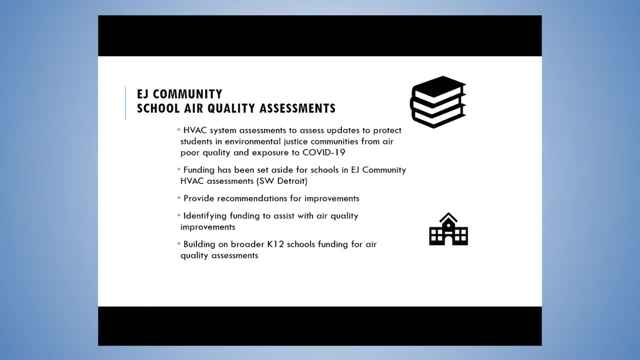 really needed the opportunity to assess their systems to see how they could be more protective. And so one of the things that you know we did early on in looking at those opportunities for air quality is worked with the energy office within EGLE to see if there was funding to support that effort. So you all may have seen if 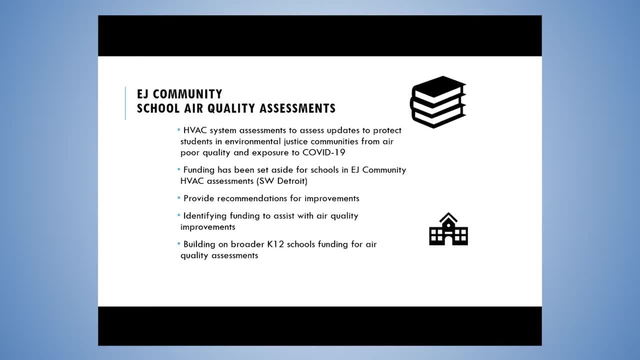 you work with schools in the state. a call for survey, information and opportunities to apply pretty much last year was when that came out in 2021. That program continues, although the survey has not The need for the survey. really, it is an application now. 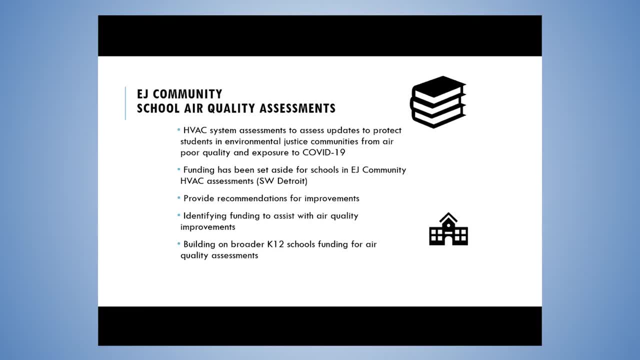 And the good news is we have funding to support these assessments in any school across the state, So every school is eligible, And we really want to help use this as the starting place of moving forward with addressing indoor air quality in schools, And so this remains available to all. 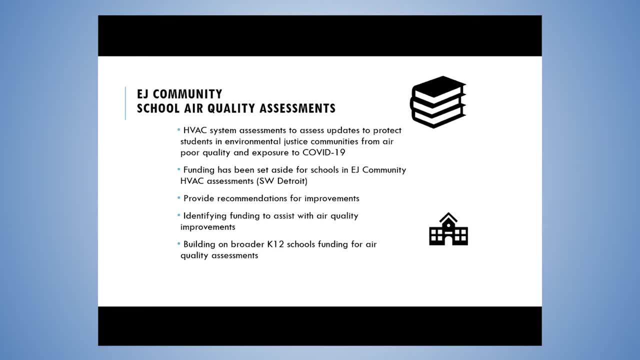 school districts across the state. One of the things that I think is critical to that, and both a challenge and, I guess, an opportunity moving forward, is in this work we're going to have to work. There is a challenge of finding contractors, not just for this work but for other work. 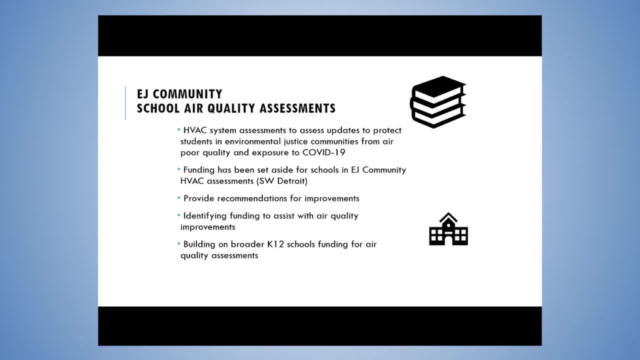 And so it has been slower than we anticipated. but there are still opportunities to have systems assessed. So I want to assure you that if your school district applies to have buildings assessed, we will definitely get you in the queue and support the cost of having that assessment done. 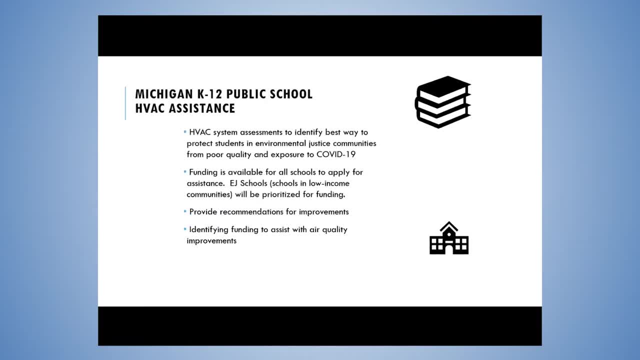 And so, really, you know, this slide just echoes what I just said. Funding is a challenge, but it is a challenge to find contractors, not just for this work but for other work. If they're not working, we're going to be able to get them in areas where they actually have this. 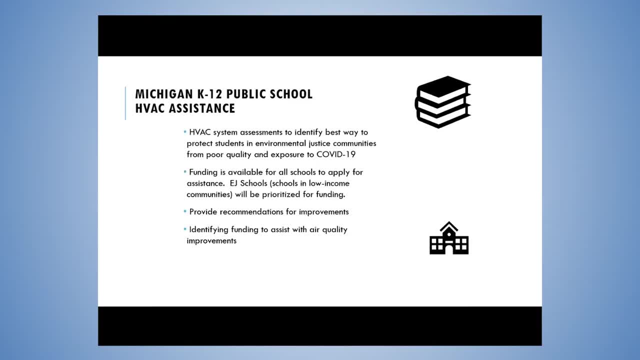 building, And so that's a challenge, but it is a challenge, So I wish you all the best in the work that we're doing. So we're going to have a couple more minutes. I'm going to ask you to put your hand up on the screen and we'll get you to take it off the screen. 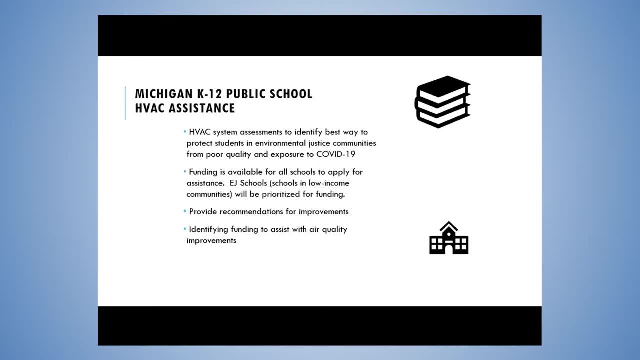 But I want to make sure that your voice is heard and you know that this program is available, Also looking at through the assessment how to make recommendations for improvements, so that then you can take that to the next level and use that assessment in concert with what the EPA IAQ office can. 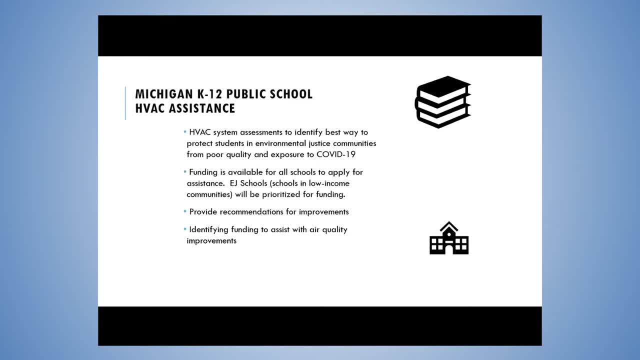 do, and other folks in the state. So just wanted to make sure I share that I will be around during the question genesis of the program and that that program can be a first step in assessing what comes next in your work for improving your quality within your school. thank you, 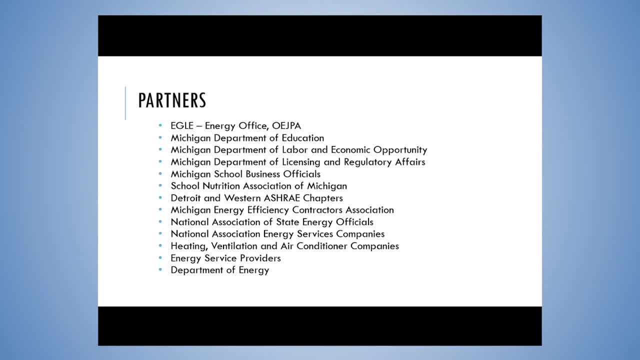 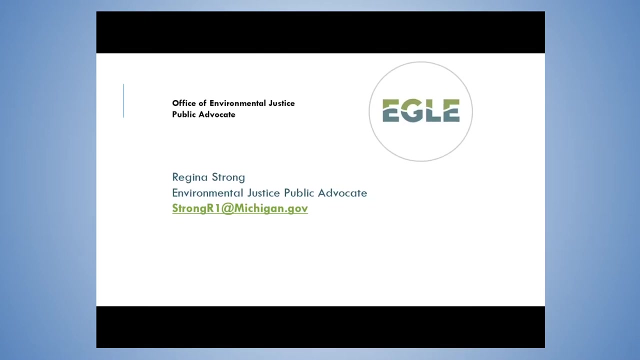 oh, just wanted to mention this has been a partnership across many departments in the state, as i talked about, as well as external partners, to really, um, you know, move this forward, support, um the cost of an assessment and take things to the next level in terms of your quality for students. now i'm done. thank you so much. thank you, regina. thank you. 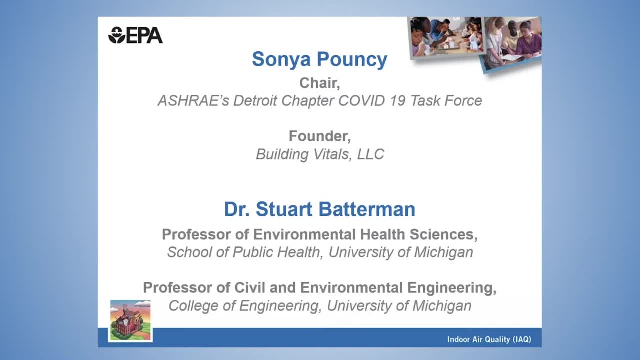 all right. and next up we have sonia ponce. she is the chair of the ashrae detroit chapter covid19 task force and founder of building vitals, as well as dr stewart batterman, a professor of environmental health sciences at the university of michigan. 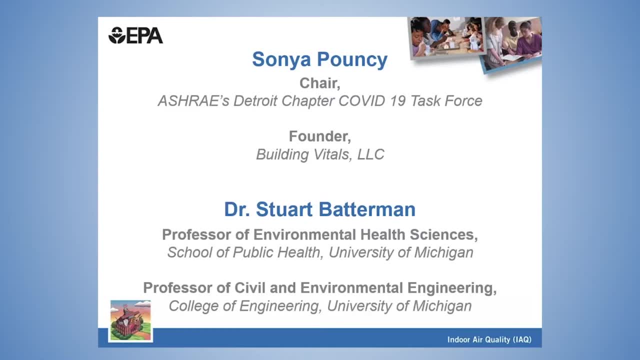 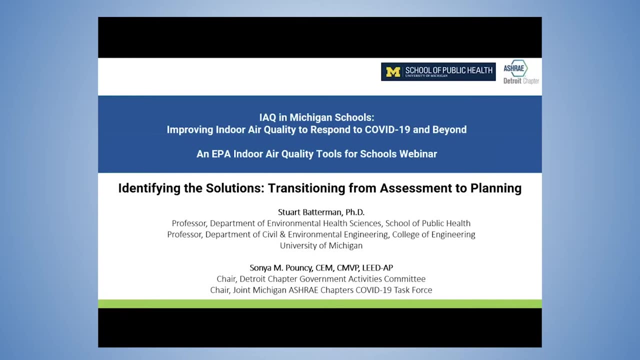 i'm also a professor of civil environmental engineering at the university of michigan. go ahead, okay. i'm going to start off and i hope you can hear me. so this afternoon, sonia and i are going to give you a fire hose here of information, just a lot of information dealing with transitioning from assessment to planning, actually improving. 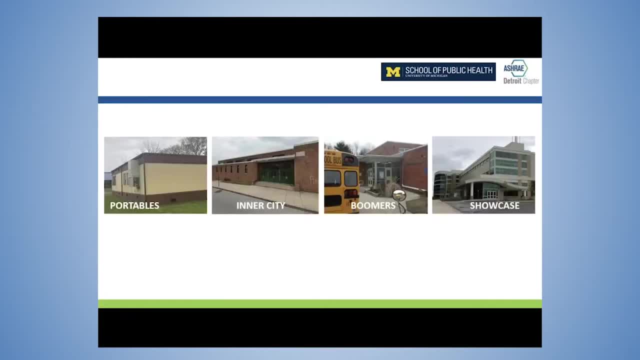 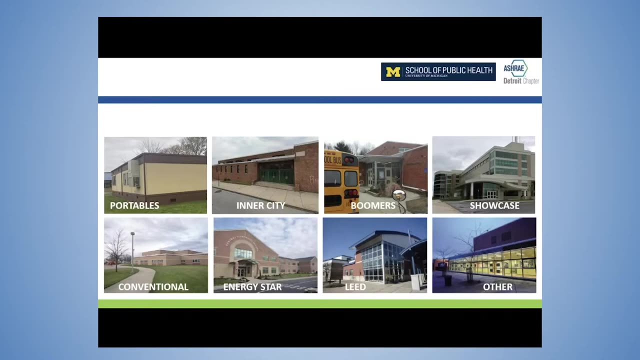 education and learning. again this afternoon, ordinatemacons for students face a new challenge in aviation, world aviation, and it's what we're looking to accomplish, and i'd like to begin by saying that you know, in our state we have to take the opportunity to really think about. what is really important is the quality of our Taste and the quality of 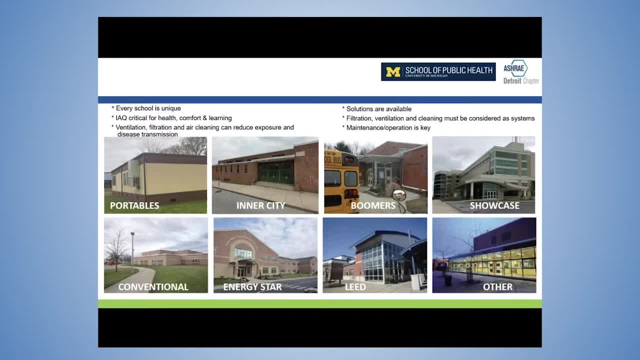 our air quality is really important and i think that's a very important piece. um, we have to try to bring in all of these factors, but i want to talk about a couple of my objectives. first, there's the school's indoor air quality is critical for health, comfort, learning, for minimizing the COVID. 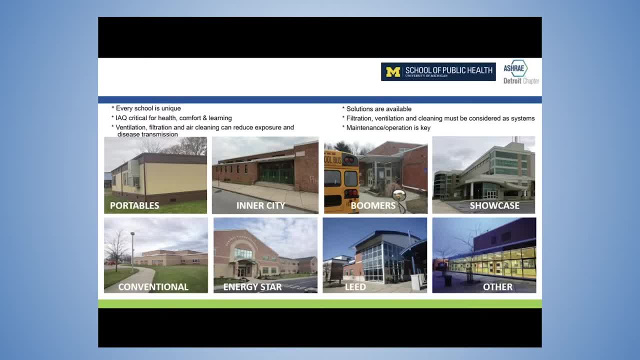 risk. The ventilation filtration, air cleaning systems can reduce exposure and disease transmission, regardless of the type of school. there are solutions that are available, but you just can't dump them in. they have to be considered as part of a building system. and then, finally, maintenance and operation, as we'll talk later in the presentation, are 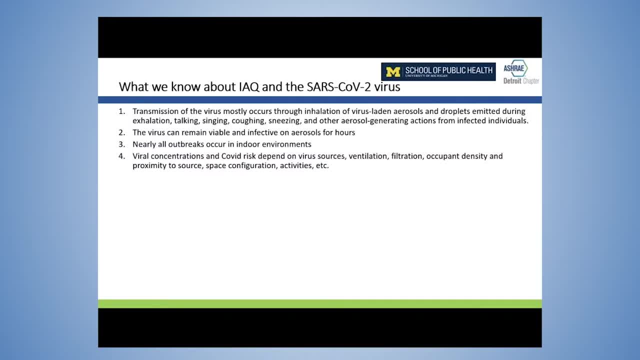 very key components. So what do we know about indoor air quality in the SARS-CoV-2 virus? First of all, it's clear now: the transmission of the virus mostly occurs through inhalation of virus-laden aerosols. Aerosols, I'll discuss, are smaller droplets or smaller particles. 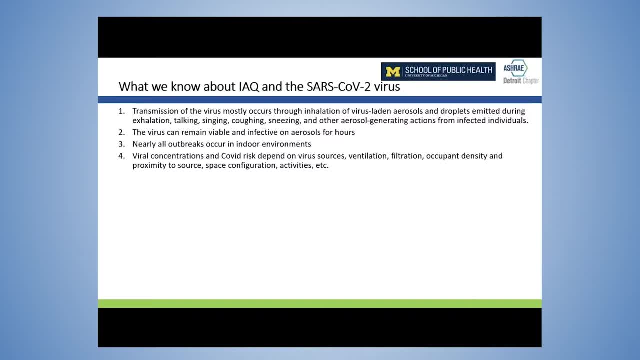 that are emitted while talking, exhaling, singing, sneezing, coughing and so forth. Once airborne, the virus can remain infective and viable for hours. A review of about 300 or 400 outbreaks showed that every one, or nearly every one, occurred in indoor environments. so the indoor environment 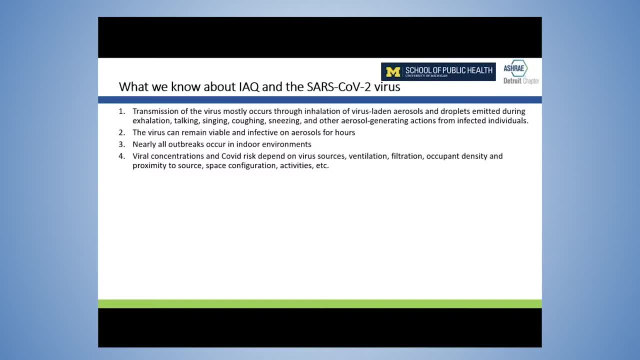 is the key place where this occurs and the risk, the viral concentration, the viral load and uptake depends on many factors that are listed in the slide, but it's clear that ventilation, filtration and air cleaning can improve things. So what's the situation in schools? in Michigan schools and 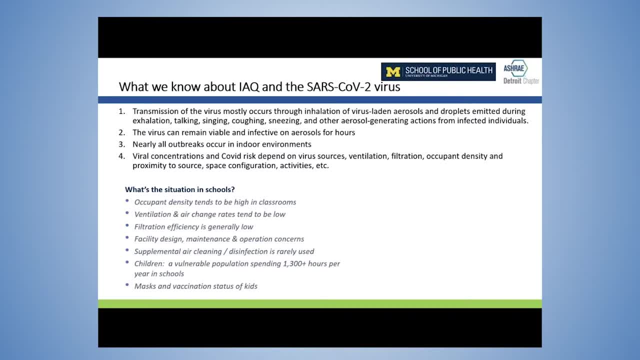 other schools Quickly. we have high occupant densities. we have issues with ventilation, and air change rates tend to be low. filtration efficiency is generally pretty minimal. there are significant concerns regarding the design, the maintenance and the operation of mechanical systems. rarely do we see supplemental air cleaning use. 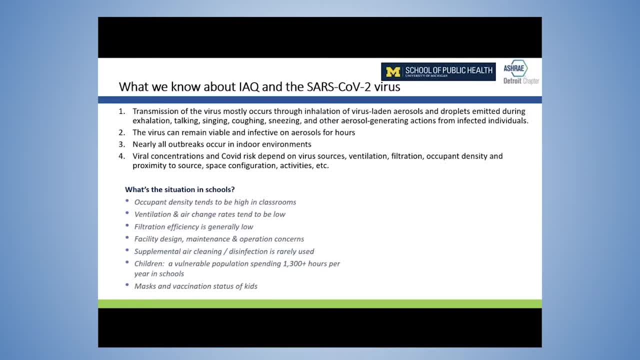 And children are a vulnerable population and they spend 1,300 or so hours per year in schools. It's the most important environment after the home for them. And of course, it's tough to get kids vaccinated and to ensure that masks are worn. So taking all these things together, next slide. 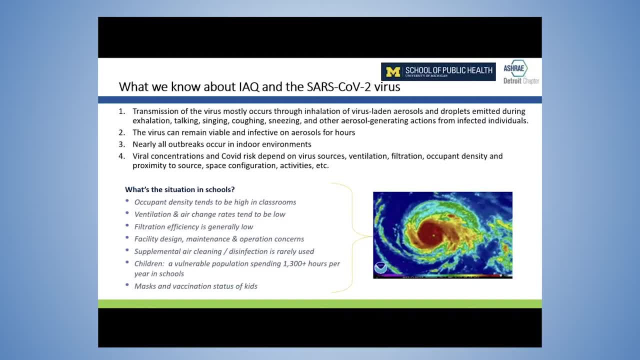 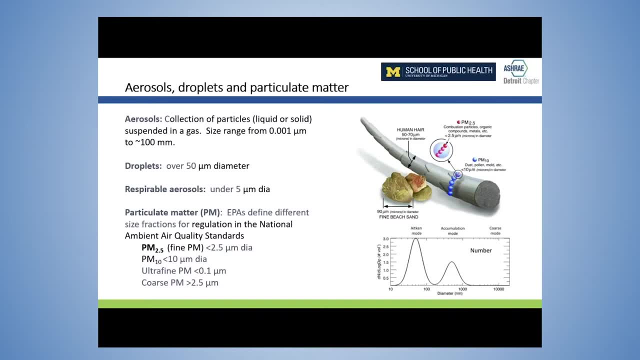 we have the perfect storm. All right, let's move on Now. I don't want to spend too much time because our time is limited here, but this picture on the right shows human hair. The little blue dots are called PM10.. These are 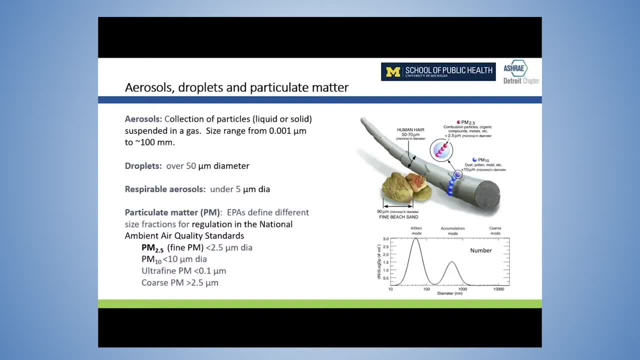 10 microns in diameter. The little pink dots on the blue are called PM2.5.. This is particulate matter under 2.5 microns, something regulated by US EPA in outdoor air. just to give you a sense of the microscopic nature of these PM2.5 particles. For COVID, what we're most concerned, 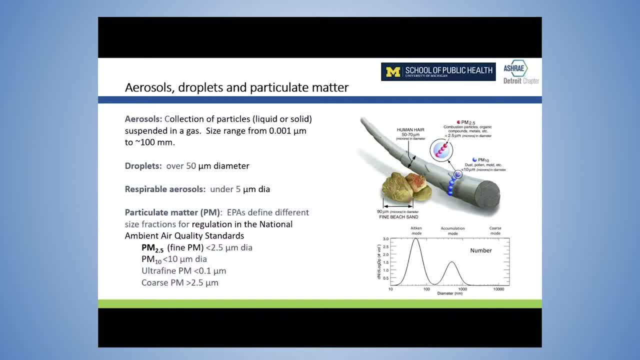 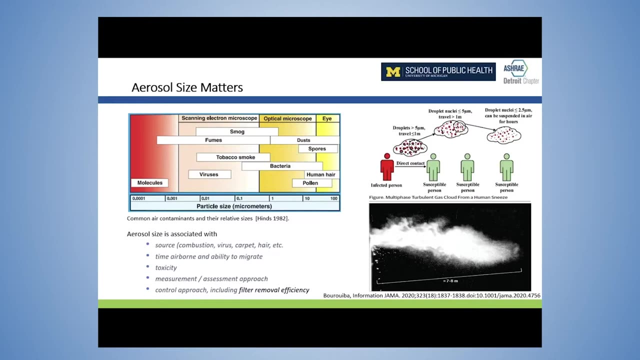 with are respirable aerosols. These are typically under 5 microns, so they're kind of a little bigger than the PM2.5. But these can all be important and you should recognize that the size of these aerosols varies considerably. So the size matters. It matters because it. 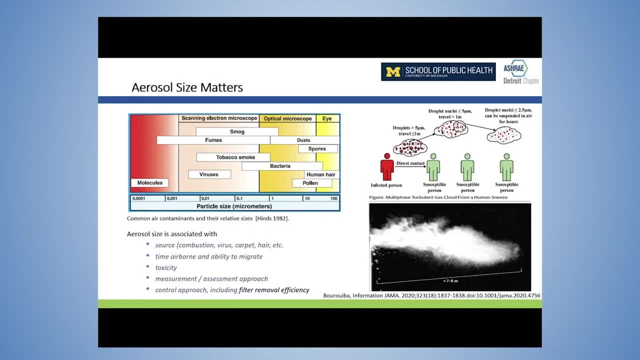 primarily affects the longevity of the aerosol in the air. Aerosols just a few microns or smaller will essentially stay airborne until they're removed by a filter or deposited somewhere. They won't fall out of the ground. On the other hand, larger aerosols, called droplets, typically over 50 microns in diameter. 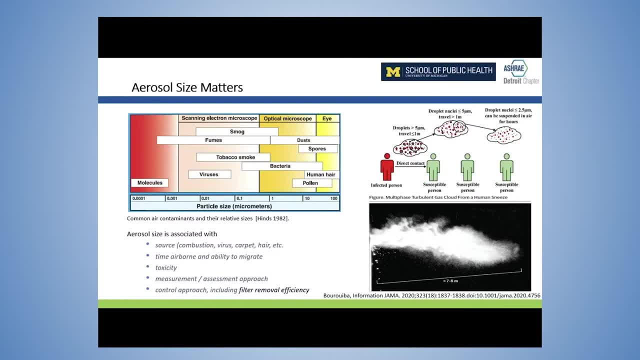 will fall out within just a meter or so. So the picture at the right shows the infected individual in red. They might sneeze. They're a micrograph. The picture in black and white to the bottom shows a sneeze where the larger particles are dropping out of the air and with a 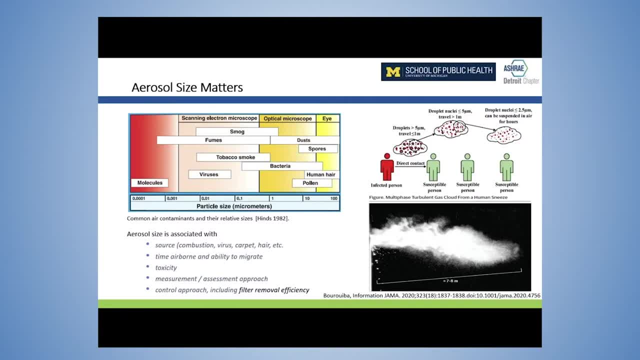 smaller amount of air. So these are the kinds of aerosols that can fall out within just a few feet, while the smaller aerosols, the respirable ones, just a couple microns in diameter, can drift seven, eight meters or longer and stay airborne. And so what we can do is to understand. 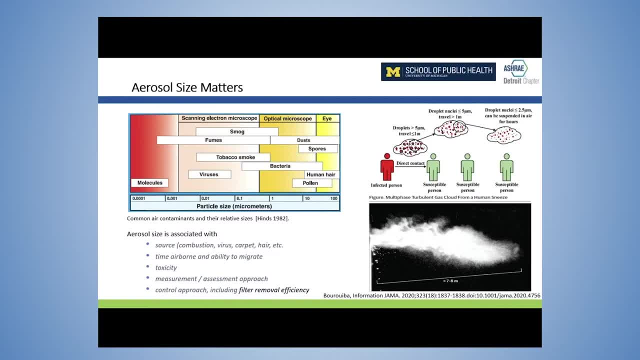 the importance of the aerosol size in aerosol transmission and the COVID risk. Also, aerosol size really matters because the ability of a filter to remove the particle is a very strong function of aerosol size and only the better filters will get these smaller. 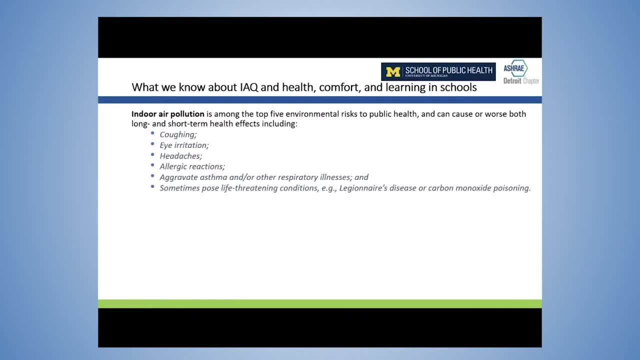 particles. So we had some overviews of the importance of indoor air quality on health, comfort and learning in schools And I don't want to repeat what was gone, what was transpired earlier in the webinar, but we know that indoor air quality is among the top environmental risks. 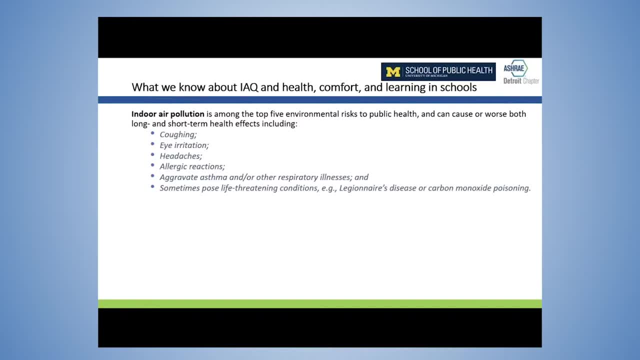 of public health and it has both short and long-term effects, including asthma, as was mentioned earlier, And these problems can affect learning and comfort and performance in schools, And in the last five or so years there have been a number of very interesting and informative. 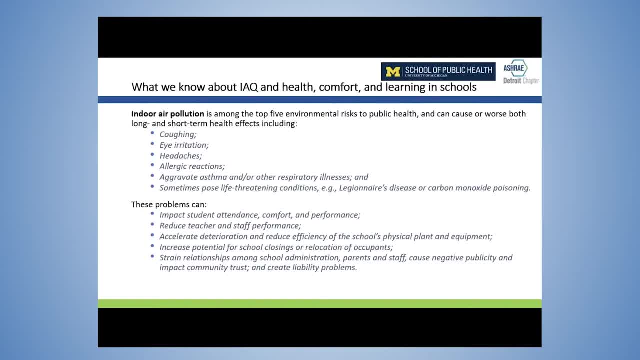 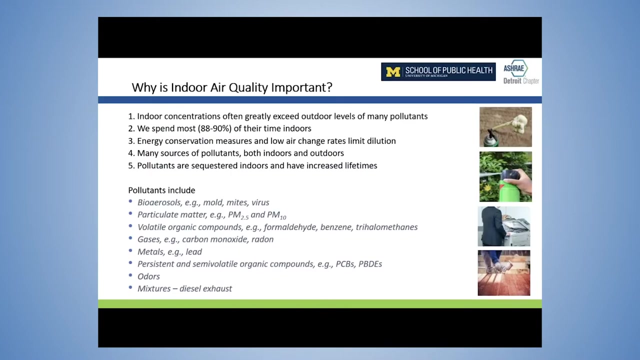 studies showing how both student and teacher performance deteriorates when comfort and air quality is not optimal in schools. So EPA likes to stress how important the indoor environment is with regard to safety and stewardship for students and staff, and also for facilities. So it's been interesting for me. 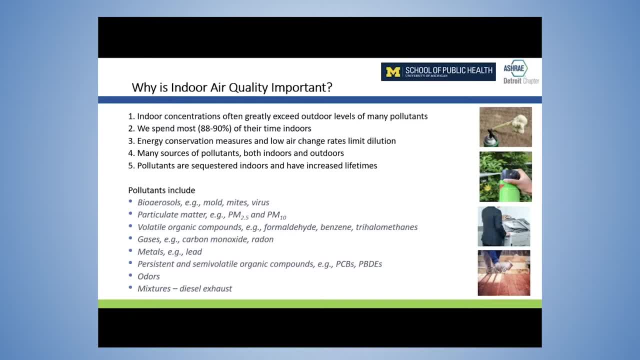 working for a number of decades in air quality, and perhaps about 20 years ago we started recognizing that indoor air quality is really very important- potentially more important than outdoor air- for a number of years, And that's really because of a number of good reasons. First, we spend most of our time indoors. 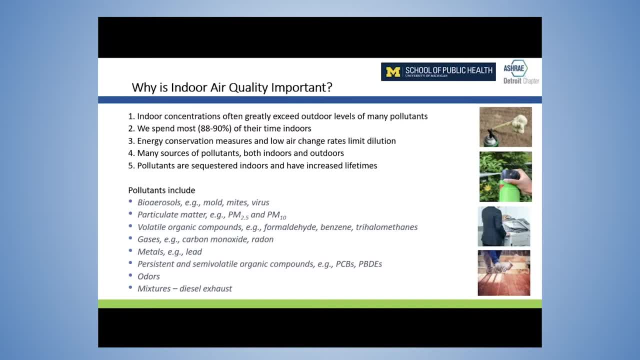 Indoor air concentrations are often higher than outdoor levels. Things have not gotten better with energy conservation measures, necessarily, which limit dilution, And there are many sources of pollutants both indoors and outdoors, And finally indoors. we actually can sequester some of these. 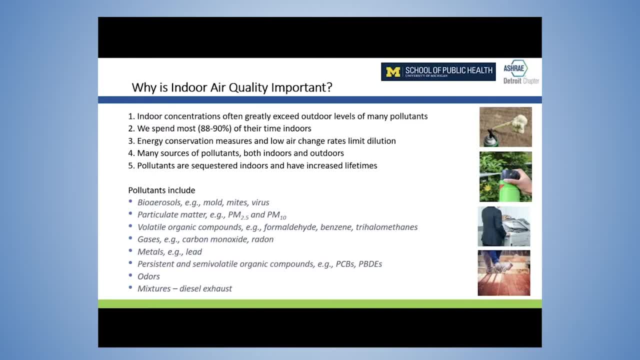 pollutants and increase their lifetime, and this can lead to higher concentrations and exposure. So there are a variety of indoor air pollutants of concern. Earlier we talked about asthma and largely particulate matters associated with asthma exacerbations And, of course, aerosols. 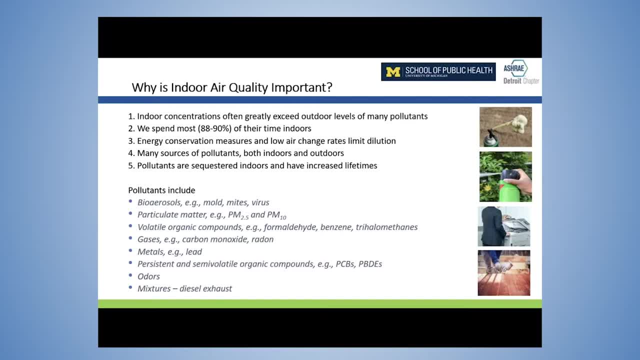 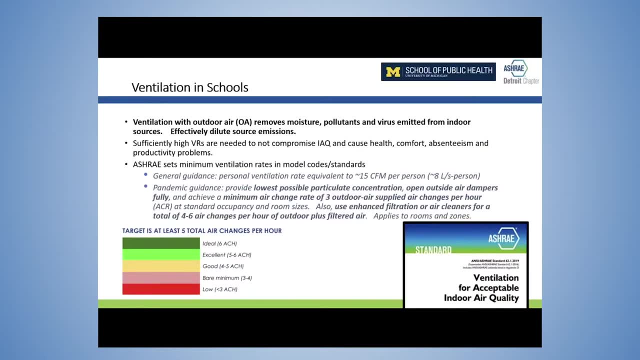 are a form of particulate matter and can transfer the COVID virus. So let's talk about some of the solutions. First, ventilation: Broadly ventilation with outdoor air removes moisture, pollutants and the virus that are emitted from indoor sources. Essentially, we're diluting emissions from a super spreader or somebody who 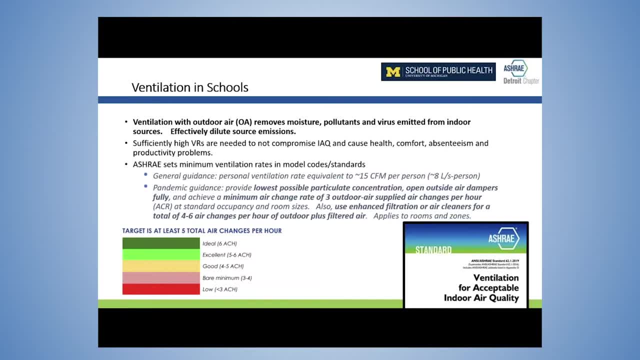 is emitting COVID. We need high enough ventilation rates so that we do not compromise indoor air quality and cause odors and discomfort and absenteeism and so forth. Now ASHRAE, the code setting organization, sets minimum ventilation rates in model codes and standards, which a new 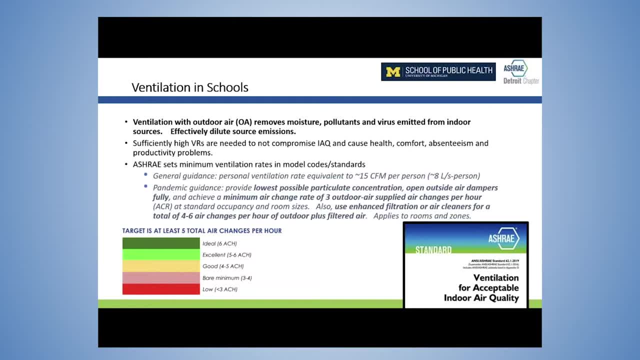 building needs to comply with. The goal is that personal ventilation rates should be at a minimum, something on the order of about 15 cubic feet per minute per person In the pandemic. ASHRAE came out with additional guidance, as did other organizations. The guidance is to provide the lowest possible particulate. 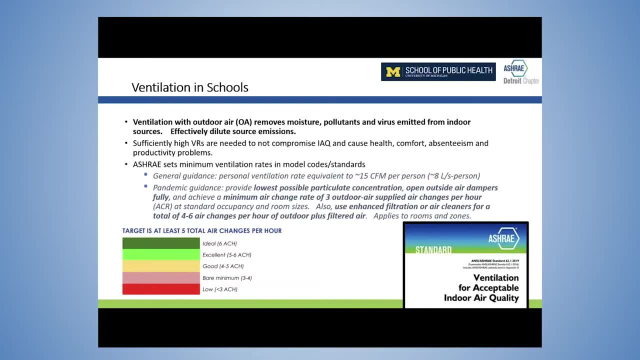 concentrations to fully open outside air dampers and to achieve a minimum air change rate of three air changes of outside air per hour. On top of this, used enhanced filtration or air cleaners to basically double the air change rate effectively to get a total of four to six air changes per hour of outdoor plus filtered air. 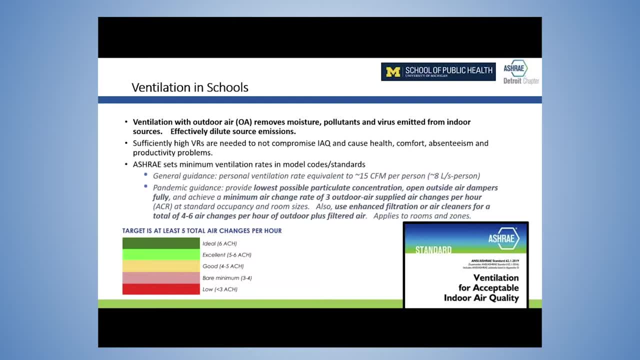 Now this applies to each classroom or other zone in the space. So the color graphic on the bottom left shows a kind of color scale where we want at least four or five air changes per hour. Ideally we'd like ten, And ASHRAE's standard is 62.1, shown at the bottom right. 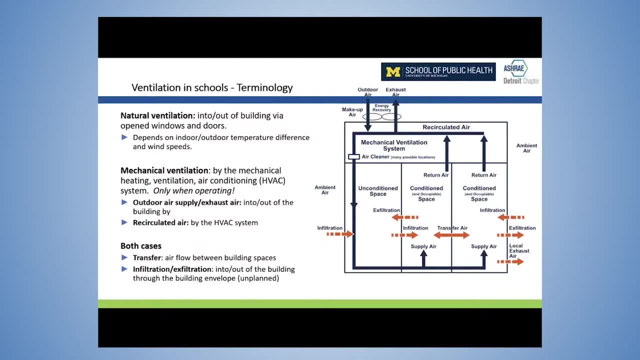 So just to make sure everybody's on the same page with respect to terminology for ventilation, I have here a schematic of a space showing you the major air flows. What we're talking about with natural ventilation is opening windows and so forth to allow flows. 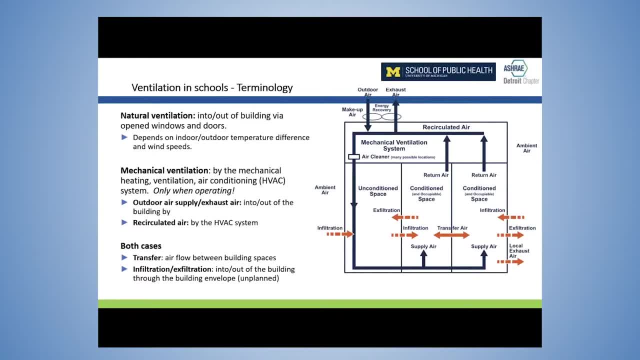 We also have infiltration- exfiltration through cracks and crevices in the building. What's not well recognized is that simply opening a window on a day like today, where it's very comfortable outside, doesn't really provide a lot of additional ventilation, because natural ventilation depends on the temperature difference and the wind speed. 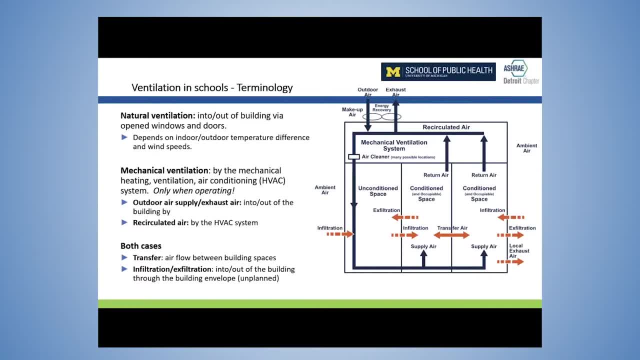 and you need large temperature difference and a wind speed to actually drive that air. Most of our schools and most of our larger buildings are mechanically ventilated. They have a heating, ventilation and air conditioning system. This provides that outside air is not as 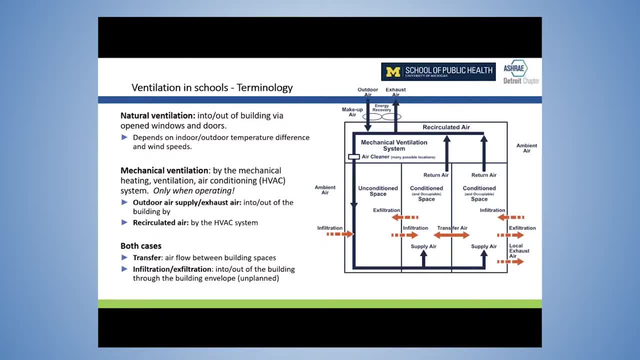 hot as outside air and the flows are shown on the diagram, And most systems recirculate air so that they don't have to heat and cool as much air, providing mixing in the space but not a new supply of outside air if the dampers are closed. 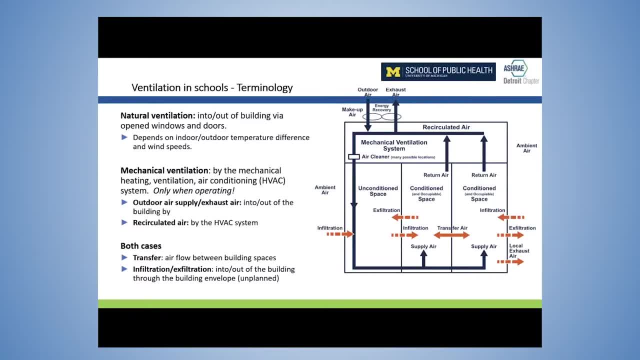 In both cases we provide ventilation through transfer between building spaces and infiltration: exfiltration, as I mentioned. Now, the guidance that I just provided from ASHRAE and others suggests that in the space we want to have three to six air changes per hour. 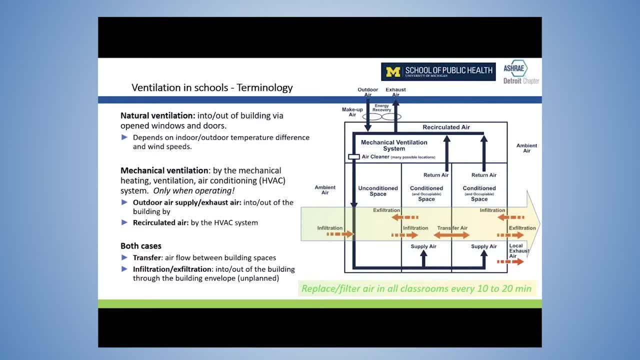 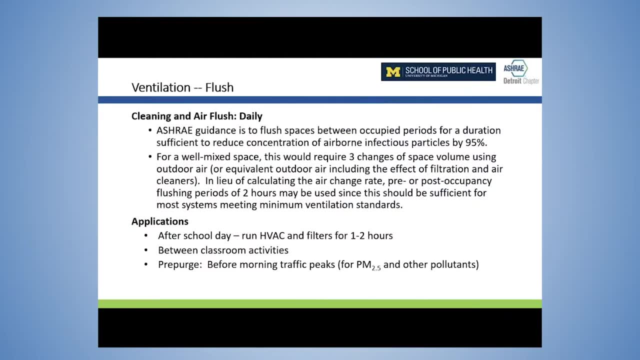 This means that in each classroom or each zone, you're essentially going to replace or filter all that air every 10 or 20 minutes. There's additional ways to use ventilation to improve the air quality, reduce COVID and so forth. There are flushing procedures where the space can be. 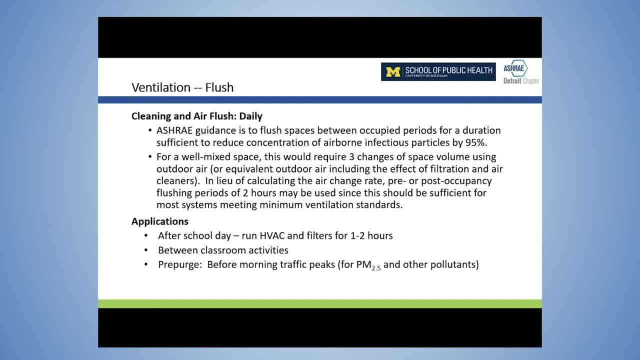 unoccupied and the space is flushed by changing the air quite rapidly. I don't see a lot of schools do this, but there are a number of good applications, both after the school day, between classroom activities and as a pre-purge in particular. 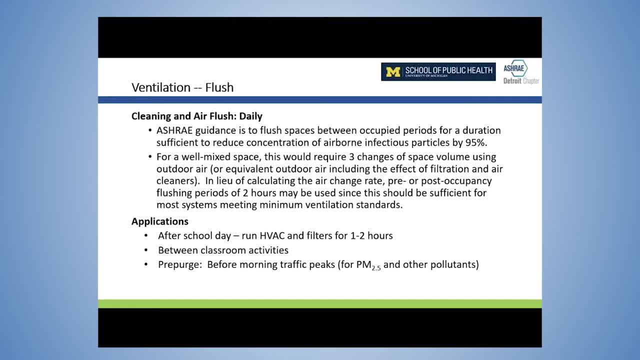 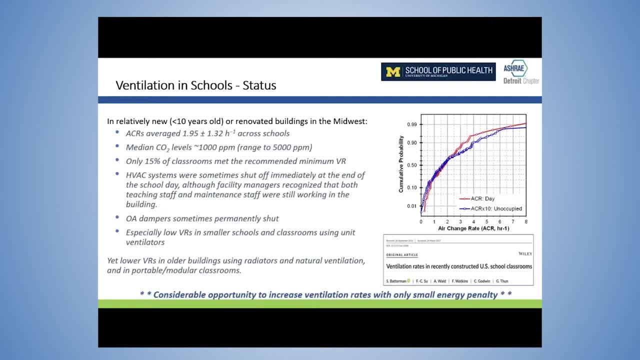 before morning traffic peak which might bring in pollutants. You can pre-purge before that and condition the space. So what's the status of ventilation rates in schools in Michigan and the Midwest? We did a study, looked at about 40 different schools, a bunch of classrooms in each one. 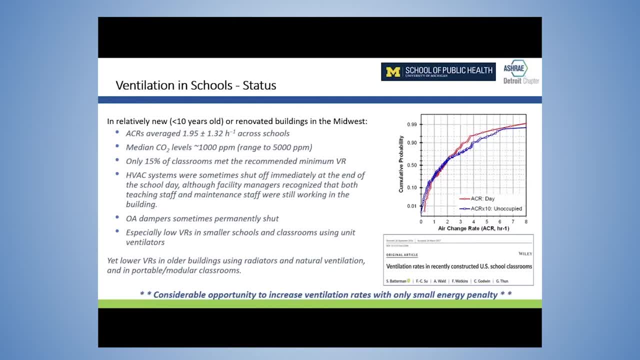 The condition that we found was not great. This was done prior to COVID, about five years ago, but in new schools less than 10 years old, or newly renovated, fully renovated schools, the air change rates averaged just under two air changes per hour. We want three. 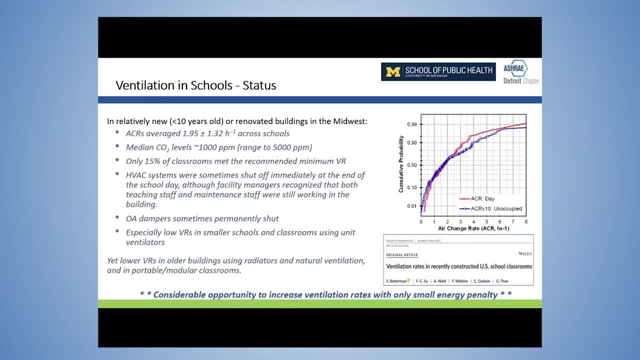 Only 15% made it to three. You can use CO2 as an indicator, Easy to measure, of ventilation rates. We have several papers that describe how to do that effectively. On top of this, we found that HVAC systems, mechanical systems, were often shut off at the end of the school day. 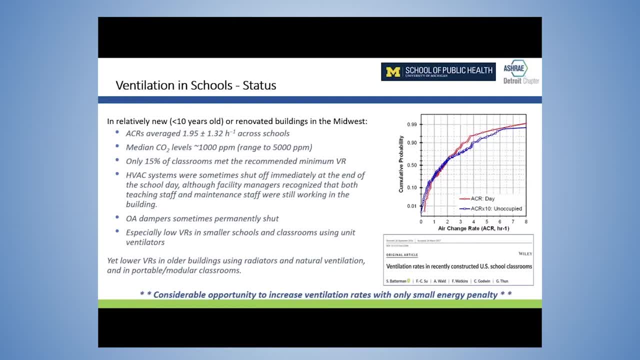 even though cleaning and other activities were still going on and folks were still working and sometimes kids were still present. We found a number of schools where the outside air dampeners were permanently shut. We found particular problems in smaller schools and classrooms where they were used as COVID ventilators. 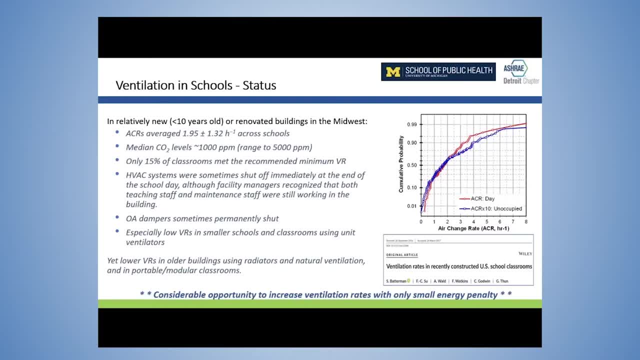 We found a number of schools where the outside air dampeners. We found particular problems. We found particular problems, problems in smaller schools. We found particular problems in smaller schools and classrooms using unit ventilators and some simpler non-centralized mechanical systems. This was the status in newer buildings. When we're looking at older buildings, 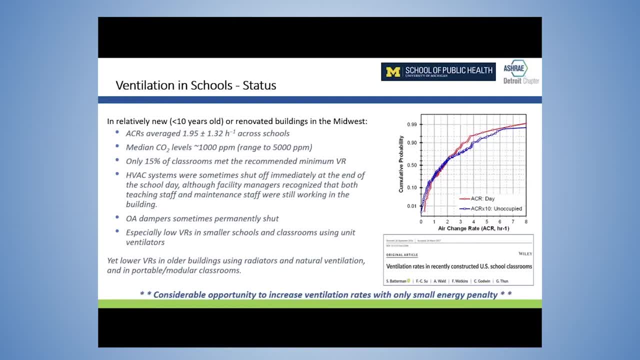 you know, 20 to 50 to 60 years old. we find much lower ventilation rates, particularly in those schools using radiators and natural ventilation, and we often find problems in portables and modular classrooms. The only thing unique- probably in Michigan, I would say- is that 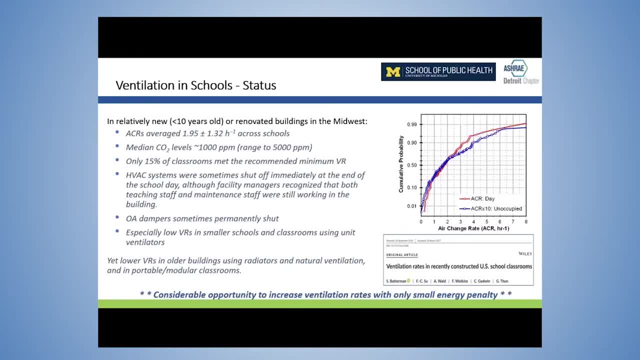 we have a lot of older schools and we have both a significant heating and cooling cycle, so we're using a lot of mechanical systems typically, or heating and cooling quite frequently. There's considerable opportunity to increase ventilation rates with only small energy penalties. My last topic, before I turn it over to Sony, is talk about filters. 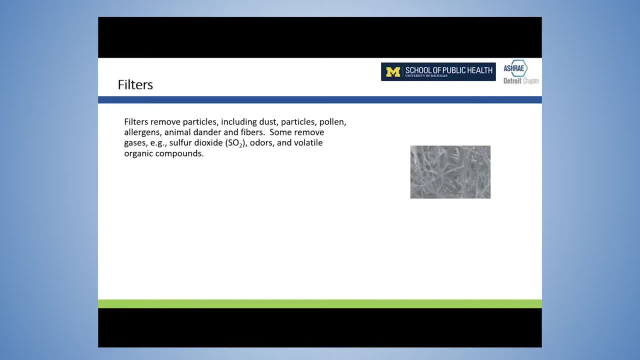 On the right we see a typical sort of fibrous filter. These can remove dust particles, pollen virus and so forth. So a mechanical system, as I'm showing here, has opportunities to have filters in several places. You can have outside air filters in treating simply the outside. 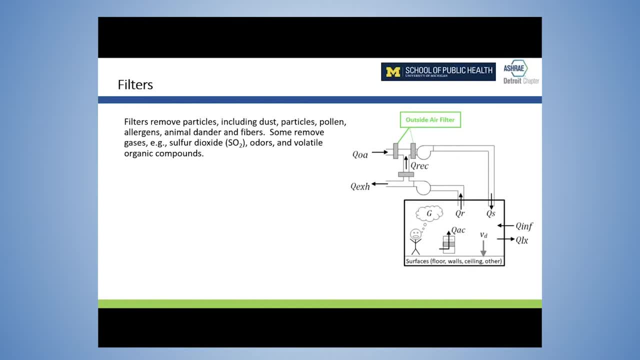 air or the combination of outside air plus return air- Next slide. We also have a mixing box, typically doing recirculation. You can have a filter there, Next slide And then finally adding a personal or a portable air cleaner or a room air. 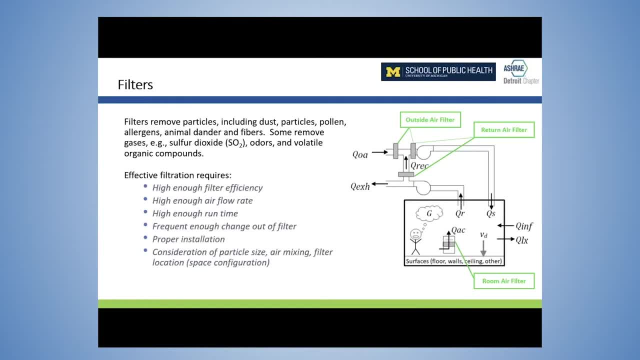 filter can condition the air in that space. To have effective filtration you have to consider this as a system. You need a good enough filter with a high enough filter efficiency for those small particles. You need a high enough flow rate. You have to operate the system. 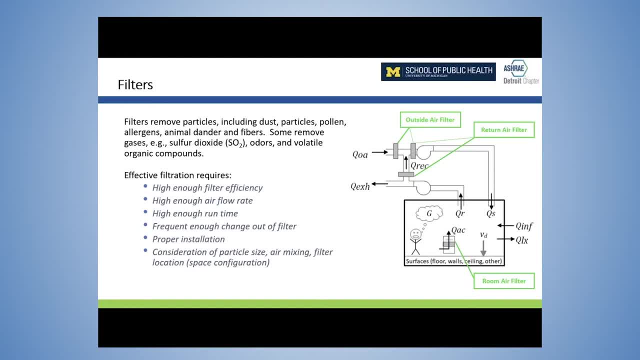 so you need enough runtime, You have to maintain your filter and have change out. The filter has to be installed without errors, without bypass, And you need to consider the configuration of the air mixing in the space and the sources within. So really I'm again. 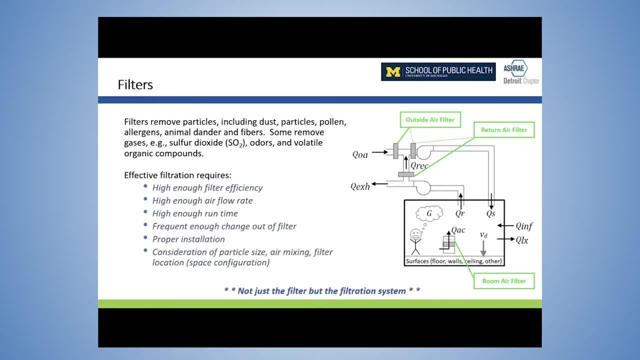 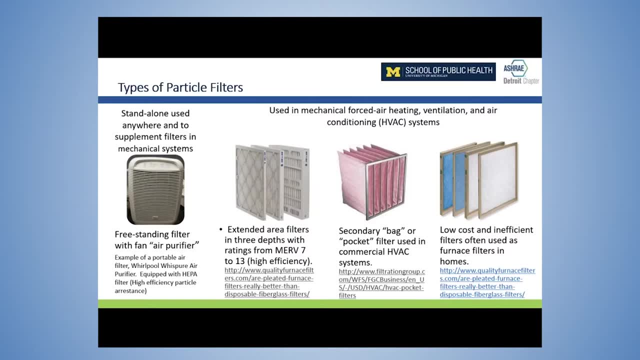 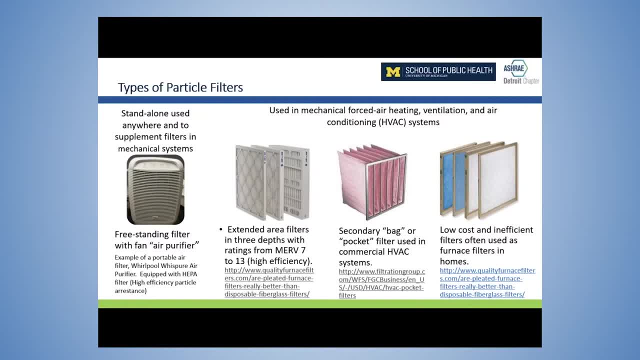 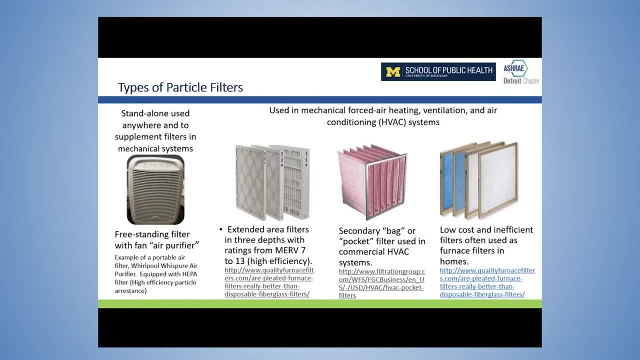 On the right we have some low-cost fiberglass types of filters rarely seen in schools, although I have seen some that are furnace filters, which basically will collect leaves and and some dust, but it won't do anything for PM2.5.. 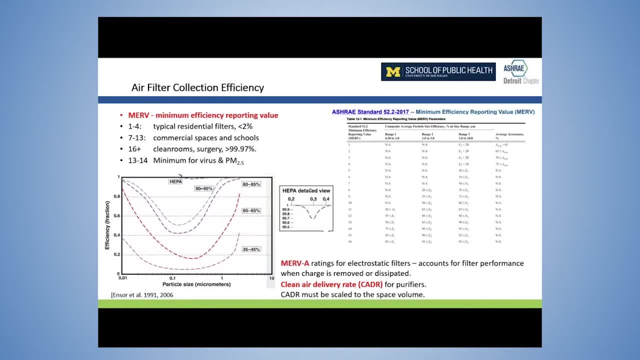 So filter efficiency is rated using several different systems. Probably the most common system is the minimum efficiency reporting value system, the MERV ratings. This is embodied in an ASHRAE code. I want to point out that when you get to smaller particles- around the size of 0.5 to 1, you 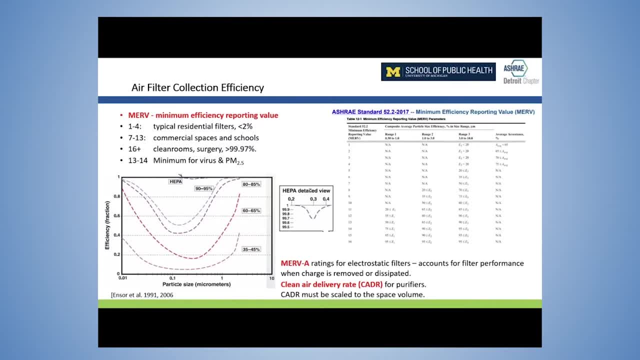 can see how the filter efficiency drops In the case of all of these different lines here. these are the sizes of particles that are very important for PM2.5 as well as for virus. Basically, a MERV filter under 11,, 12, or 13 does very little for PM2.5 or the virus. 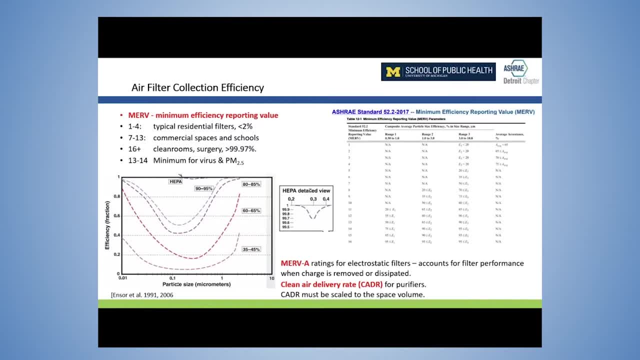 So we really recommend a minimum of 13 is a MERV rating to address PM2.5 and the virus. So think: What are your schools equipped with? I also want to mention that, for the most part, the extended area drop-in filters that are 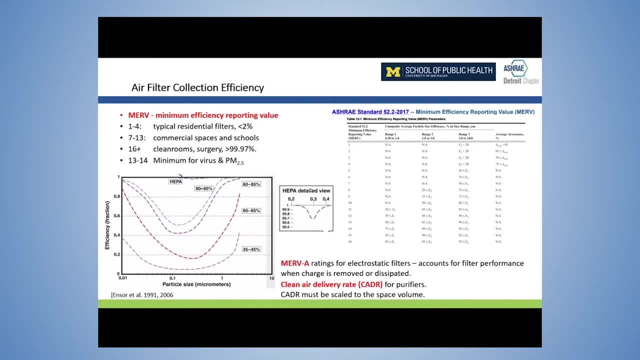 rated for MERV 11 and above are using electrostatic fibers and the MERV rating does not account for their deterioration, which occurs quite rapidly as they lose their electrostatic charge. So we have a newer MERV system called MERV-A. 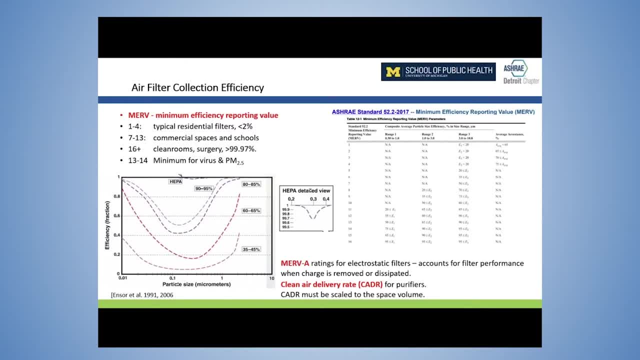 And I really encourage you to get filters that are tested, if you can, or at least demand this, because the filter manufacturers have not done this very much- Get MERV-A filters that meet your 13 requirement For a portable air filter. you also need to consider the clean air delivery rate. 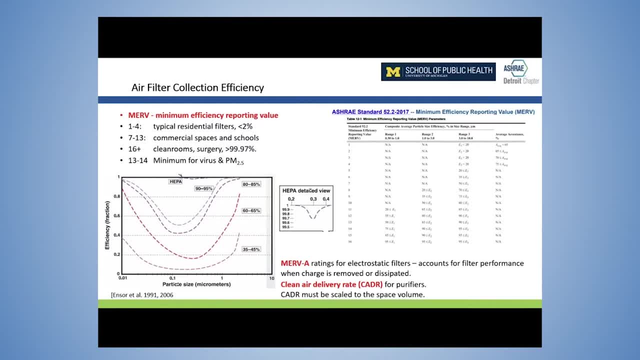 and Sonia will talk a little bit more about that Take-home point. here is a filter under 11,, 12, or 13.. It's not going to do much for you for a COVID or for PM2.5.. So what do we find in schools in the Midwest? 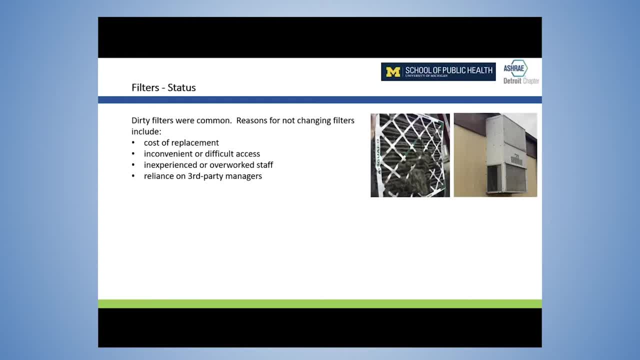 We find a lot of dirty, overloaded filters. A number of good reasons for not changing them out are listed here. We find lots of filters, misinstalled gaskets, missing. this bypass quite common. We find both dirty filters plus bypass And we typically find MERV ratings from 7 to 8 as the default. 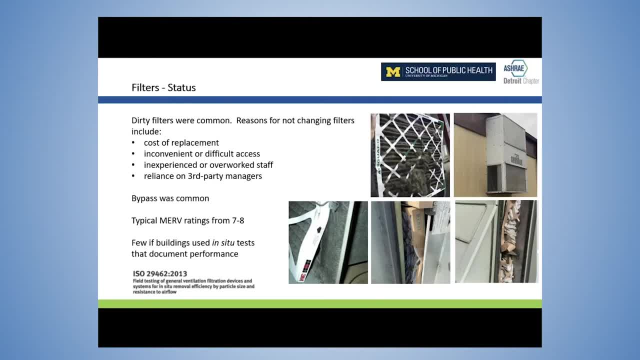 And then hardly any of the schools had institute tests that document performance of their air filtration, much less the HVAC system, despite the existence of a standard for doing so. So I think there are many opportunities to upgrade filters in schools. All right, my last slide here is: do we know if filters work? 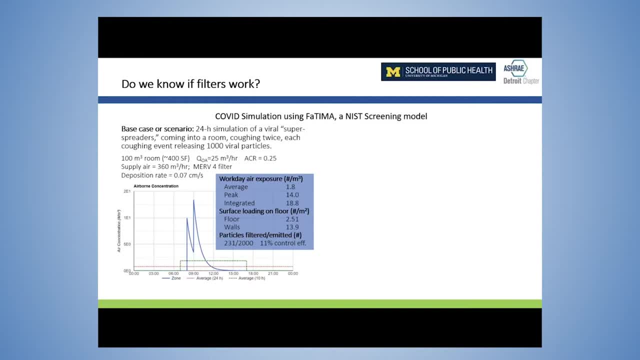 One of the issues with COVID is it's very difficult to measure the virus in real time in ambient air or indoor air. What I'm going to present here is a few things. First of all, we need to know if filters work. Here is a simulation of COVID from a super spreader who comes into a room. 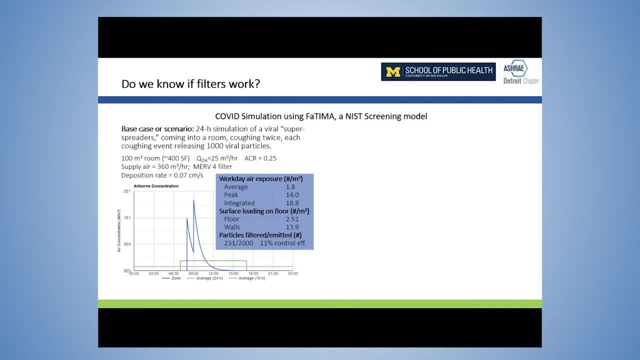 at about 8 o'clock, sneezes or coughs twice, sneezes again, maybe an hour later. And this is a prediction of the airborne concentration that you get from this sneezer, with the scenario releasing 1,000 viral particles. just an arbitrary number? 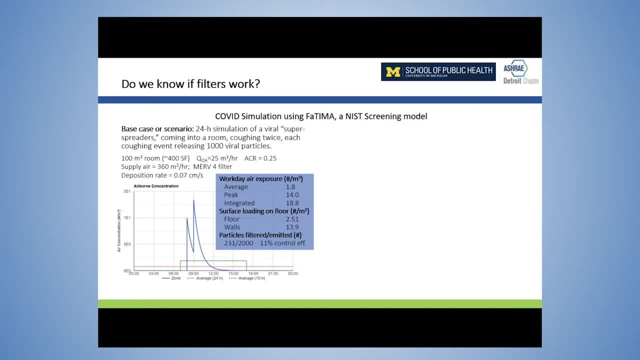 This is in a room with minimal filtration, about the size of a classroom. If we use filters, we're going to be able to measure the virus, So we put in a HEPA filter like the one that I showed you, operating at about 300 CFM. 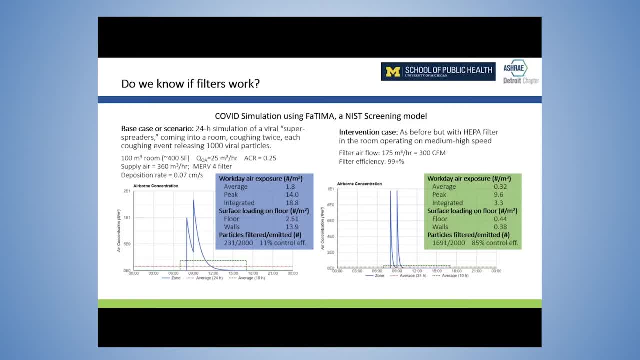 change nothing else. let this super spreader cough twice. We have a reduction in the peak concentration by about two. It doesn't sound like that much, But in terms of the integrated or the average concentration, it's fallen six times And we can see that we've in fact captured about 85% of the viral particles. 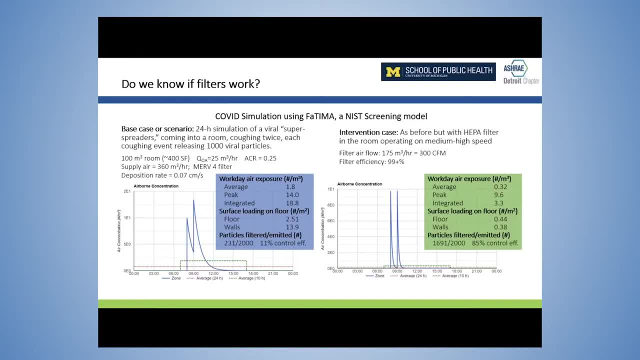 that were emitted by the filter. So this is just a model, but it's a, you know, physically based engineering type of model showing how, with higher ventilation and higher filtration, we can actually greatly reduce the exposure to COVID. I'll pause here and let Sonia take over. 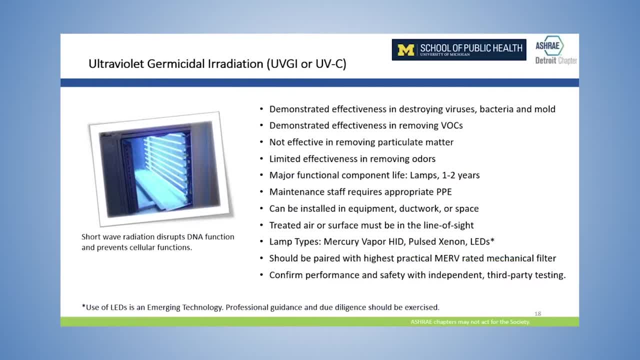 Thank you. Thanks so much, Stuart. So Stuart was talking about filters, and mechanical filters are just a real excellent strategy for the virus, And I think that's part of the strategy for providing good indoor air quality. But there are times, like now, when we want to do more, when we want to go beyond the ability. 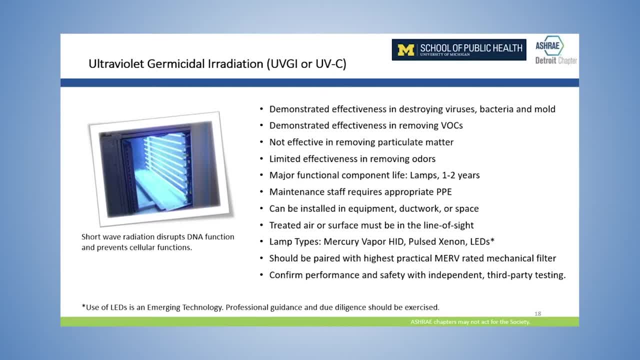 of the typical mechanical filter, And so you may want to include an advanced air cleaning technology either inside your major equipment, like your air handler or your ductwork, or standalone equipment inside specific rooms. You might look at incorporating something like ultraviolet domicidal irradiation. 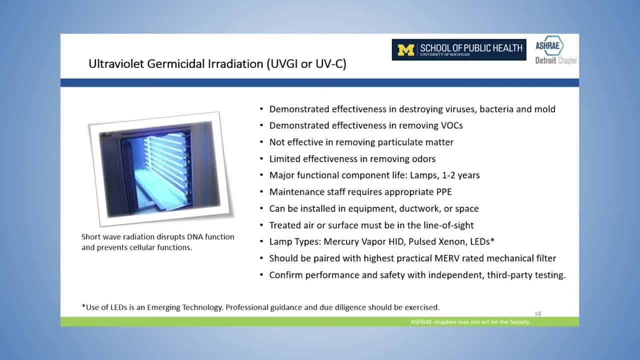 also known as UVGI or UVC or GUV or just UV. UV radiation is naturally occurring. It's about 10% of the sun's radiation falls into this category. We've known about the germicidal properties of UV for nearly 150 years or so. 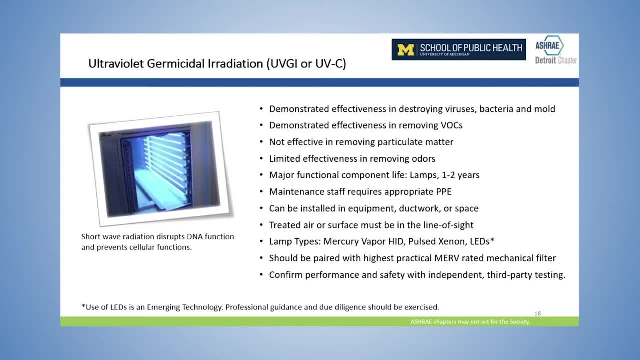 And since the early 1900s we've been developing and using UV technology in various settings, So it's got a long standing and well-documented track record of effectiveness against viruses and other microorganisms. Essentially, it works by damaging DNA and preventing cells from replicating. 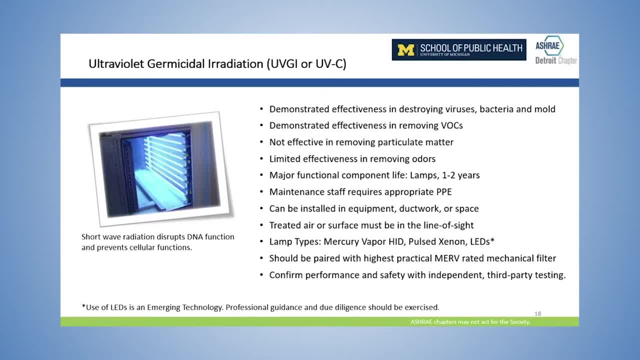 It's frequently used in hospitals, laboratories, clean rooms, municipal water treatment facilities And increasingly we are seeing it used in commercial applications like schools and large office buildings. If you're interested in bringing a technology like this into your space, a couple of things to just be aware of. 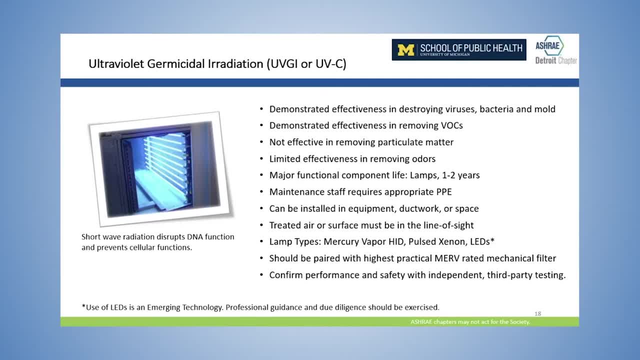 One that UV can damage eyes and it can create sunburns. So you want to make sure that staff who are tasked with maintaining this system are outfitted with proper PPE when they're involved with it, And one of the key things that you want to be aware of is that some of the newer UV technologies that you know we've been looking at energy efficiency for a number of years now. 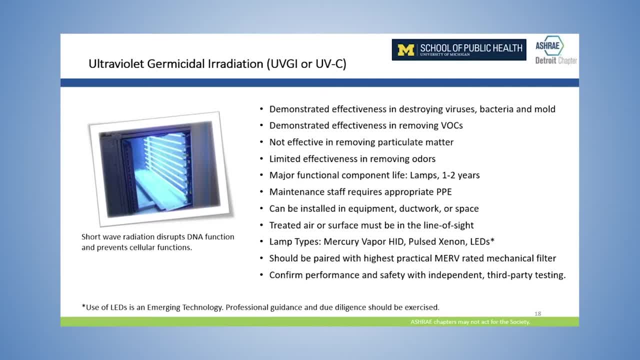 And so people have begun transitioning their lighting from older fluorescent technology to LED technology. They're looking at doing the same thing in the in the UV market, But just note that UV systems using LED lighting rather than, you know, mercury vapor or other noble gas lighting may not be as efficient or as effective as you might think. 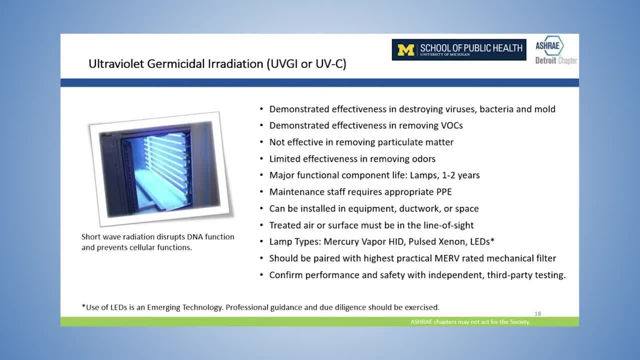 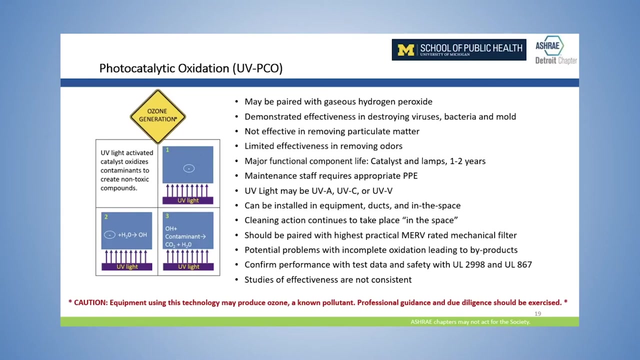 The LED lighting is more efficient in terms of electricity consumption, but it is not as efficient at deactivating viruses, And so you just want to make sure that you're exercising due diligence when you're bringing in this new technology. So, this next slide and the slide after it, so we can actually go ahead and advance two slides, because I know I've got about five people behind me, so I'm going to try to pick up the pace a bit here. 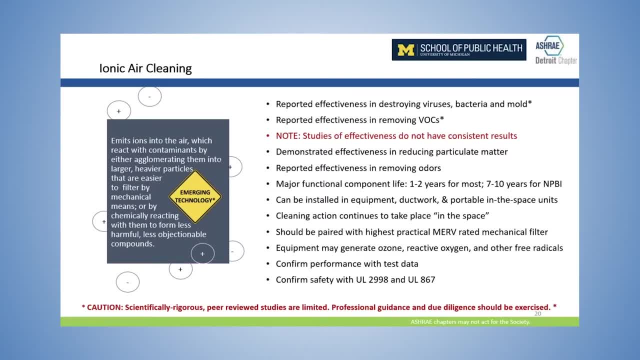 But these next two slides. they address some of the emerging technologies in air cleaning. So the previous slide that talked about photocatalytic oxidizers- those use UV light as well as a catalyst to act on water marks and so forth. So these next two slides address some of the emerging technologies in air cleaning. So the previous slide that talked about photocatalytic oxidizers- those use UV light as well as a catalyst to act on water marks and so forth. 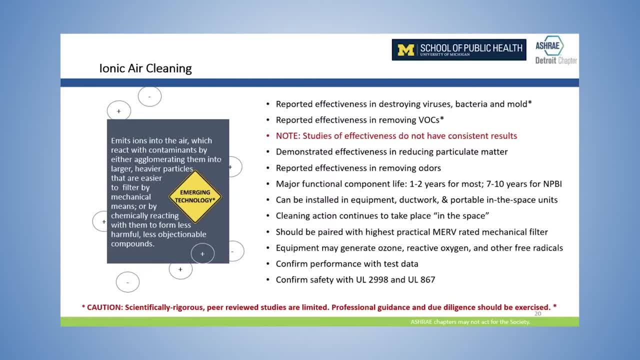 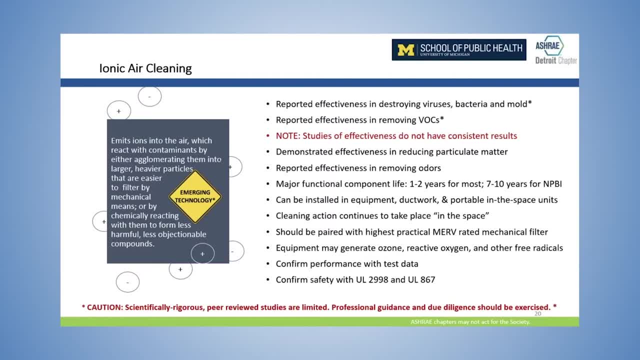 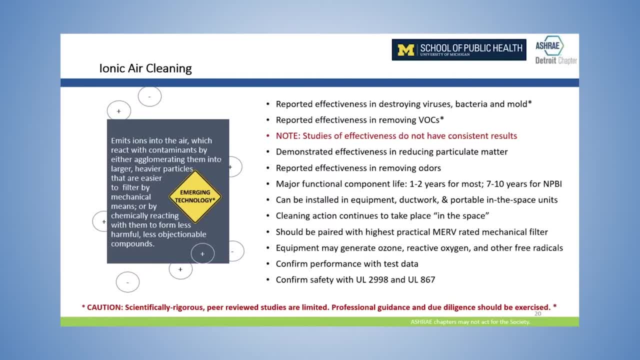 is. you know how this functions, what is its safety record, what is its performance record, things of that nature. Now, some of the photocatalytic oxidizers: they use UVA or UVB instead of UVC, So they may not necessarily be as effective at destroying pathogens, And some of 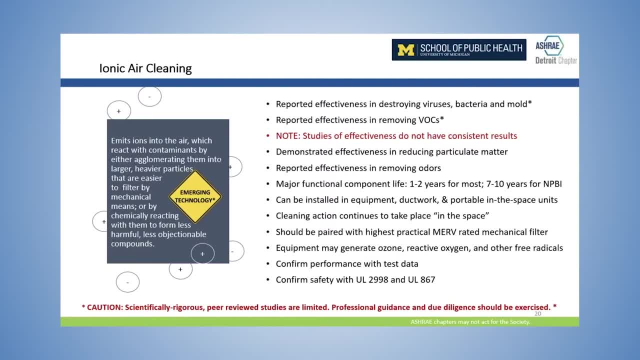 the test data for both of these technologies, the ionic air cleaners as well as the PCOs. a lot of these, the effectiveness testing has not been consistent, meaning that some studies show that they're effective, Some studies indicate that they're not effective, And so that's just. 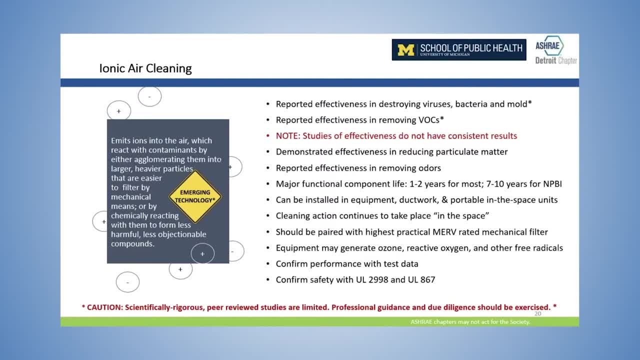 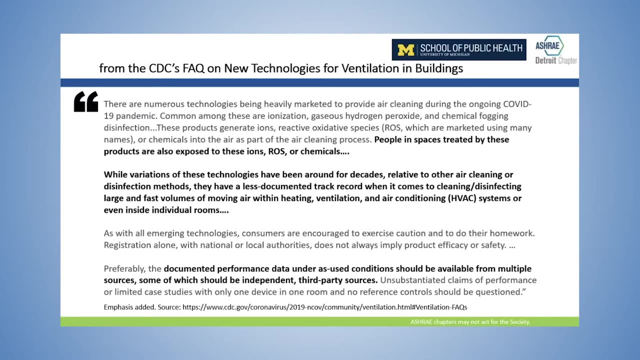 you know how things go again with an emerging technology, as manufacturers are perfecting things. That's why in the next slide you can see that the CDC is really encouraging everyone to use due diligence when evaluating technologies. This is very, very important, whether the technology is wholly new or when 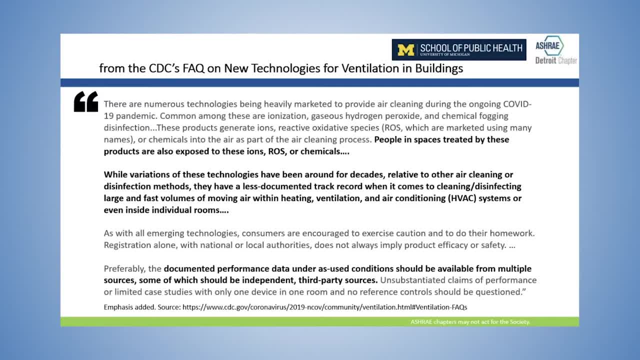 they're adaptations of older technologies, but you know they have been used in one particular application but they may not have been proven effective or safe in a new application. For example, PCO often is combined with dry hydrogen peroxide. Dry hydrogen peroxide has been used for 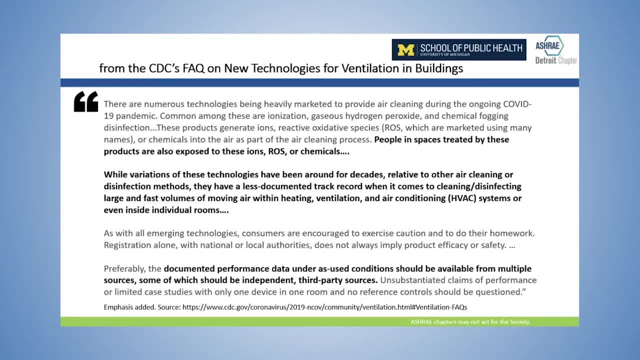 medical instrumentation sterilization for quite a while and as an alternative to steam sterilization. It's known to be very effective at sterilizing instruments in an enclosure under a vacuum with a small sealed air volume, but its effectiveness and safety moving around an occupied building hasn't been studied as much and is less understood. 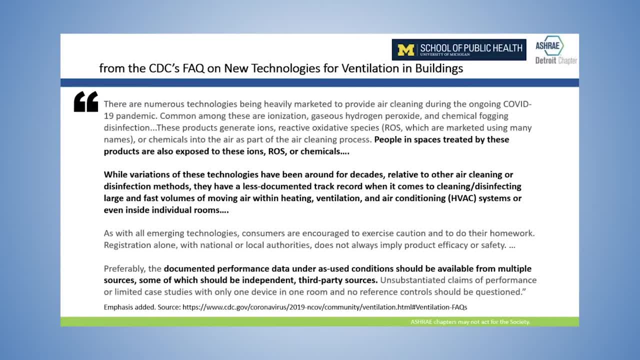 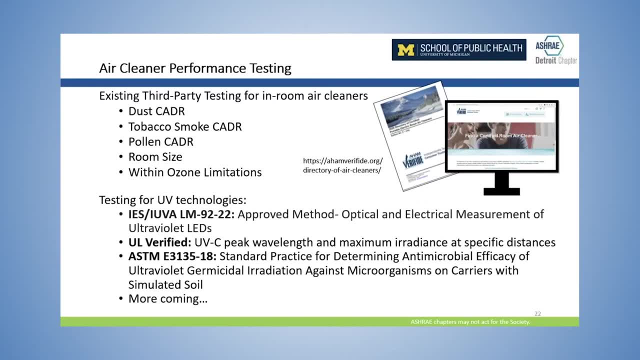 So we want to ask manufacturers and reps for data, as we can see on the next slide here, that substantiates their performance claims. right, This data should be either independent third party test data or it could be manufacturer in-house test data, but to an industry standard. 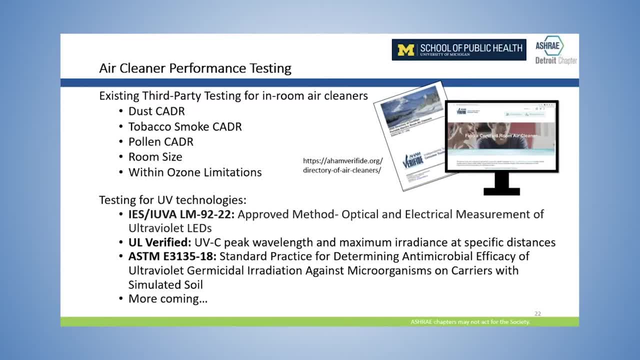 For established technologies, the test procedures are out there and you should fully expect that manufacturers are using them, and they are For newer technologies and emerging technologies. all the test data may not be there, So in that case you may ask manufacturers. 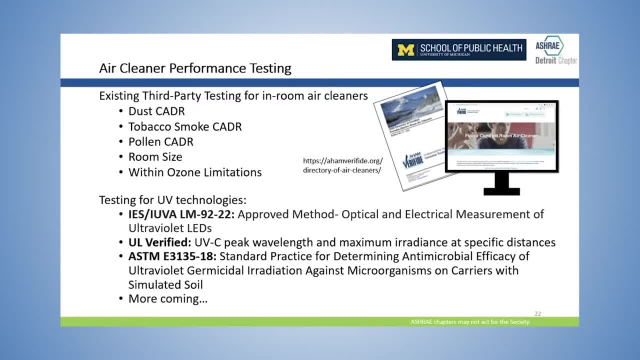 what tests are they using, or what are they planning to use, to substantiate their performance claims, And then what are the requirements of their equipment? If the manufacturer doesn't have certified test data, then perhaps ask for a witness test that reflects your specific application and be aware that new tests are coming out all the time. 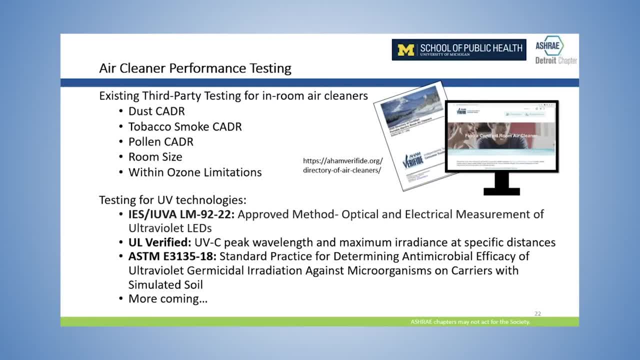 Just a couple of months ago here, IES and IUBA introduced LM92-22 to look at LEDs for ultraviolet applications. The ASTM standard package does have a LED and it does give you a little bit of a sense of the time difference between these two. 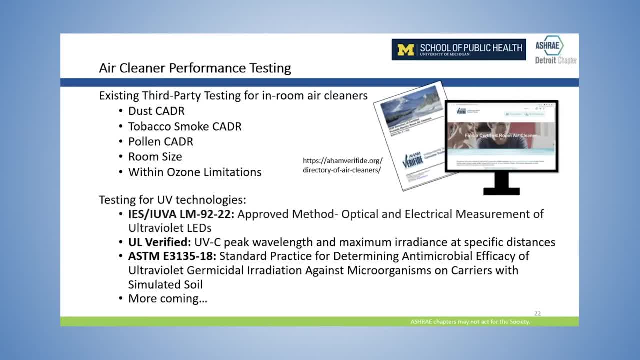 ASTM standard that's been around for a while. that's specifically looking at UV applications for surface cleaning and sterilization. AHAM, which looks at the in-room air cleaners, typically what you would see in residential and small office applications. they just introduced a new standard that looks at measuring the rate. 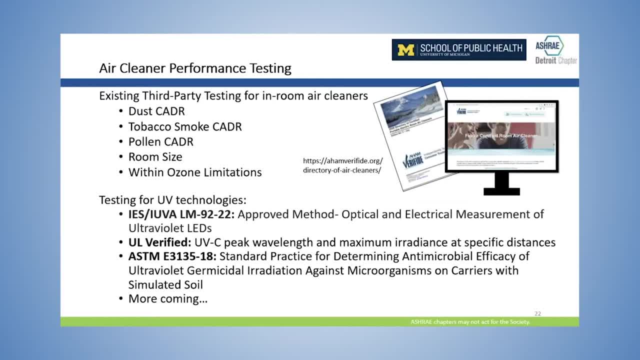 at which air cleaners reduce bacteria in the air in space. So there are new standards coming out regularly, not just because of COVID, but certainly more because of COVID. that will help us to be able to look at equipment and evaluate the operation of equipment. 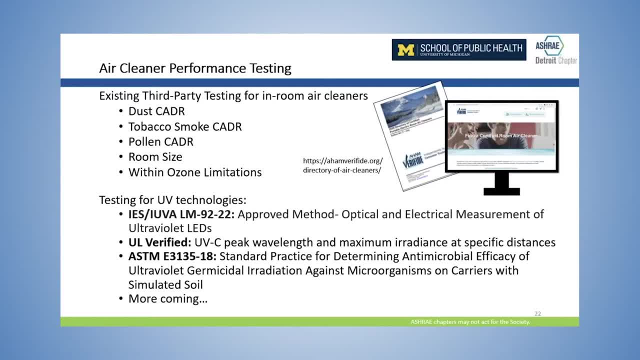 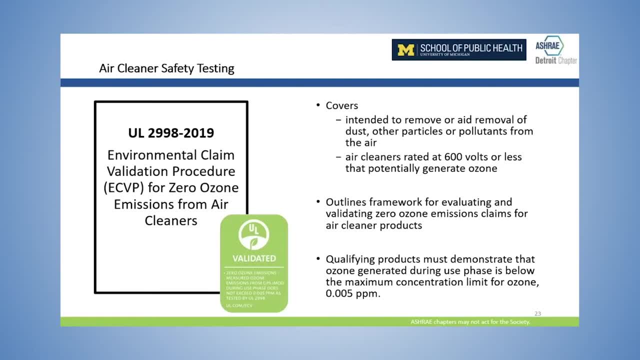 and compare one manufacturer's equipment to another. Even if that performance test data is a little bit fluid, the safety testing should not be. Any equipment you bring into a school building should have appropriate safety certifications. For example, some air cleaners have a known potential of creating ozone. 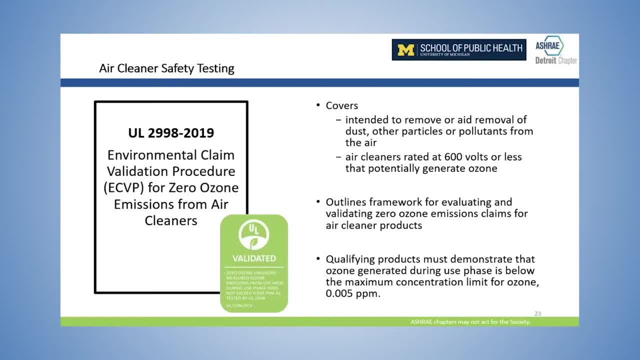 as a byproduct. We know that ozone is a pollutant, So we would want to make sure in that case, if we were bringing in in-room air cleaners, that they have been tested and that they have a UL sticker for UL 2998 certifying that they produce ozone at the low. 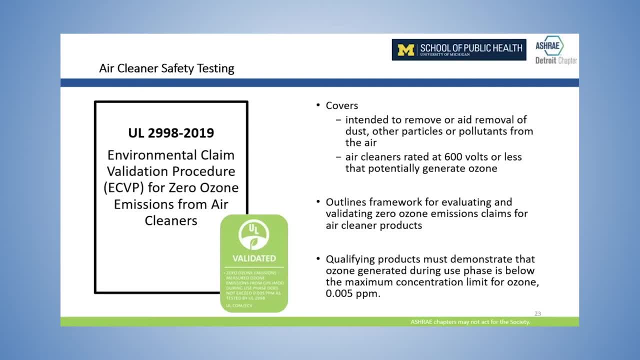 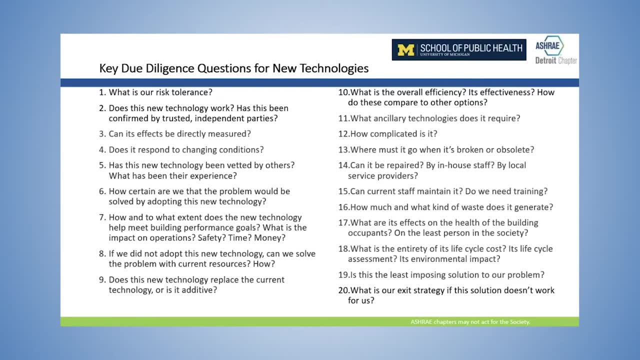 of the threshold level of 0.005 parts per million. And we don't only want to ask questions of manufacturers, We want to also ask them of ourselves. right, We want to be honest with ourselves. Can we afford to buy new equipment, Can we afford to operate and maintain and ultimately, 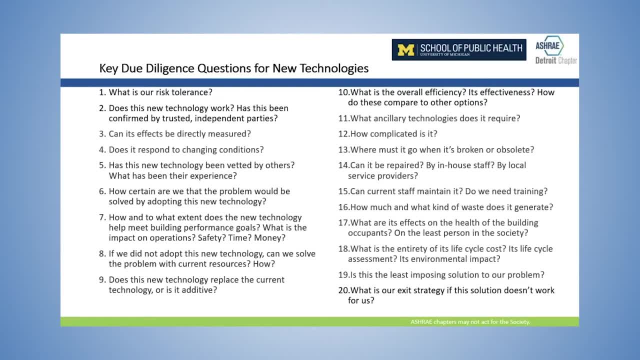 dispose of it? Do we have enough in-house staff? Does our staff need new training? Is this in our budget? What's the total cost of ownership right? These are very, very important questions. And then a very, very important question is: what do we do if this doesn't work out? You know? 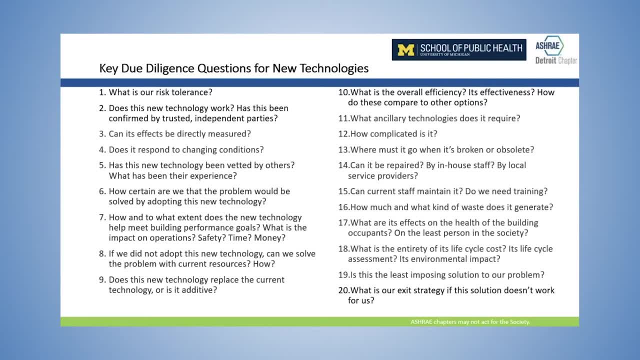 what's our exit strategy for this solution? Having the answers to the questions like these will help inform your decisions about adopting new technologies, whether they're well-established new technologies or just new to you, to your facility, And we want to make sure that we read. 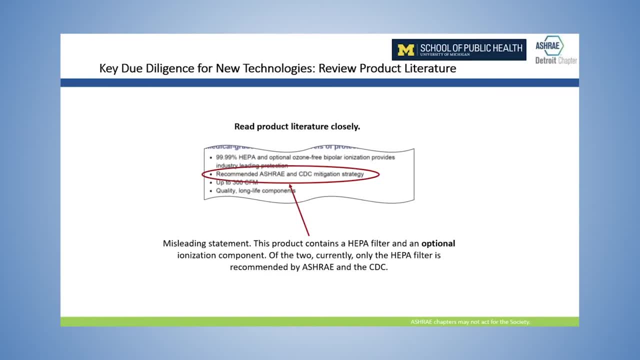 the data that we get from manufacturers very carefully. You know people aren't necessarily intending to be misleading, but sometimes the way things get worded they can be misleading. So, for example, here we're looking at a statement from a manufacturer. This piece of equipment has a HEPA filter and it also has an optional. 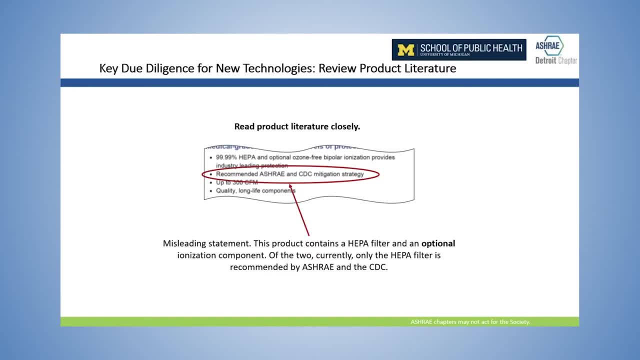 ionization component to it And it says here that it's recommended, that it's a recommended strategy, And actually it's got two pieces. It's got two technologies in there And only one of those technologies is actually the recommended technology. So we want to make sure. 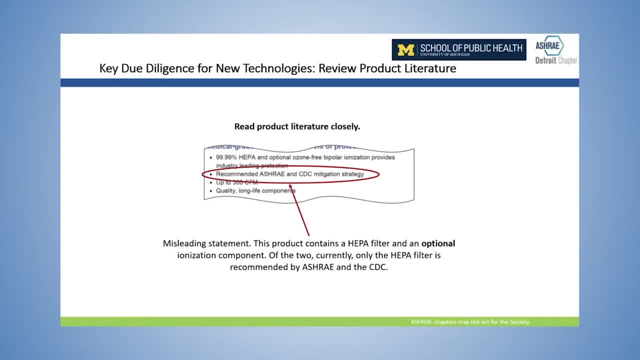 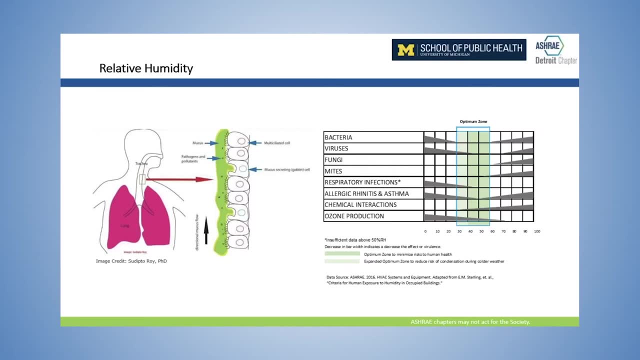 that we're understanding what we're looking at and reading the data that we get from manufacturers carefully and asking questions, asking probing questions- And I just kind of put this slide in here. I know that we haven't really talked about this much in this presentation. Stuart mentioned: 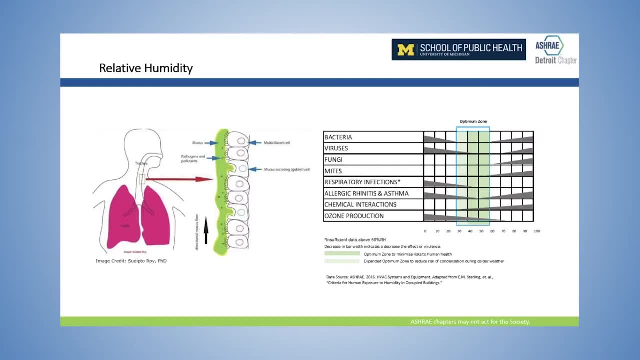 relative humidity just very briefly here, But I want to throw this in because a lot of times we overlook relative humidity. It's particularly here in Michigan. But relative humidity matters. We typically only talk about it when we're talking about what's going on outside, what's the heat index, But it matters in spaces and it matters to. 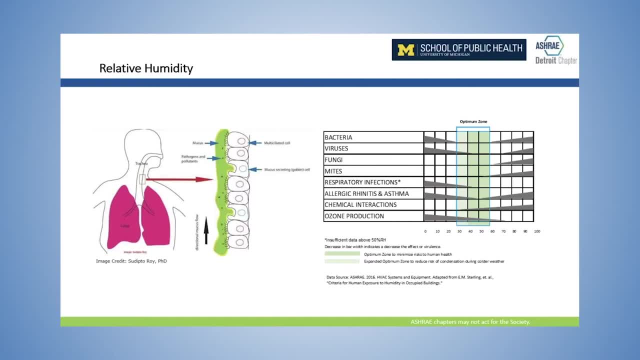 the way our bodies function in spaces. Our health depends on a proper balance of water, both inside and out. For example, when the humidity is too low or the mucous membranes in our nasal passages, they can't effectively humidify and filter out particles from the 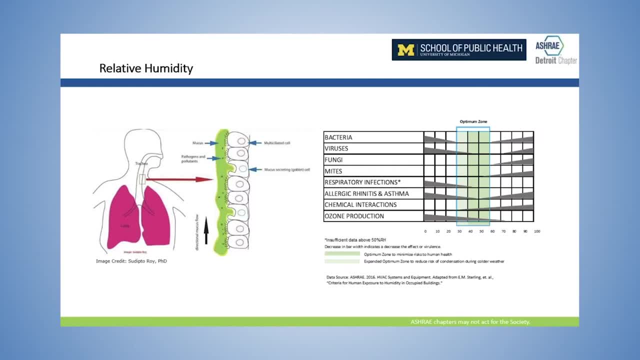 air that we breathe And then they allow those particles to travel deeper into our lungs, which can cause problems. So we want to make sure that we've got proper humidity in our spaces as well, And this slide talks a little bit about that. And interesting to note the relative humidity range that's. 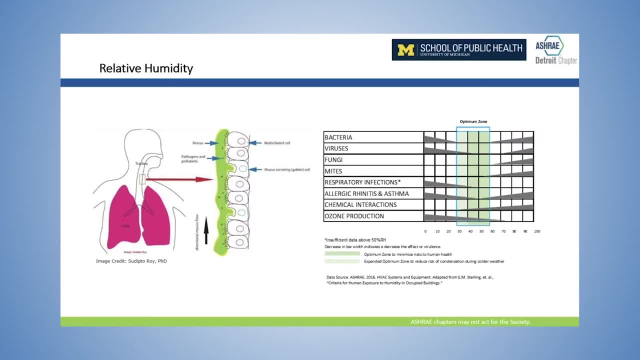 ideal for humans is the opposite for pathogens. So we like for it to be between- really ideally between- 40 and 60 percent. We have a little fudge factor here in Michigan, but we're not sure We're going to take it down to 30 percent because it's really dry in the wintertime. 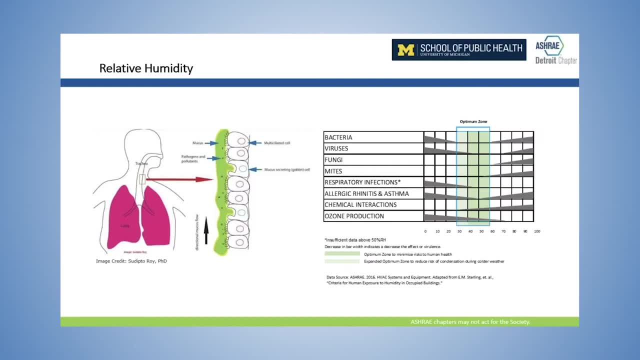 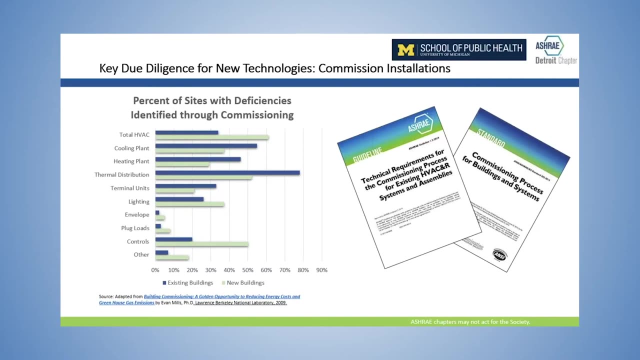 So we take it down to 30. But pathogens don't like that range. They prefer to be outside of it. They prefer to be less than 20 or more than 65 percent relative humidity. So, regardless of what kind of technology you bring into the space, there are- there have been numerous. 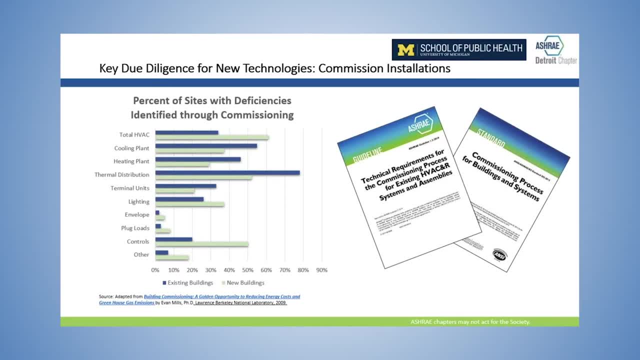 studies that demonstrate the value that commissioning plays on overall project quality, both for new and existing buildings. And then there's a number of studies that demonstrate that And I think that's a good idea to have that. But that's a good idea to have. So that's a good idea to have, And 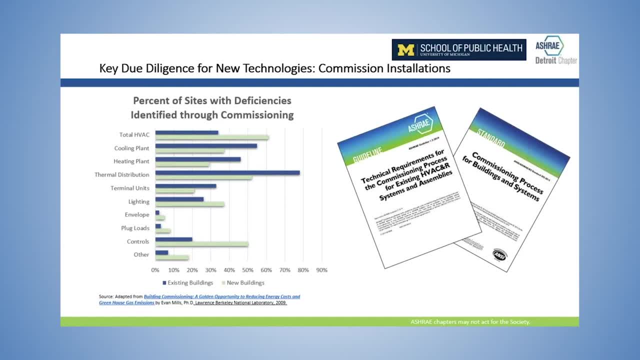 a lot of projects tend to say, oh, we can't afford commissioning, But you can't afford to not commission your projects. Commissioning is that quality assurance process that makes sure that the selected equipment is going to meet your needs, that what's delivered to the job site is correct and complete, that 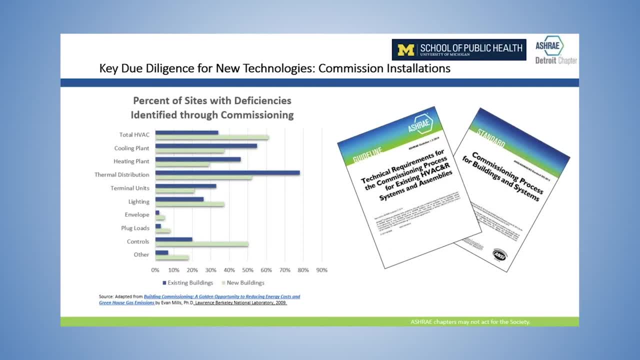 it's installed properly, that it's functioning properly And, very importantly, that your in-house staff have been trained on how the equipment should be operated and maintained, including any safety protocols And procedures that they should be following, and that they have complete reference documentation. 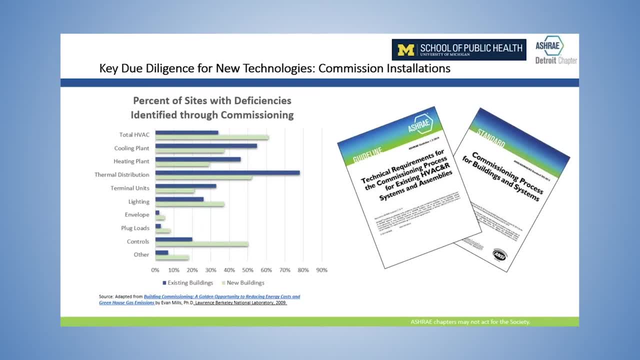 to refer to, for record keeping, for refresher training and for training of new employees. Right When folks come into the facility, they don't know how things are supposed to be working. Your documentation, your building system library houses all of the information. 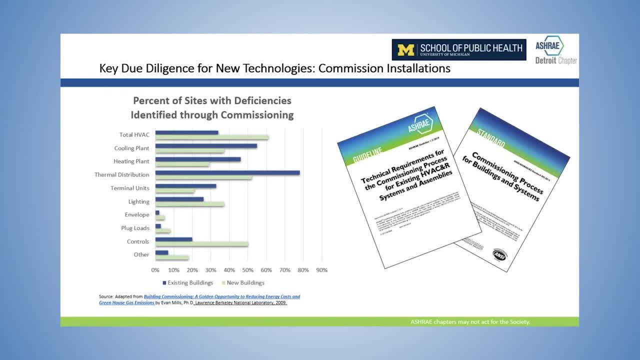 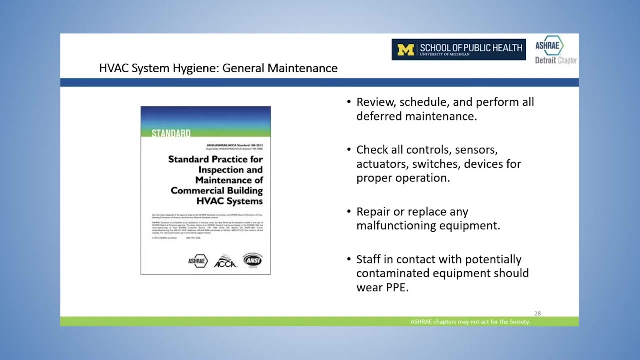 that tells them that, And having a good quality commissioning process, make sure that all that stuff is in place, which dovetails very nicely into your maintenance program, which you can see on the next slide. So one of the things that Regina and Stuart both mentioned. 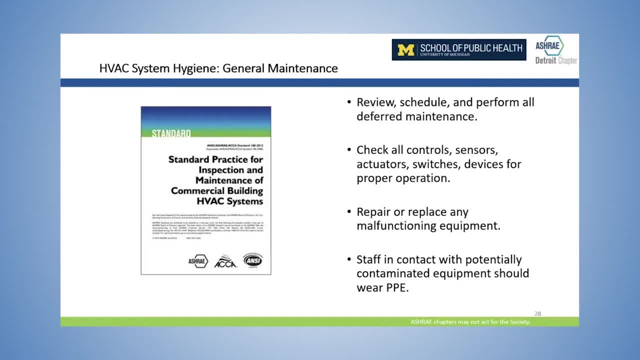 was that often one of the big problems in schools is deferred maintenance, Right, Which is really kind of a nice way of saying that broken things remain broken. But we know that the sole purpose of the HVAC equipment is to provide good indoor environment, Right. 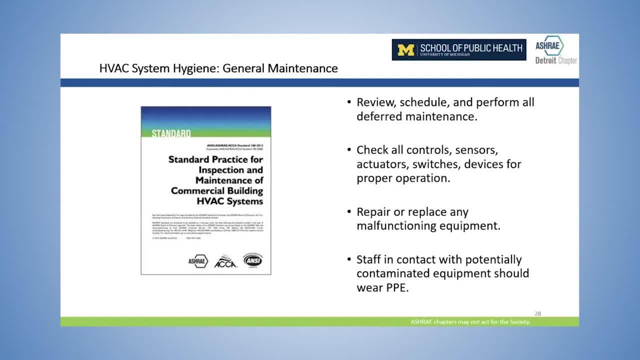 That supports student learning. So this HVAC equipment can only do its job if all of its parts work Right. The the most common unmaintained components in the HVAC system are the actuators and the sensors, particularly those on economizers that control the amount of outdoor air that's. 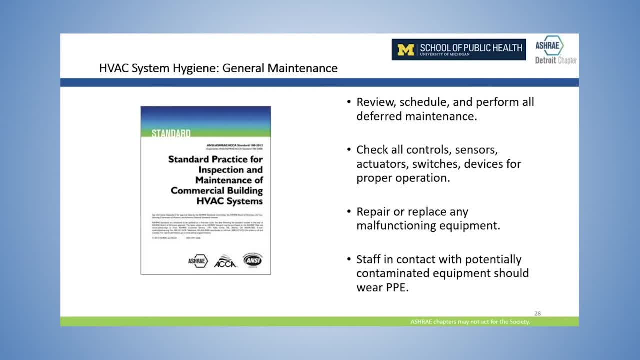 brought into the building Right And this is one of the key components. Outdoor air is one of the key components of indoor air quality. So we want to do our level best to make sure that we eliminate deferred maintenance, And we can do that, as we can see on the next. 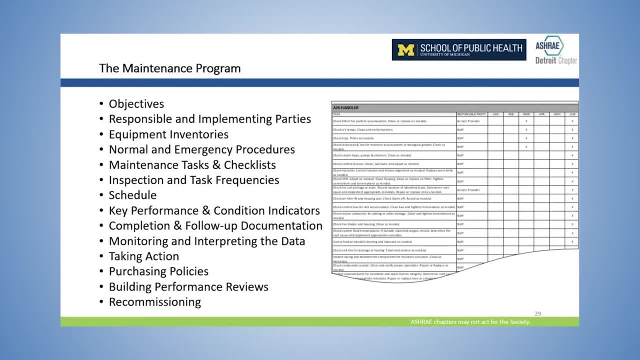 slide by starting with a good maintenance program that's tied to enterprise objectives and championed by executive level management, who expect and demand to see regular performance reporting with KPIs that connect to the goals and objectives. For example, we know that outdoor air ventilation rates impact student performance, So what are the average ventilation? 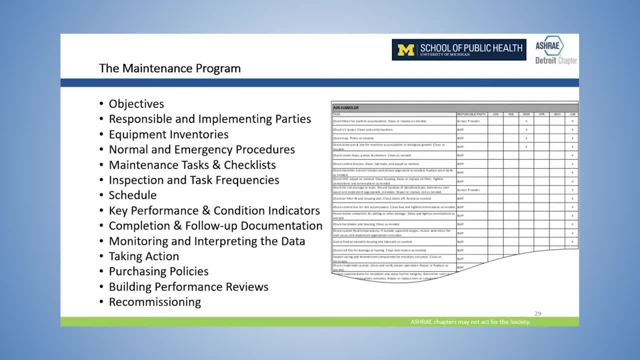 rates in each classroom. Are they supposed to be high performance? Are they supposed to be meeting high performance standards? Do they even meet minimum standards, Right? As Stuart mentioned earlier, many of them do not Right, But data from a solid maintenance program will help schools answer. 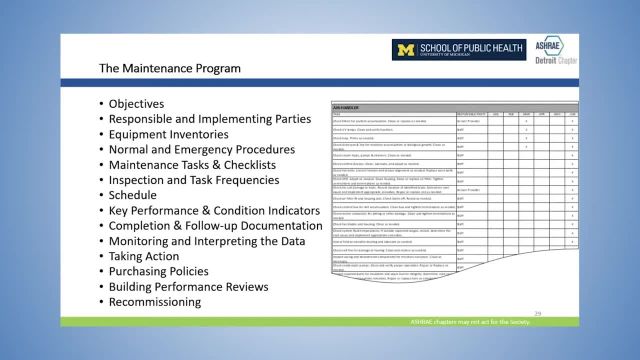 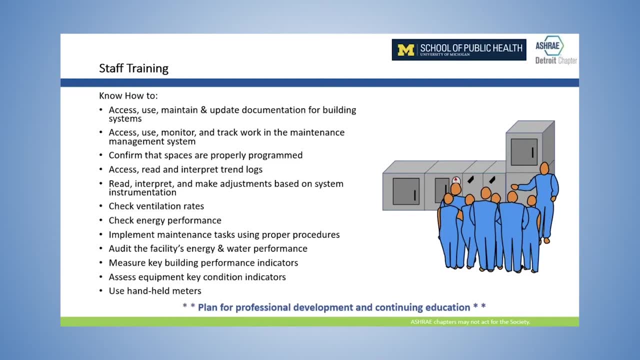 those questions real time Right. And one of the one of the other key components to facility O&M plan is staff training. I cannot stress enough the importance of regular ongoing training for O&M staff With the goals for energy performance and IAQ that we have currently across the country. 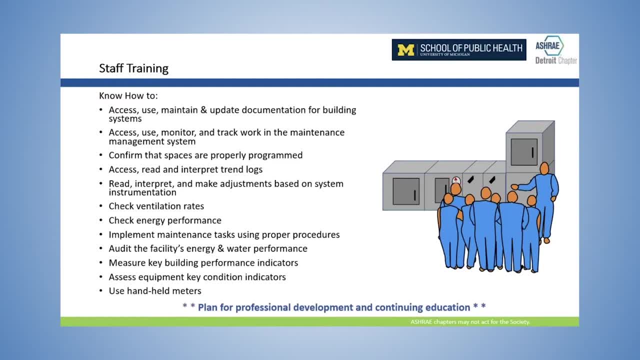 we're asking a lot of our buildings. They're becoming a lot more complex. We've got integrated controls for multiple equipment by various manufacturers: data tracking, remote operations, diagnostics, information modeling. State of technology is ever advancing. State of building technology is ever advancing and the knowledge and skills and competencies of our facility. 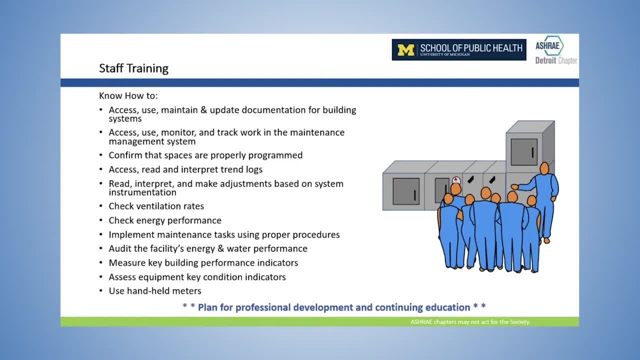 O&M staff And we're asking that we also be ever advancing. The HVAC system cannot do its job of providing a quality indoor environment that supports student learning If the personnel tasked with its upkeep don't know how to identify problems, don't know how to repair problems. 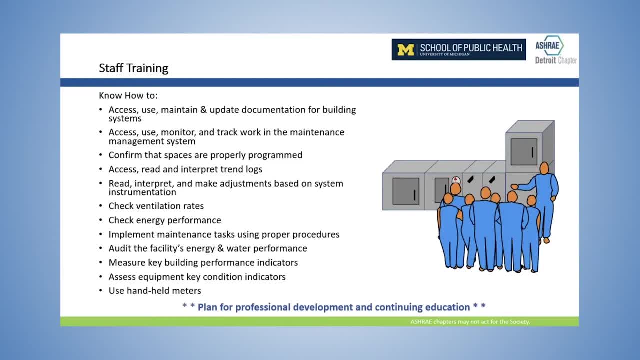 and don't understand how the HVAC system, or even their own role, impacts the whole school operation. So training should be provided not just for O&M staff, but for all of our students, for principals and other administrators, for teachers and even students, Of course. 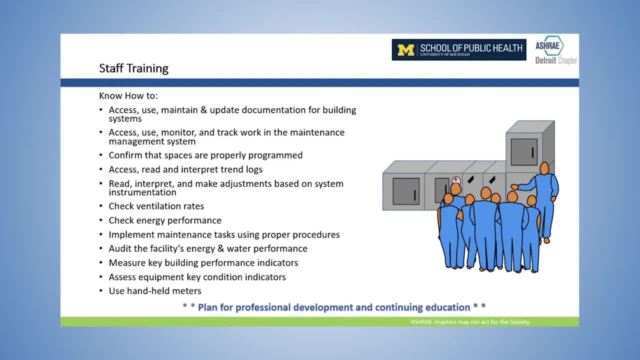 not everybody needs to know how to change the filters, but training should be commensurate with the person's role within the organization. So, for example, students don't need to know how to operate a butchiller, but it would be helpful for them to know that it's not. 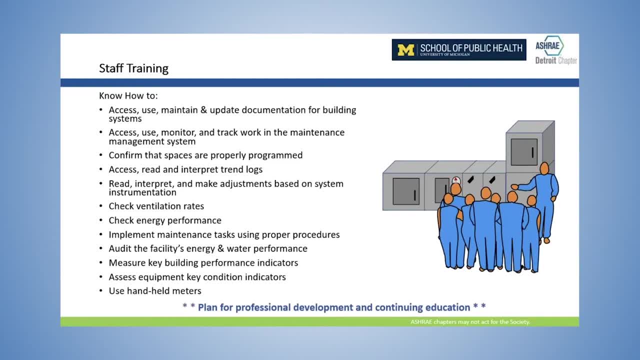 a good idea to leave crayons on the radiator. Or it may be helpful for teachers to understand that their desks shouldn't block airflow from ventilators, or where and how they should place in room air cleaners, And so some of the things here with. I'm just going to briefly, you know, talk a little. 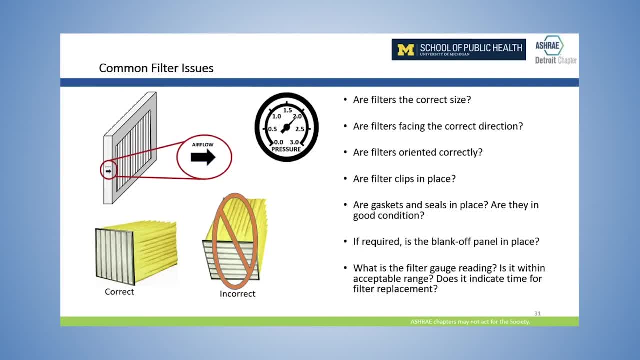 bit about the filter issues, Some of the things that I've seen in some of the assessments that I've done across the state, in schools and in other buildings as well. You know filters have a direction. If the maintenance tech doesn't understand this, they may install. 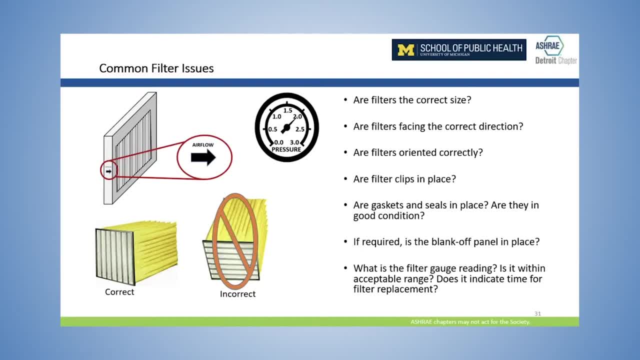 the filters backwards and then you get reduced filter performance. The filters are designed for airflow through them in a particular direction. So, again, one of the things that's out that's usually broken in the facility is the filter gauge. So how do you know when you need to replace the filter? Are you replacing it on? 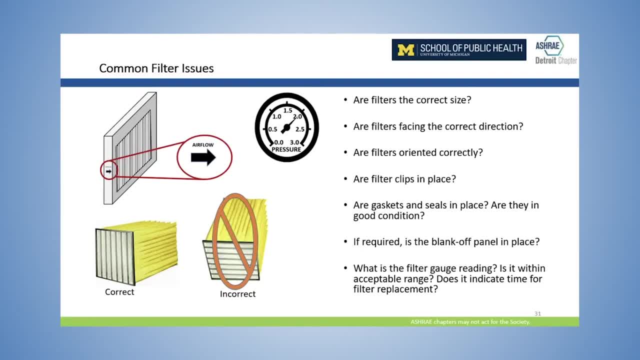 a schedule? Most cases not. So if you don't have that, that filter gauge to tell you when it's time to replace it, very often replacements happen much too late, And then you know sometimes people have they're well-meaning, but they just go over a little bit. So for 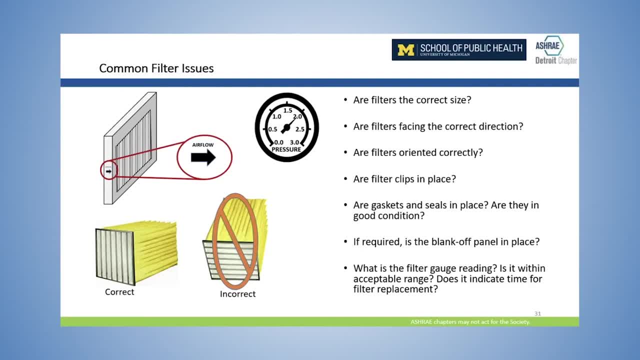 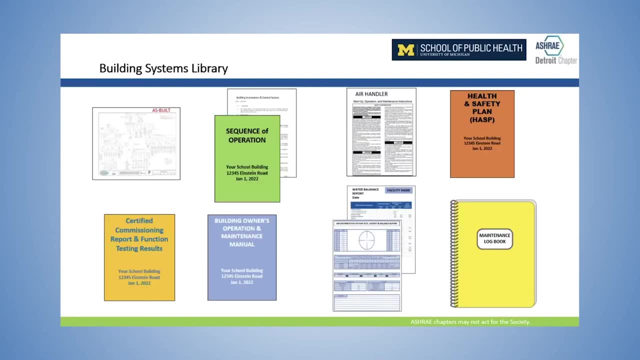 example, are the filters installed in the curriculum? Are the filters installed in the direction right? The bags should be oriented vertically, not horizontally. If you orient them horizontally, you will end up with possibly reduced airflow and higher pressure drop. Very briefly, I want to just talk about the building system library. 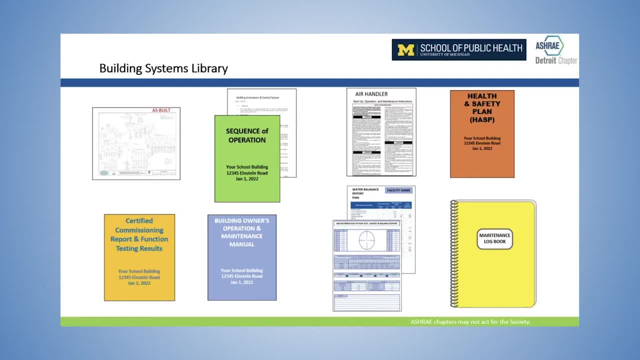 Every building needs to have one. We should have as-built documents for our facilities that talk about how they operate, how they're intended to operate and what the set points are, what the proper protocols and procedures are for startup and shutdown, And I'm going to rush through this. 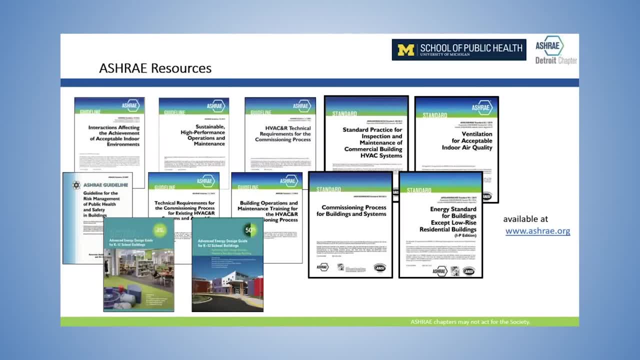 because I've got just a couple minutes here. Next slide: I want to just talk a little bit about some of the documentation that is available to assist folks that are looking to improve their building performance and their indoor air quality. There are standards for pretty much everything. 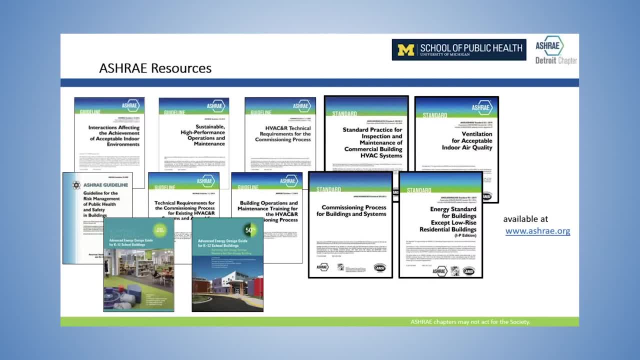 that we need to do. It's related to a building, from the design of the building and how it operates to the maintenance of the building, to the commissioning of the systems for the building. There's a number of resources here from ASHRAE, And I just want to end on this note and say that very often we 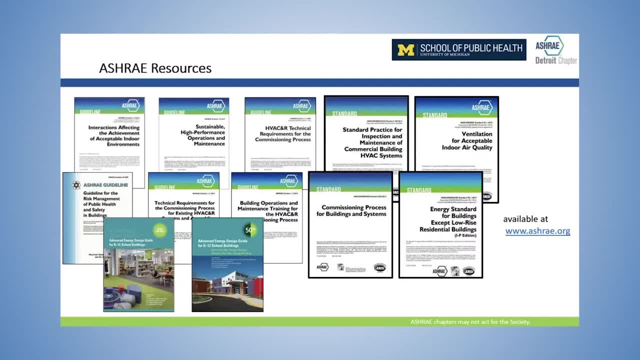 think about how that there's a conflict between indoor air quality and energy efficiency. There is not, And so we can see here in some of the documents that ASHRAE has: we have energy standards, but we also have advanced design standards for energy efficiency and facilities as well, And with that I'm going to turn. 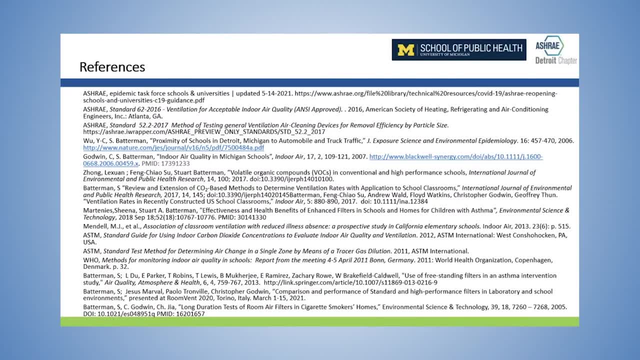 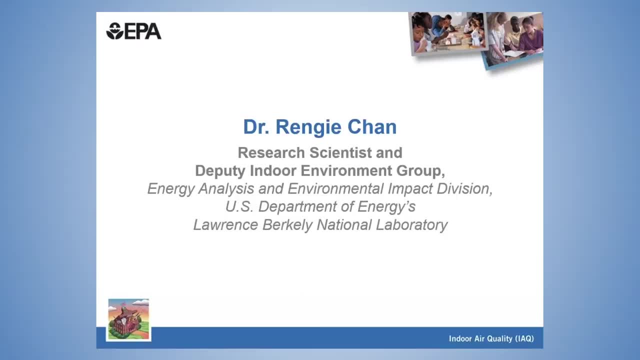 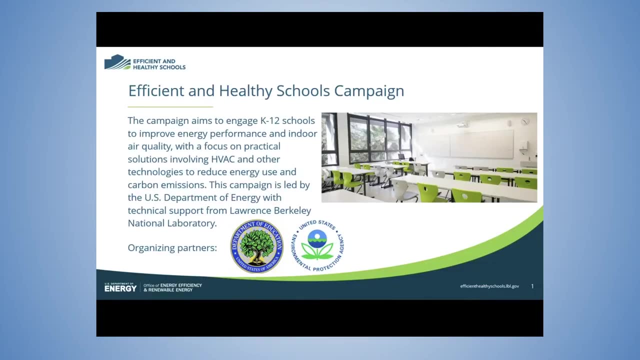 things over to Rengy to talk more about balancing that energy efficiency in buildings. We have Rengy Chan Hi Rengy, go ahead and start Rengy's with DOE, our sister agency. Sure, Thank you for having me today. 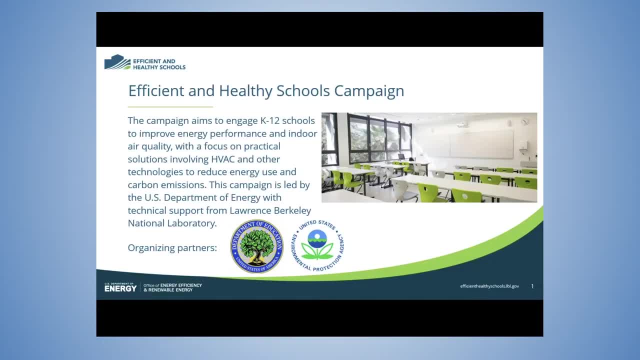 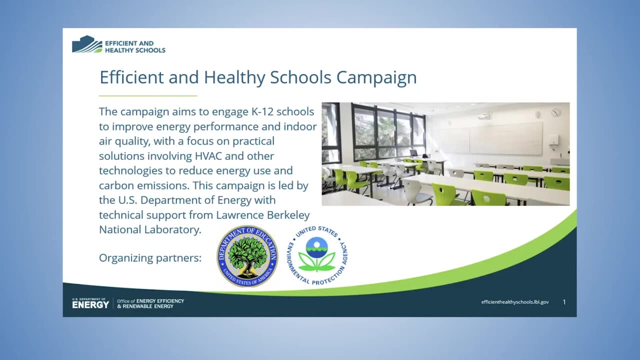 I know we're running out of time. We're running short of time, so we're going to go fast. I'm a research scientist at Berkeley Lab, leading the Efficiency in Healthy Schools campaign for the Department of Energy, And we've been hearing about the energy concern. The campaign is here to help. We're here to provide technical assistance to look at approaches that can improve both energy performance and indoor air quality. 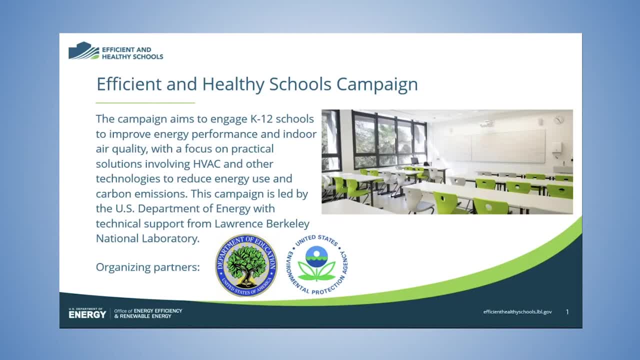 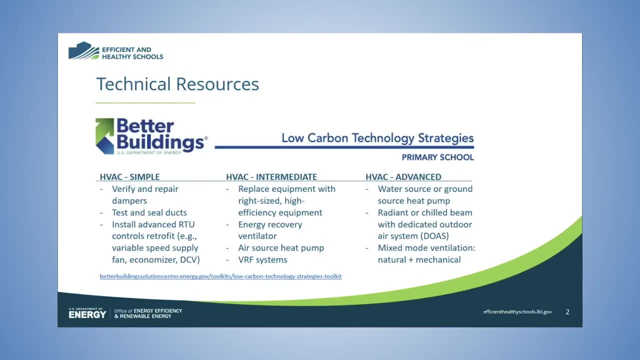 We're really lucky to have EPA and Department of Education as partners, which is really grateful to learn from the deep experience in working with schools. So today we'll talk about many approaches that schools are considering to improve ventilation, filtration and air cleaning. 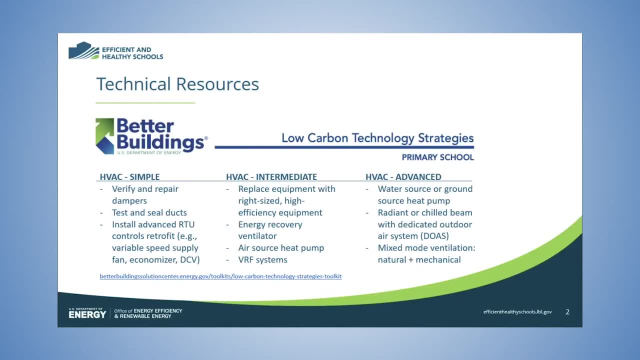 And we recognize that some of these measures will increase energy use, but note that there are strategies to lower your overall HVAC energy use. There's some relatively simple things you can do: making sure things work, like some are seeing the commissioning. making sure your air dampers work. 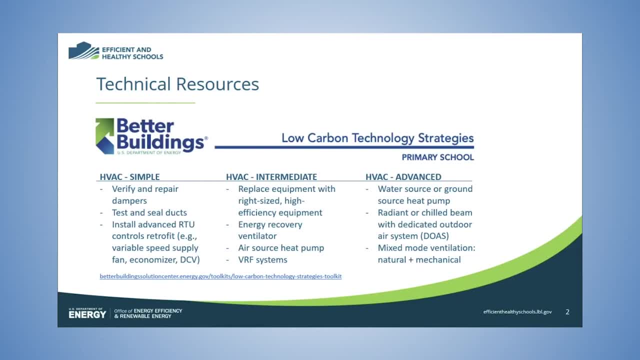 Do air duct ceilings. Install advanced controls such as Economizer. Make sure that Economizer works. Okay is working. So all those are relatively simple And as you think about the greater energy saving that you can achieve from replacing your system, there's where some of the resources 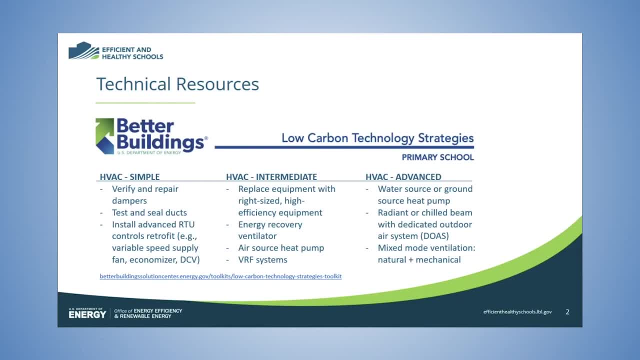 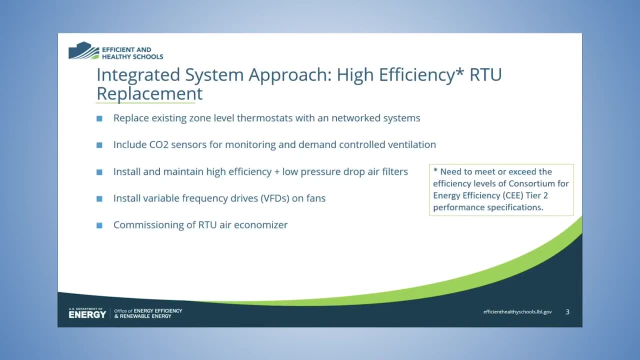 that the Department of Energy, on the low carbon technology strategy toolkits, can help give you some guidance and good technologies to consider If you are retrofitting, replacing your system. we're really encouraging your schools to use the integrated system approach. So first start with the high efficiency equipment. Be really explicit in your performance. 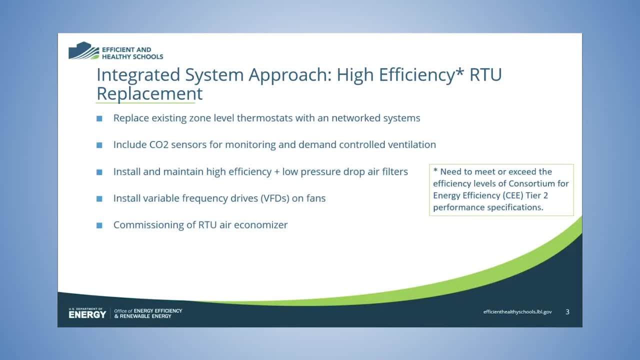 specification of what efficiency equipment standards that you want to hit, and then layer on top of measures that can get you further. For example, you will want to replace your existing Sono level thermostat with a network system, And better if you can include your 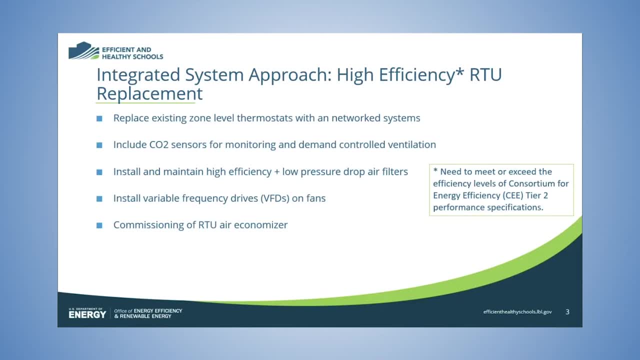 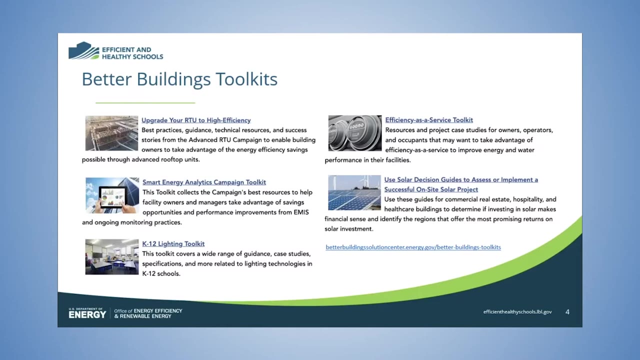 CO2 monitoring better, if you can do those filter rack design that Sono was showing you so you can achieve high efficiency, low pressure, drop infiltration, And if you even think of bigger, to go beyond HVAC and look at all the other synergies that you can get from doing retrofits. 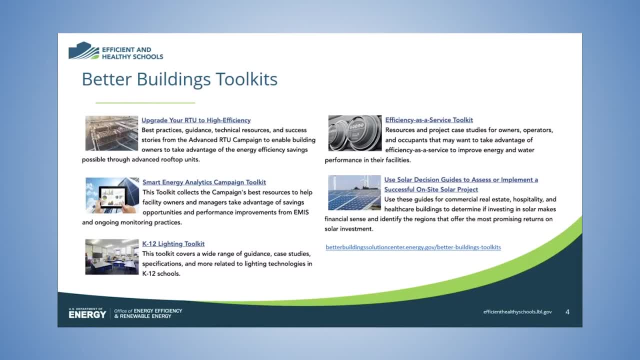 on your building technologies. So if you're thinking about lighting, if you're thinking about air energy analytics, the Department of Energy has a better buildings toolkits. really encouraging of you to go check it out so that you can think through more holistically. 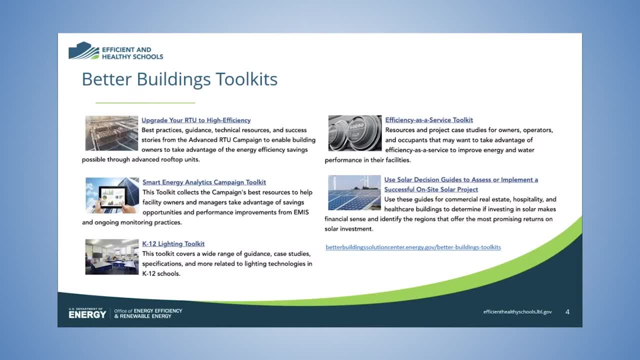 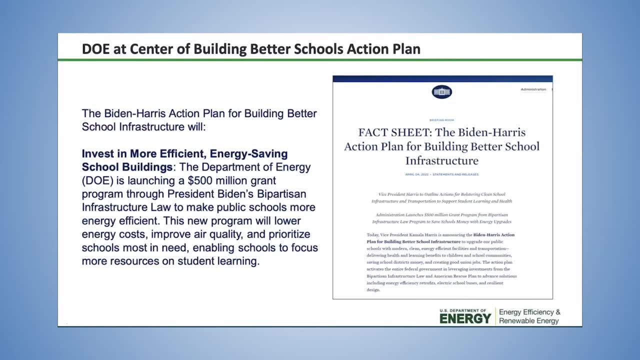 How can I really get at those good energy savings as I improve indoor air quality? So Tracy already mentioned the American Rescue Plan funding and the Department of Energy is also launching their 500 million grant program through the bipartisan infrastructure law to make public school more energy efficient. 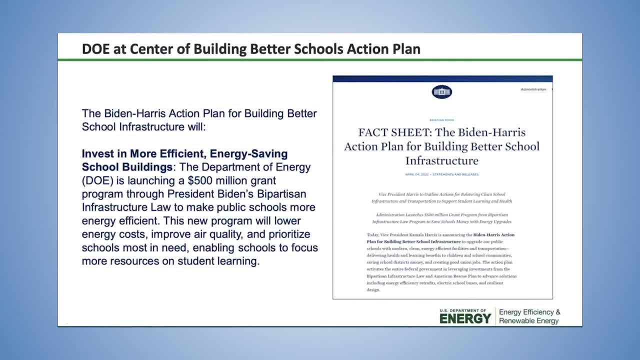 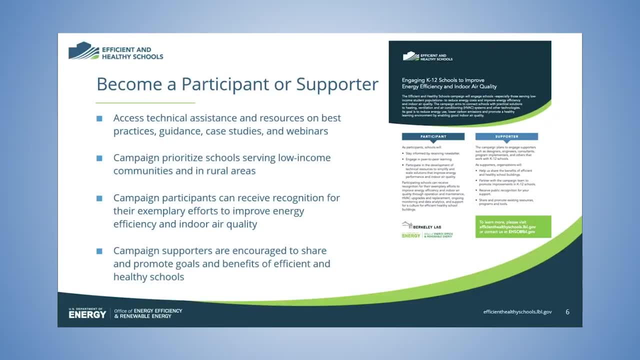 And the programs really aims to lower energy costs, improve indoor air quality and prioritize schools that are in those in need. So really encourage you to join the campaign. We're here to help, whether you're interested in direct technical assistance, Recognition opportunity or just want to learn more about the- all the opportunities. 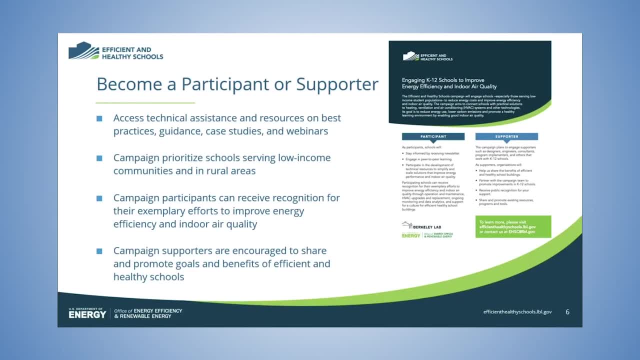 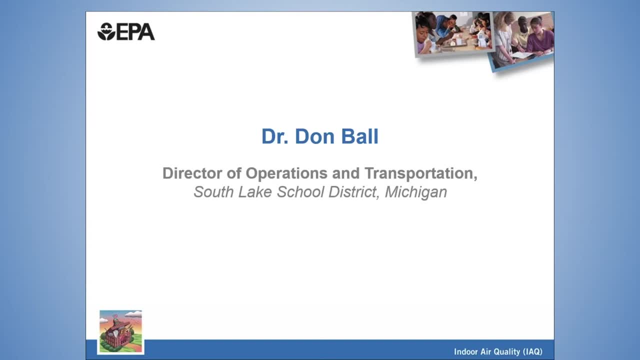 and resources that the Department of Energy has offered. Please sign up here to help. Thank you All right, so we've now reached the part of the webinar. we'll be hearing more from folks that are on the ground in the school district. So first up we have Dr Don Ball, the Director. 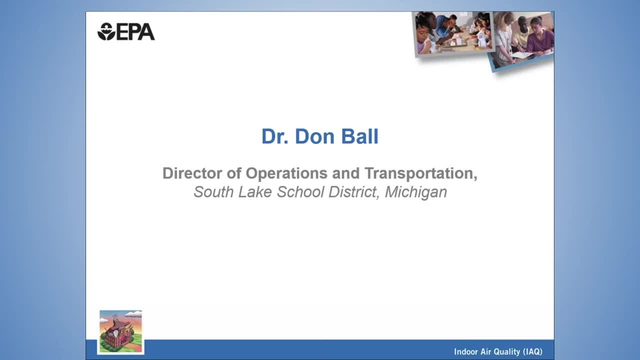 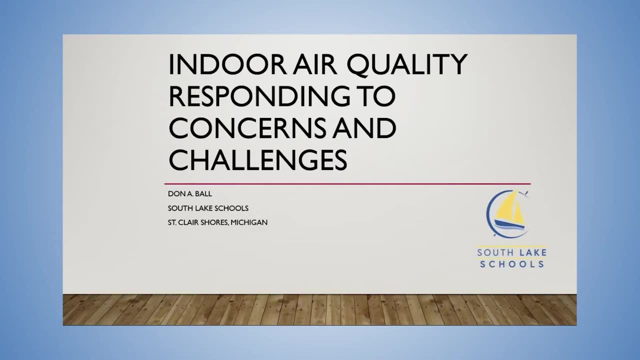 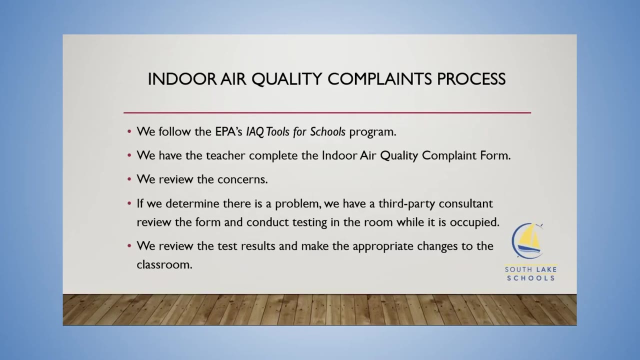 of Operations and Transportation for the Southlake School District. Hi, I'm Don Ball, Director of Operations for Southlake Schools. I have 26 years experience in schools with indoor air quality. Okay, right now, the model that we follow is the EPA's IAQ Tools for Schools program. 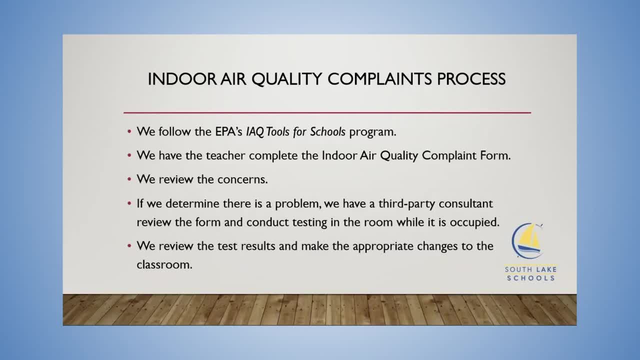 We have a teacher has an issue with indoor air quality in their classroom. We haven't complete the indoor air quality complaint form. We review the concerns. If we determine there is a problem, we have a third-party consultant review the form and conduct testing. 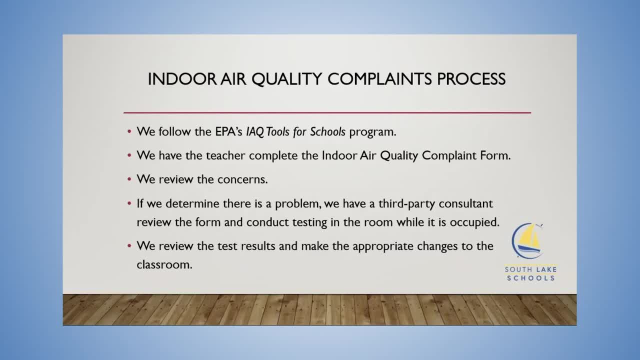 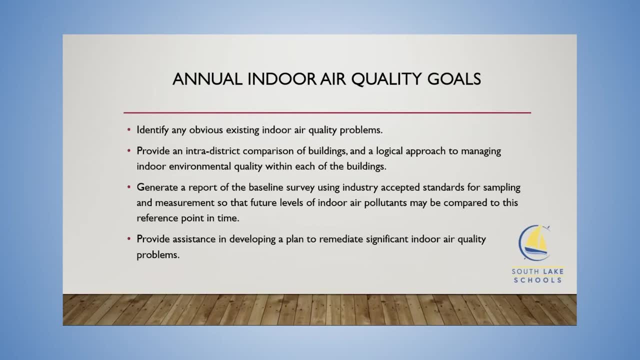 in the room while it's occupied. We then review the test results and make appropriate changes to the classroom. Our indoor air quality goals are to identify any obvious existing indoor air quality problems, provide an intra-district comparison of buildings and a logical approach to managing indoor 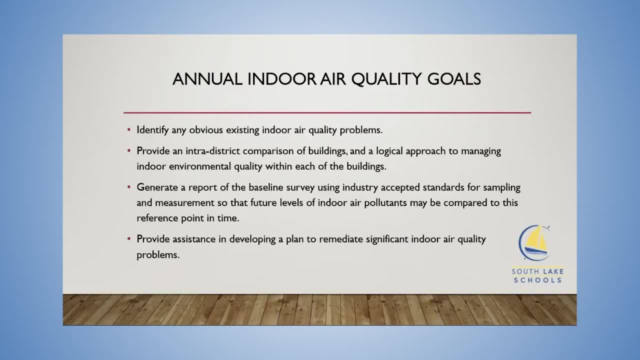 air environmental quality within each of the buildings. We generate a report of the baseline survey. We review the standards for sampling and measurement so that future levels of indoor air pollutants may be compared to this reference point in time And then provide assistance in developing a plan to remediate significant indoor air quality problems. 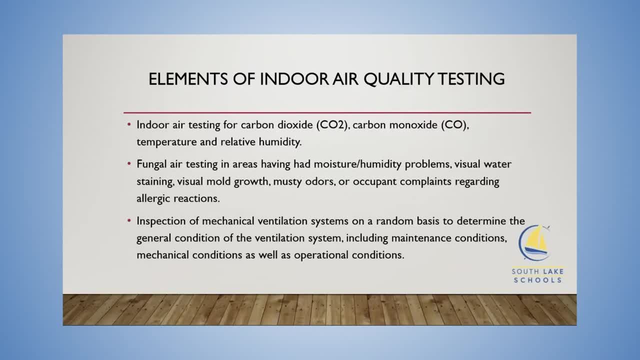 Our indoor air quality testing is for carbon dioxide, carbon monoxide, temperature and relative humidity. We do fungal air testing in areas having had moisture humidity problems, visual water standard and temperature and relative humidity. We provide physical and staining, visual mold growth, musty odors or occupant complaints regarding the allergic. 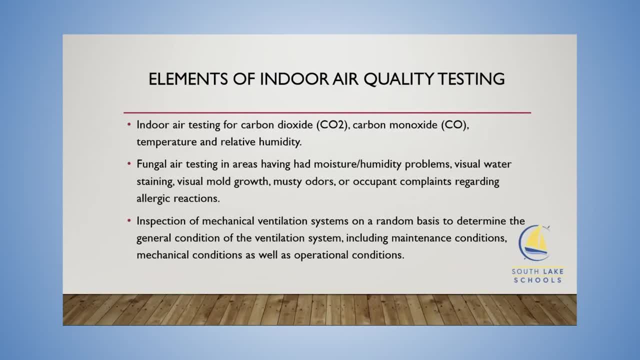 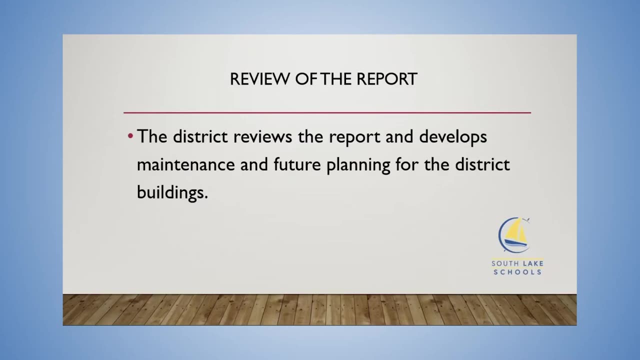 reactions that they may be having. We also inspect mechanical and ventilation systems on a random basis to determine the general condition of the system and include maintenance conditions, mechanical condition as well as operational conditions. The review of the report. We review the report and we develop our maintenance and future planning for the district buildings using 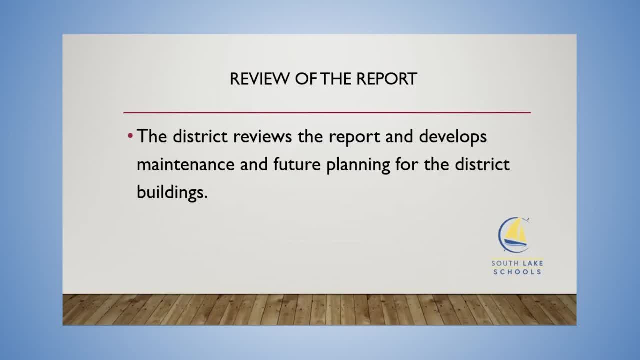 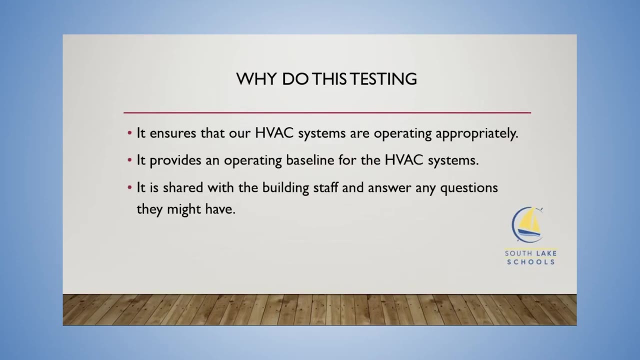 that report. We do this on an annual basis for all the buildings in the district, so we have a baseline moving forward to see what needs to be changed on a yearly basis and make sure that our preventative maintenance programs are in good shape. So why do we do it? Our testing ensures 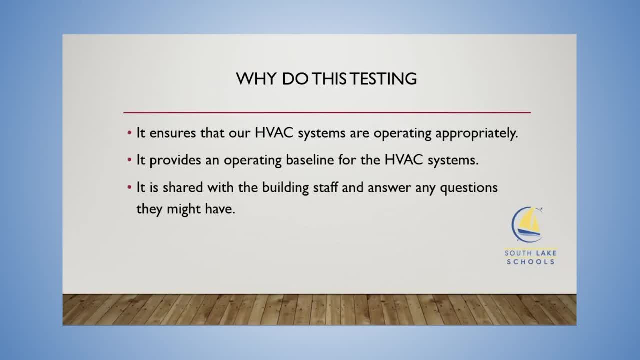 that our HVA systems are operating appropriately. It provides an operating baseline for our systems and is shared with the building staff and answer any questions that they may have. Now I'm going to hand you off to one of my colleagues, I believe Peter's, up from. 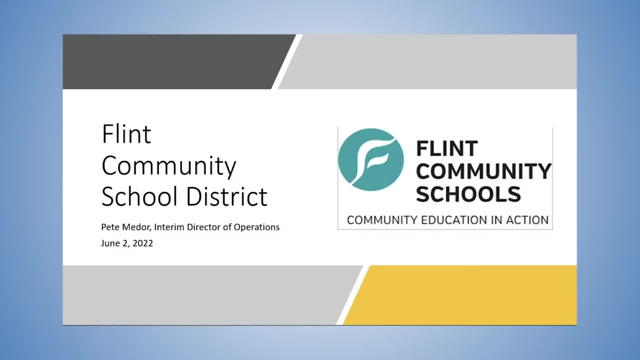 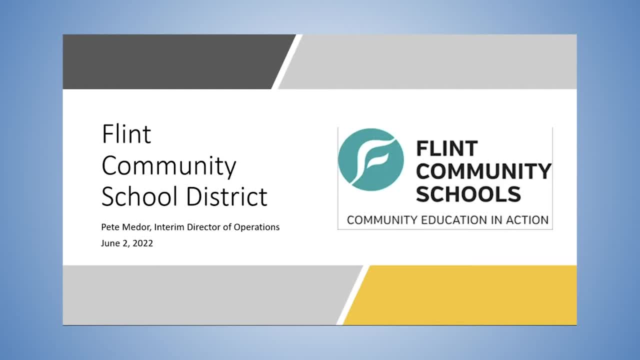 joined the administration staff as interim director of operations and taking that position, obviously I knew what I was getting into. I understood all the infrastructure and mechanical and variety of issues that I inherited by coming on with the, with the Flint administration And in the last eight months I've been 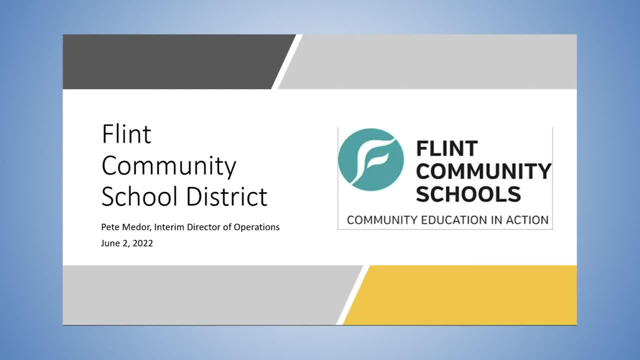 I have been addressing as many issues as I can And, of course, a few years back, when the pandemic started, that was our air quality issue. But if people remember the history of Flint, back in 2014,, we have a water quality issue. So we've been addressing that as we go along. But now, with the COVID putting a hot white spotlight on all air quality, I am impressed with the work that you're doing And I'm very happy to be here, Thank you. 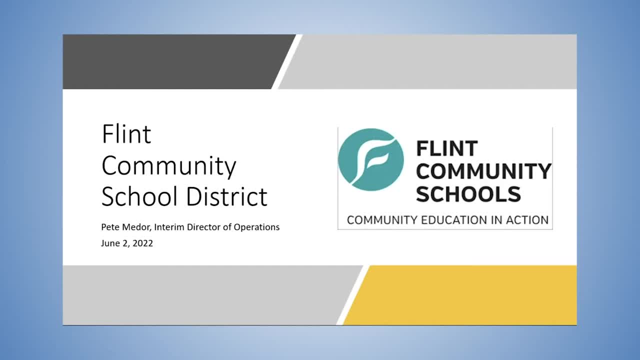 I'm in my research mode right now And I have been so blessed to have the EPA come on board and to assist me, give me guidance and hopefully it will evolve into some good, positive decision making as we move forward, as we work on our buildings, keep them operational and to improve them to the best. 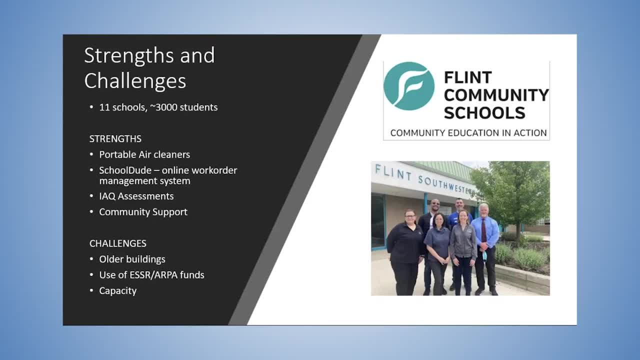 we can. This is a picture of my my new friends at the EPA And with Melissa and Monica Camden, Jeanette, we went through four different buildings in Flint schools And I think they got a good idea of what what we're in store for as we move forward with making improvements. 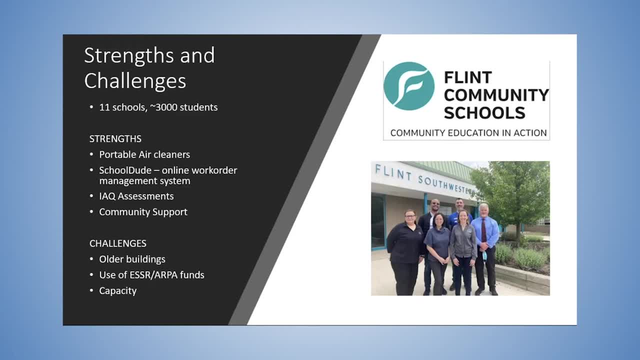 Pictured here in front of the Flint Southwestern Academy, which is our high school now, And we've been serving a lot of our students for a long time. We've been doing a lot of work with our community And we're very proud of that. 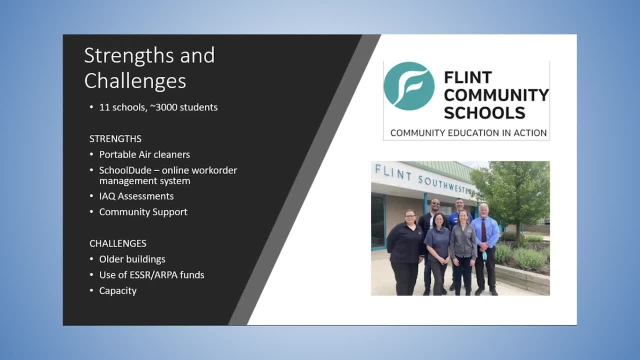 And we're very proud of that. At one time Flint had four high schools, is over 3000 students in them, And now we have just one high school, one junior high and nine elementary schools. So the district is shrunk dramatically. We still have 11 buildings and roughly 3000 students. 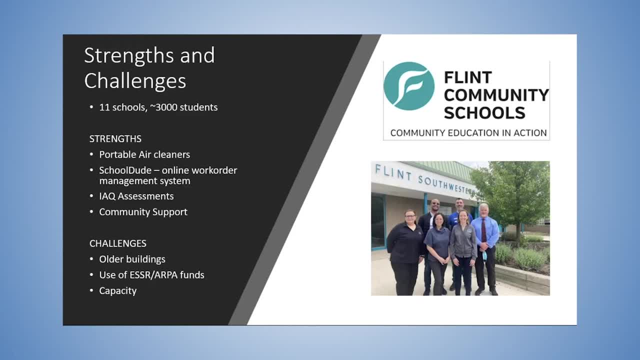 And With our maintenance program it's it's pretty modest and we utilize the school dude, which is our online work order management system, And with that that, the teachers, the secretaries and principals of each one of the buildings, when they come across an issue and identify it, they will submit that into school dude, which then we 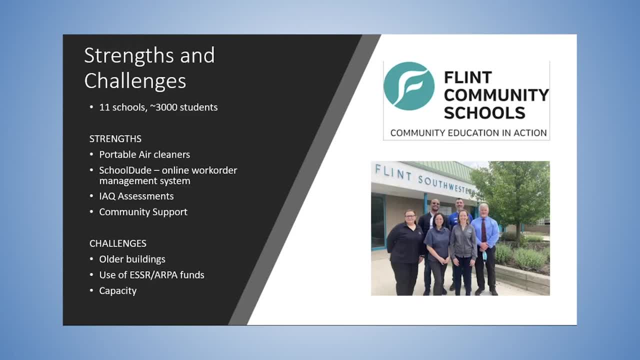 will direct, depending on the need to maintenance or custodial staff to to address the issue and the upon the onset of covid went because of the older buildings we have- they're average 66 years old- primarily a hot water or hot water boilers or steam boiler system which 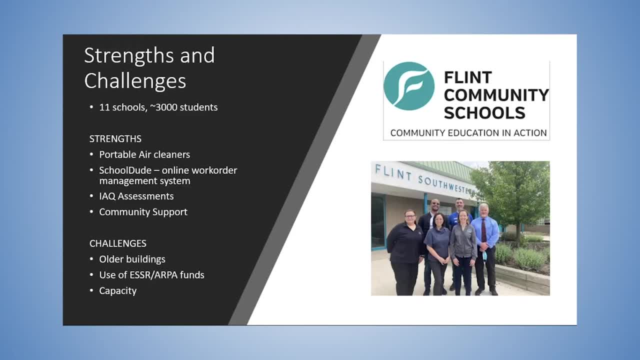 was running through the, through the buildings, into either radiators or into some kind of an air handling system. we really really had a minimum amount of airflow and, more importantly, air exchange. and they- my predecessor- went and did apparently some research, probably not enough, according to what some of the experts. 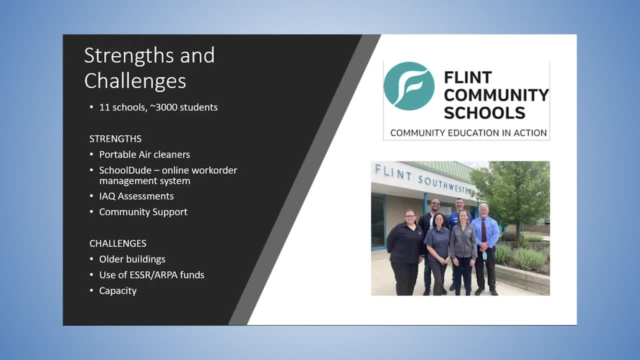 have told me, but they went with the itech ion stat, which is just a very small wall mounted unit and, as I found out as I looked into it further, that it does have emits ozone and in some type of a peroxide which I've been told by. 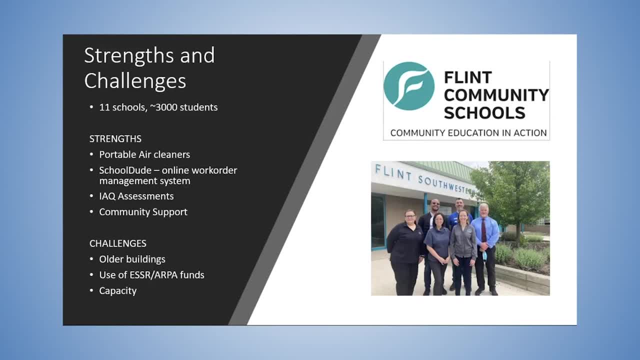 not just the EPA but anybody else that understands indoor air quality- that that's not a good recipe, especially with students with asthma and other respiratory issues. so I have, since realizing that, have been in that again research mode and I've heard many of the bans in the 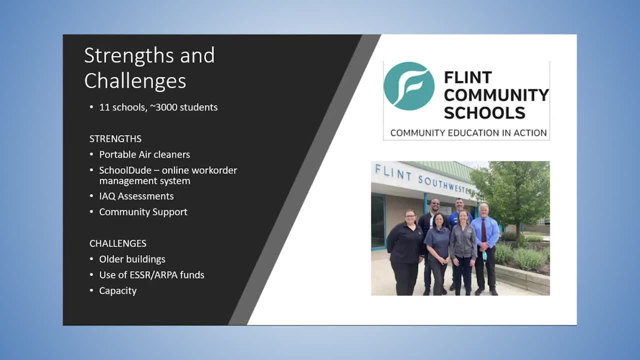 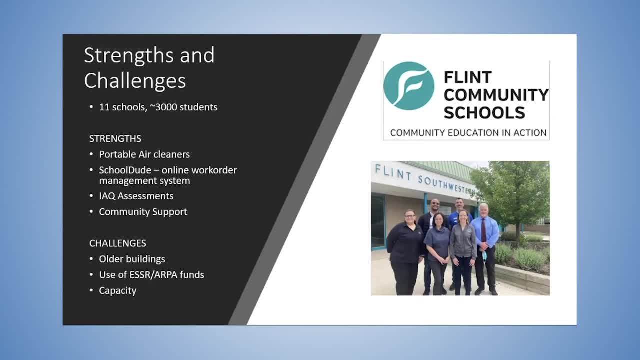 purifier, and in the buildings with the Honeywell. I guess because of the brand name and with the smaller rooms that we have, they let some people feel that that is an alternative to lease addressing, in trying to improve the air quality as much as we can, the schools themselves we have. 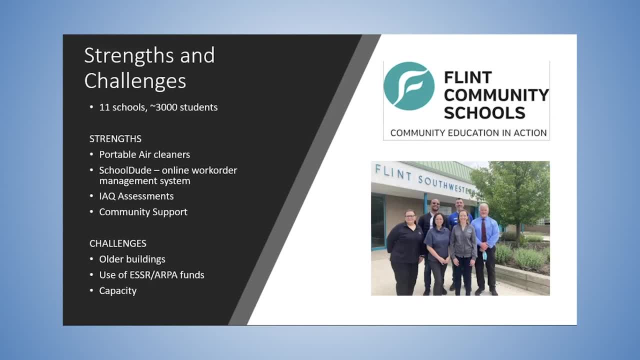 a contractor that changes our air filters for us and they have moved up to a MERV 10 as far as the the quality of the of the filter, which still allows adequate air flow and provides adequate filtering, and I have urged them to move it from four months as far as the filter change to three months and 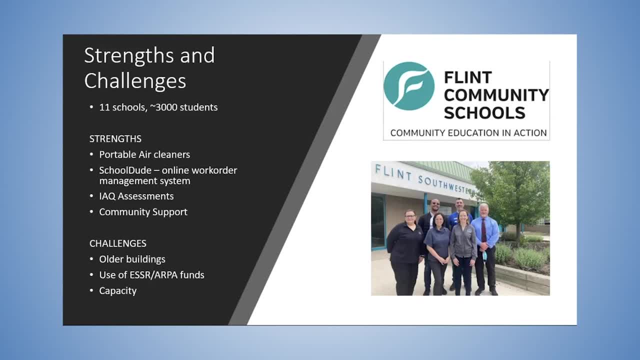 based on the information I've gotten from several of the zoom meetings that I've been involved with, I realize that the higher the the number is is key, especially with the air purifiers, which is one of the items I will be looking at when we do purchase ours. but 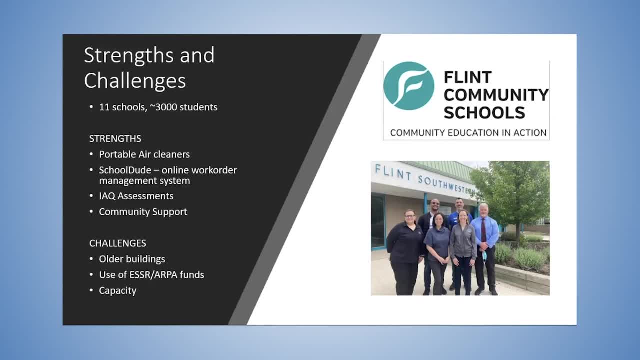 when you look at the old antiquated air systems that we do have. the MERV 10 is is what the school has decided to go with, at least in the interim. that's what our contractor is using, the. I'm really looking forward to the assessment that is being done by the EPA, and I do want to not only utilize that document, but 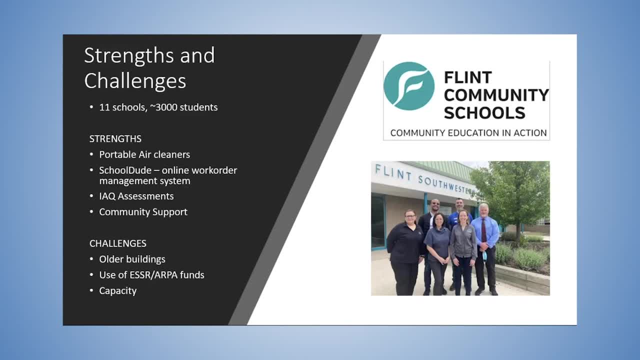 also to move forward with some indoor, indoor air quality testing to determine to what level we have to bring our standards up and with these older buildings, like I said, 66 years old, we have many, many challenges. these buildings have bad, very poor designed and maintained roofs. many of them are- almost all of them are leaking. so 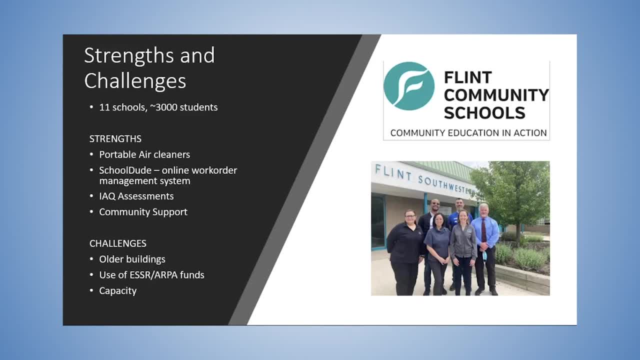 we got to address those issues which obviously affect the air quality, but especially with the air quality of the residential area, also the. we also need to purchase 250 air purifier here within the next month or so to to change out the the I-Tech ion stats that we currently have and to hopefully, when the kids come back to school in August- I think it's August 2nd- that we'll be ready for them. hopefully the pandemic will be quieted down and we won't have such a problem with it. 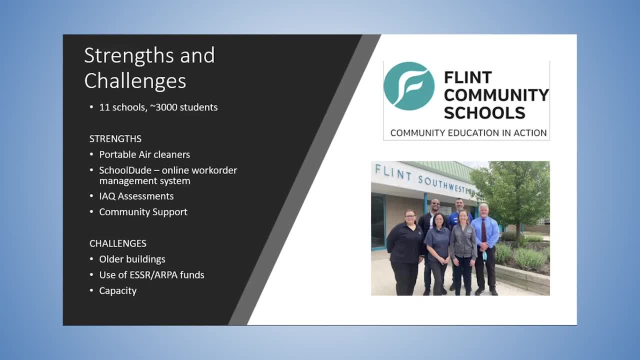 quiet it down and we won't have such such a big issue as we had in the recent past. but lastly, i want to be able to utilize whatever funding is available, which is a big part of why i'm involved here with this, with this discussion, and, of course, flint has esther. 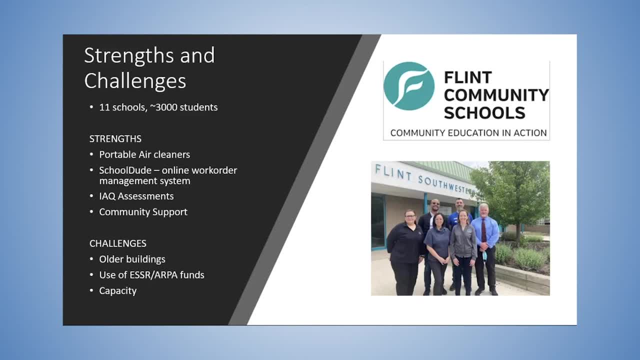 funds and the arpa funds, which will be. it will become valuable and the the challenge there is trying to retrofit hvac systems and and other air quality improving systems into these older buildings because they are so antiquated and basically wore out. that it's it's going to be. 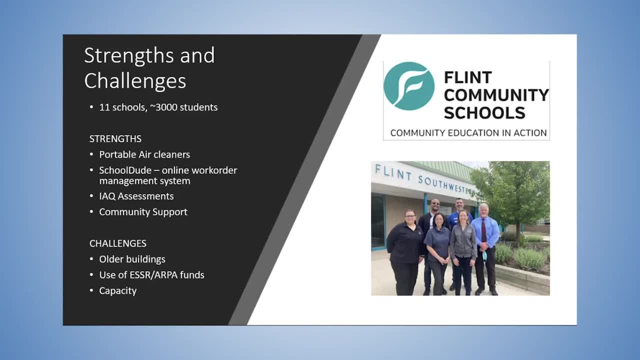 a challenge for any contractor to be able to retrofit their equipment to any of these buildings. so, having said all that, it is a real privilege to work for flint community schools. i have been here for a long time here, like i said, for eight years- and it is really a privilege to work with this group. 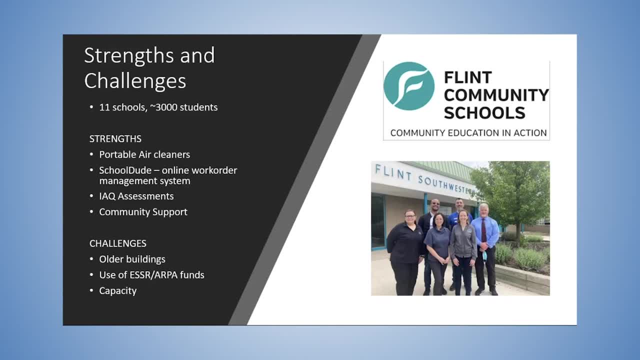 within earshot of me right now because i'm in that research learning mode and i just want to make sure we utilize our decision making to the best of our ability and utilize all the funding that is available to the best of our ability. so i'll sign off with that. i want to thanks. 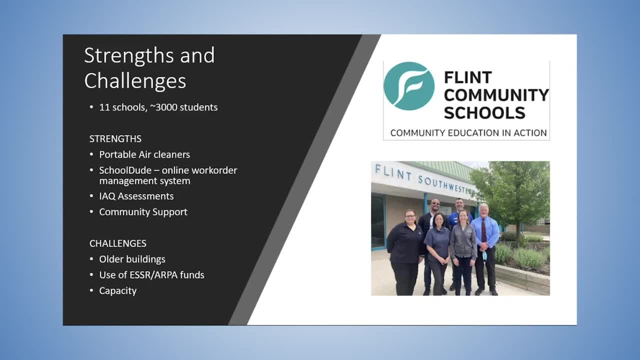 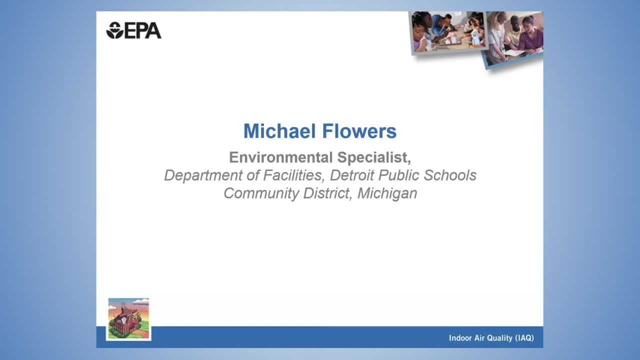 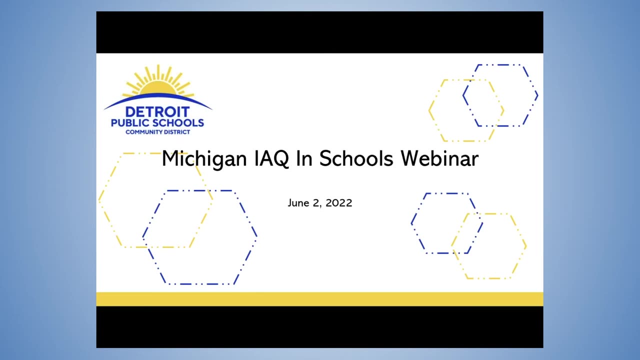 thanks again for all the great information you're providing me. have a good day, okay. next one: go ahead, mike, go ahead. all right, i'm going to try to make this as brief as possible. so good afternoon. my name is mike flowers. i'm the environment, health and safety uh inspector with montreal public schools community district, so just. 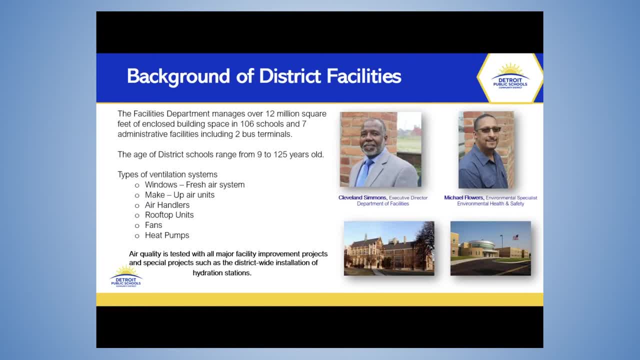 a brief background. the district manages over 12 million square square feet within close building space. that equates to 106 buildings, seven administrative facility buildings and two bus terminals, and our average uh age of our buildings range from nine to one hundred twenty five years old. on the bottom slide here it just shows the different types of ventilation systems. 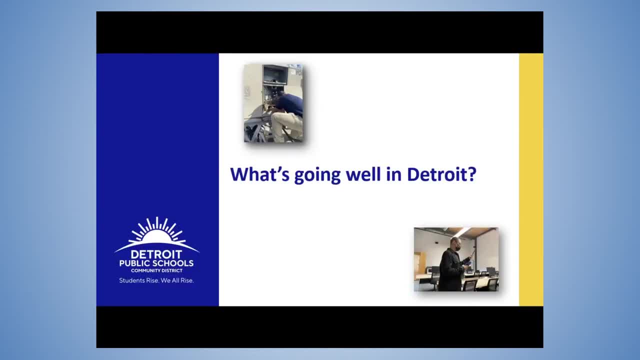 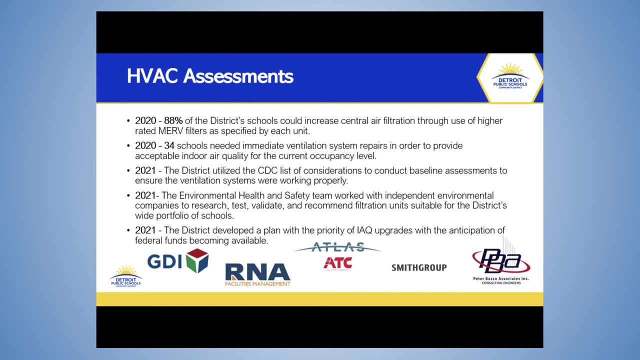 that the district utilizes all right well what's going well in detroit. so we conducted uh hvac assessments uh back in 2020 up until 21.. through that assessment uh, we found 88 percent of our buildings could increase central air filtration through the use of higher rated merv filters. 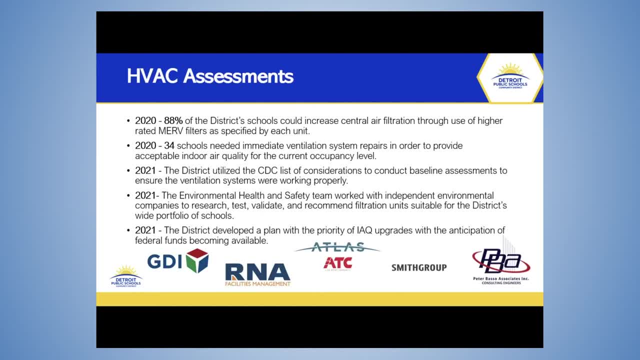 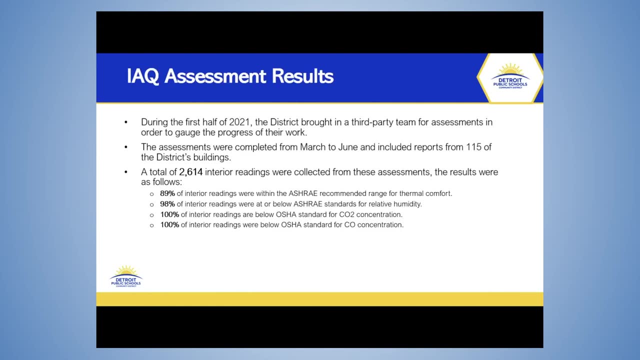 uh 34 schools needed immediate ventilation system repairs and uh the department or district developed a plan with uh priorities to upgrade uh these buildings with federal funds that were becoming available. so our indoor air quality assessment results showed 89 of our interior readings were within ashrae recommendations for thermal, that's temperature 98. 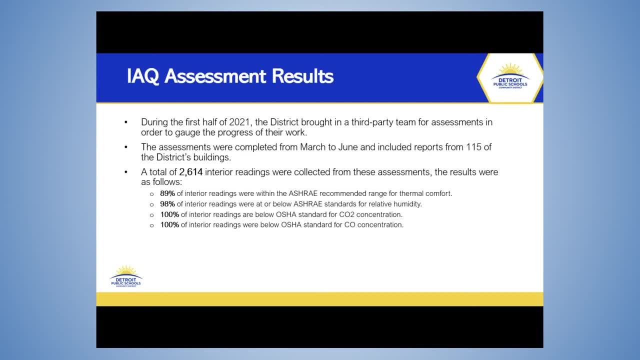 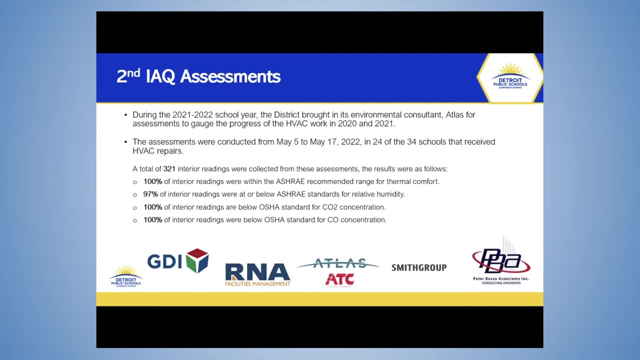 were below ashrae standards for relative humidity, 100 of our buildings were below osha standards for co2 and 100 were below standards for co for carbon monoxide. so, with that being said, we conducted a second indoor air quality assessment and an assessment of our hvac equipment on those 34 buildings. 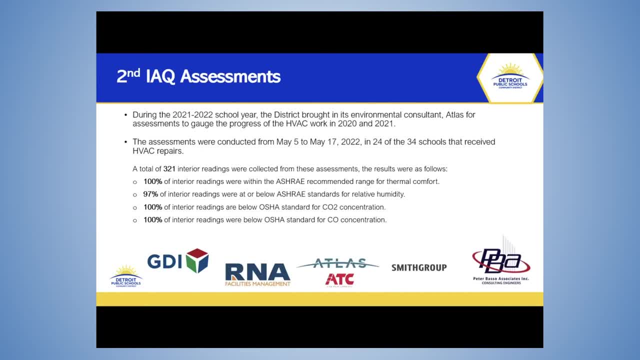 that needed immediate repairs back in our previous assessment in 2021.. so, with that being said, we conducted assessments in 24 of those 34 buildings. uh, a total of 321 interior readings were collected and a hundred percent of the readings were within ashrae standards for. 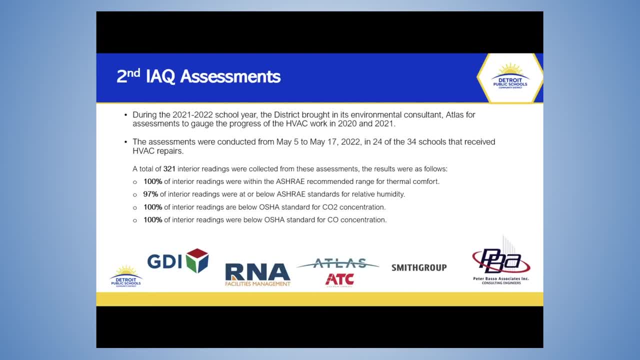 temperature 97 were within or below ashrae standards for relative humidity and we achieved 100 on both uh, co2 and co um with those readings. so the 97. we had one school that had some issues with some coils. those have since been repaired, so um, hopefully when we get these tested again, 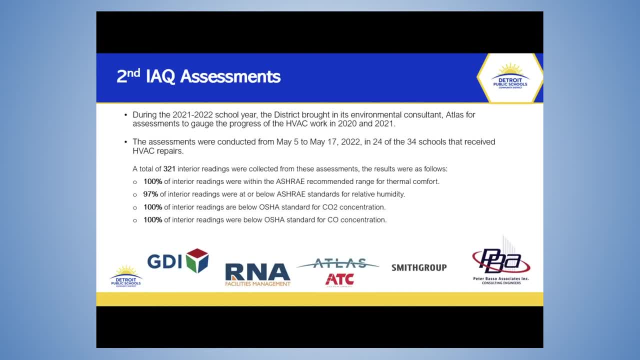 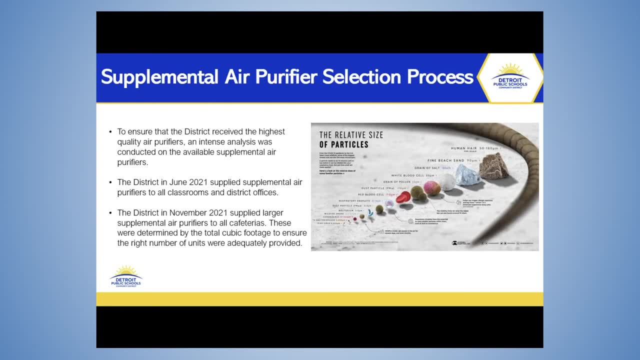 we'll achieve a hundred percent for all of those ratings. so our ongoing challenges. so with that you know the district. we looked at providing supplemental air purifiers for all of our classrooms and office spaces, and so we did an early analysis of several uh air purifiers that. 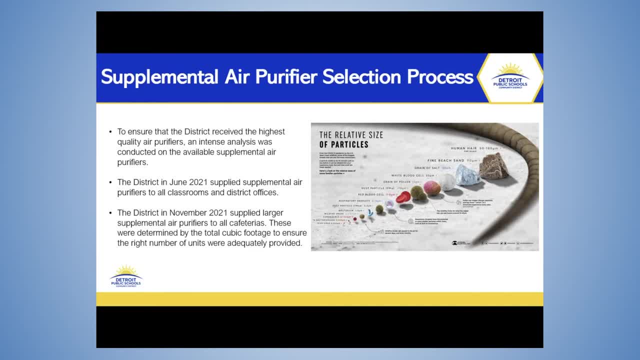 vendors had provided to us. so, um, the chart or the slide next to it shows a relative size of particles, and i think this was mentioned by stuart and some others earlier. so we were looking at. what are we trying to filter out? so we know that the code particle ranges anywhere from 0.06 micron. 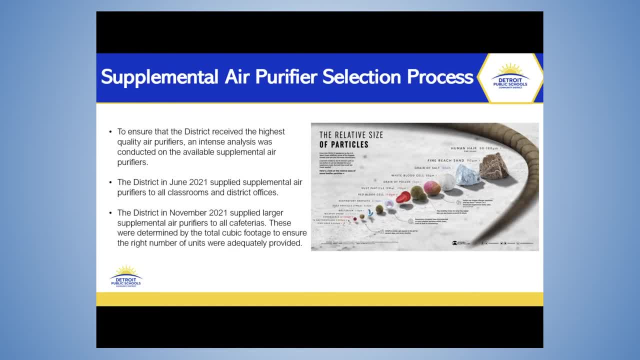 and your label and the absolute amount for us, which betrays- so we're addingiest- of only 1.4 micron, and then from 1.6 to ёз to 1.4 micro. for this example, that gave us 1.4 microns, so we were. looking at supplemental air purifiers that could filter down to 0.1, and those were the supplemental purifiers that had southern 13 filters. so there's a difference between true hepa and and hepa 13.. so true hepa, for example, would only go down to point three microns, whereas half of 13s will go down to. 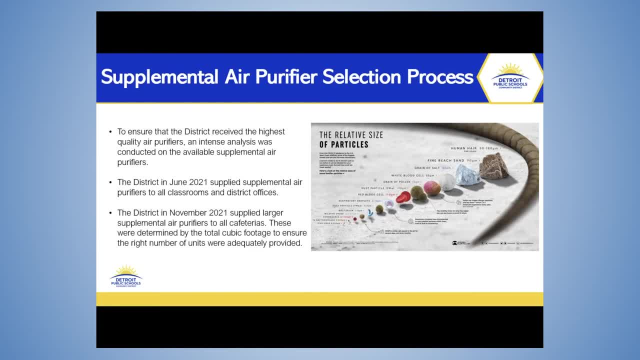 COVID particle, but you know the mid range to the large COVID particle size. So that's why we selected air purifiers that could achieve those goals for us Also, and then we started providing supplemental air purifiers in June of 21.. And then in November of 21,, the district 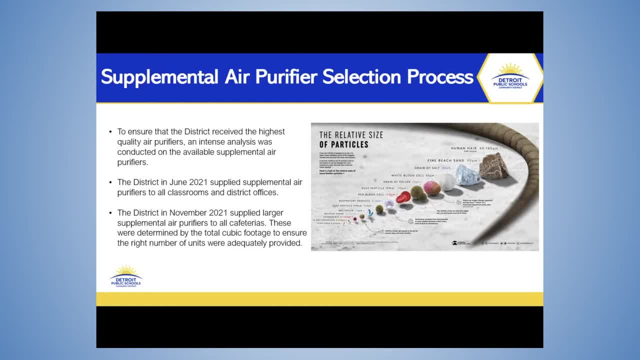 supplied larger air purifiers to our cafeterias, And this was determined through the total cubic footage of each of those cafeterias. So we wanted to right size the adequate number of air purifiers so that we were be achieving, you know, those filtration rates that we wanted. 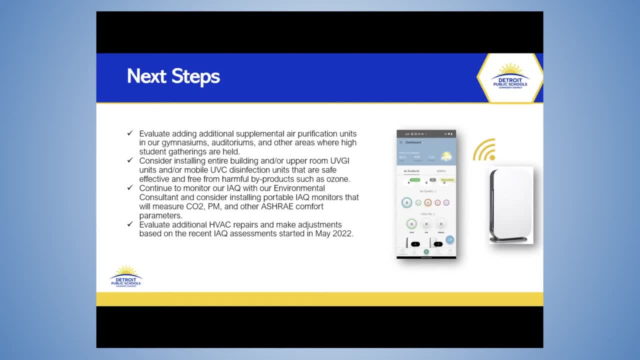 So our next steps are will be continued to evaluate adding additional supplemental air purification units to our gymnasiums, auditoriums and other areas where you have high student gatherings, And we're also considering installing entire building or upper room UVGI units. and 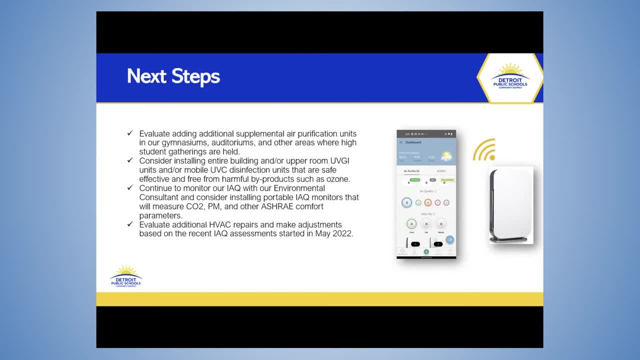 mobile units, UV disinfecting units that are safe and effective and that are free from harmful byproducts such as ozone, And we're also going to continue monitoring our indoor air quality with our environmental consultant. Right now, we're doing this on an annual basis And we're also 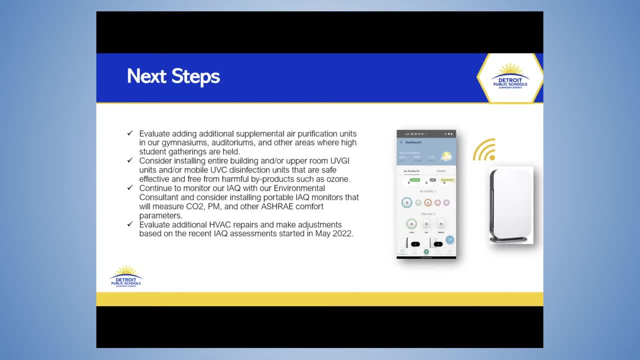 considering utilizing portable IAQ monitors that will measure CO2, particulate matter and other ASHRAE comfort parameters And, as I believe Dr Bateman Stewart mentioned CO2- a good indicator of if you're achieving your proper air exchanges. you know, in your 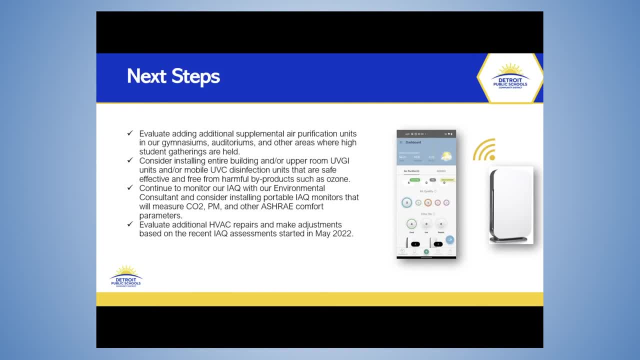 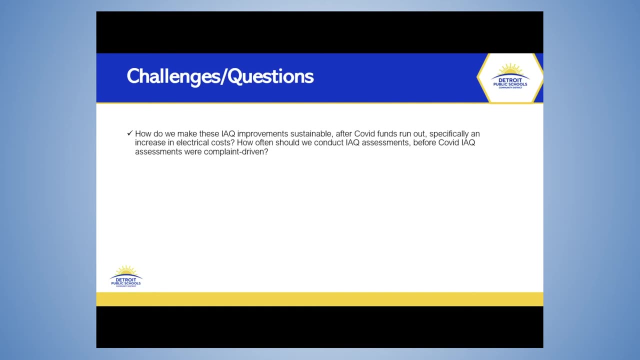 classrooms. And then we'll also continue to evaluate those HVAC repairs and just make adjustments based on our recent indoor air quality assessments that were just completed this May. So our challenge is, you know, for the district is how do we make these indoor air quality? 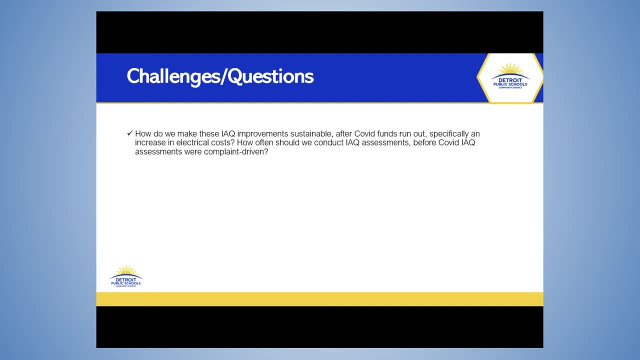 improvements, sustainable. So after COVID was run out, we're looking at, you know, increasing electrical costs. There's also going to be, you know the cost with, you know, changing our MERV filters. Right now, the district, we went from a six-month change out of our MERV 13s to now we're doing. 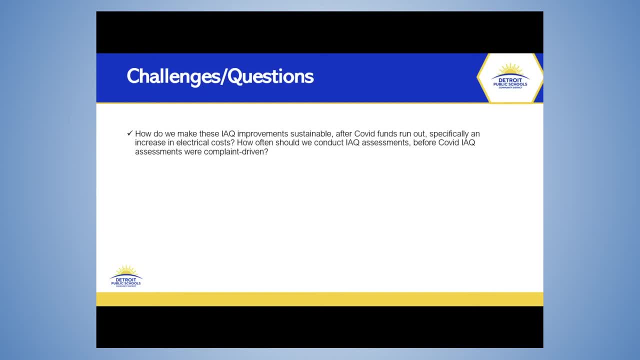 it 90 days for three months, So there's going to be an adequate increase in our cost to maintain these items and to operate them. And also, the question that I would propose to the panel is: you know, how often should we really be conducting these indoor air quality assessments? 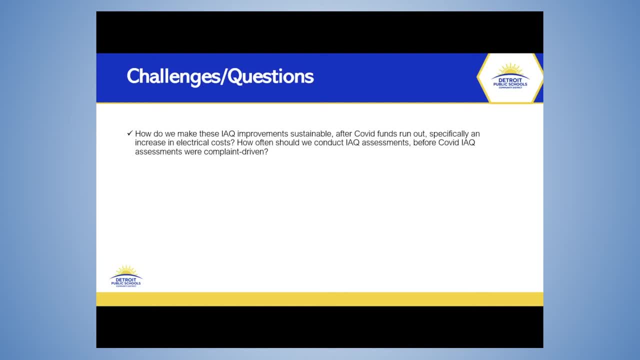 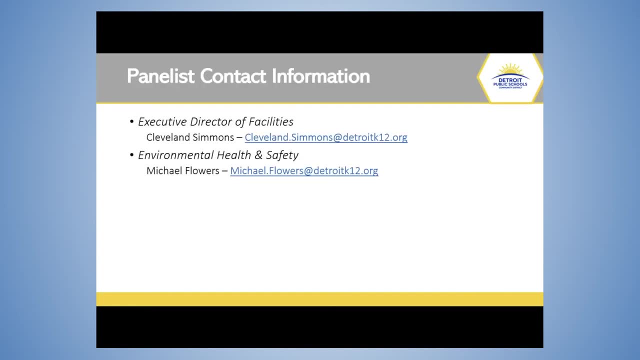 Again, you know we're doing it annually now, but prior to COVID the district would conduct these, you know, on a complaint-driven basis. This is just information for me and my director, Mike Simmons, Cleveland Simmons, And thank you. 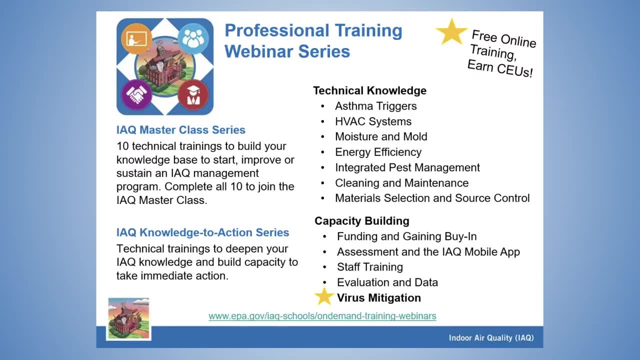 Hopefully I got this out here in some good time. All right, Thanks to everybody for staying with us here. Jeanette, Next up is Jeanette Marrero of my team. Good afternoon. Thank you for our speakers for great information, great presentations. 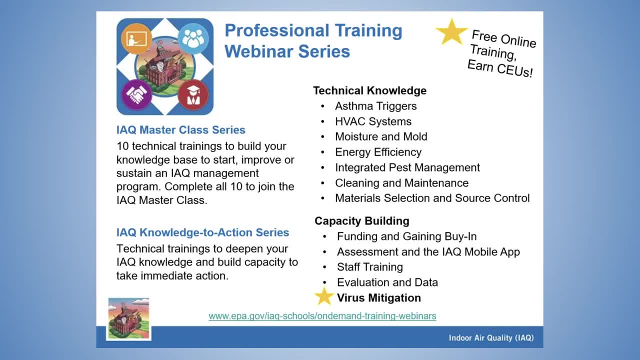 We heard information on planning and assessing two key drivers of our framework for successful indoor air quality management. I want to share information and other resources Region 5 offerings and make a request to help you move in a path of further learning and action. 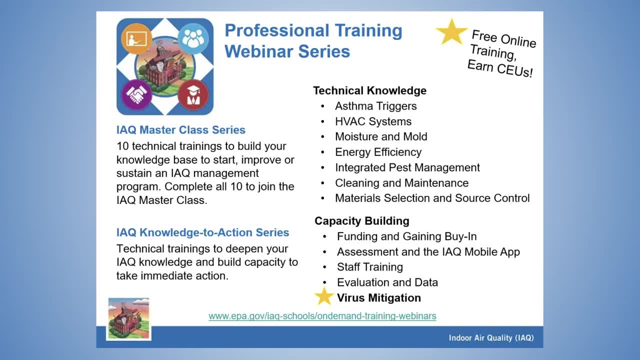 And in this slide you can see the professional training webinar series. It's a free ongoing series available online and on demand to view at your convenience. You can complete an evaluation and receive a certificate of completion. You can use this as a training program for your staff. 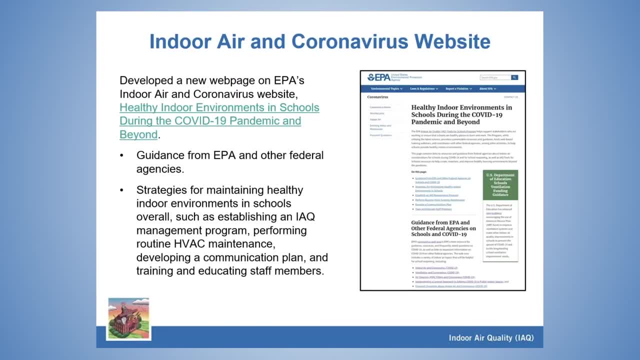 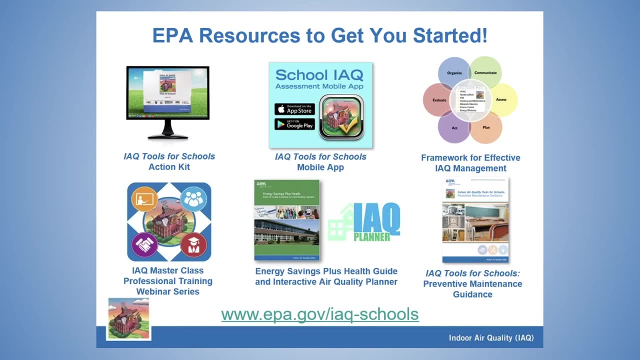 EPA has a dedicated website on indoor quality and coronavirus that provides strategies to maintain a healthy school. It includes a Q&A section and is constantly evolving, So please visit often. Here you can see our main indoor air quality schools website where you can find resources. 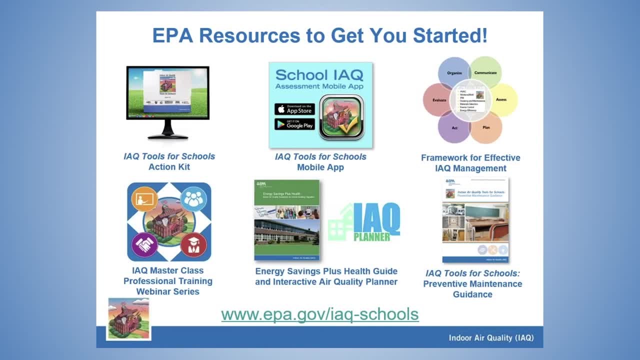 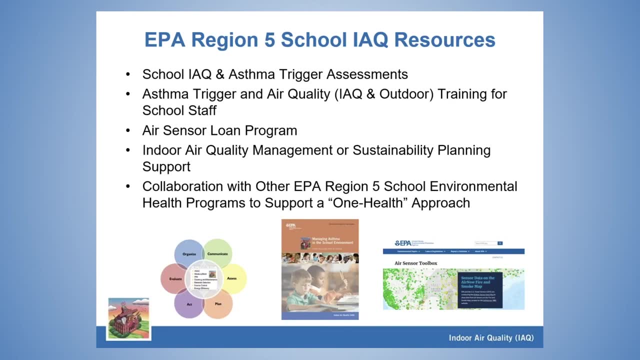 such as our mobile app guidance and resources. Thank you. Engineering cells and Energy and indoor quality, preventative maintenance and much more. EPA Region 5,, as it was mentioned before, has been working and assisting schools for many, many years. 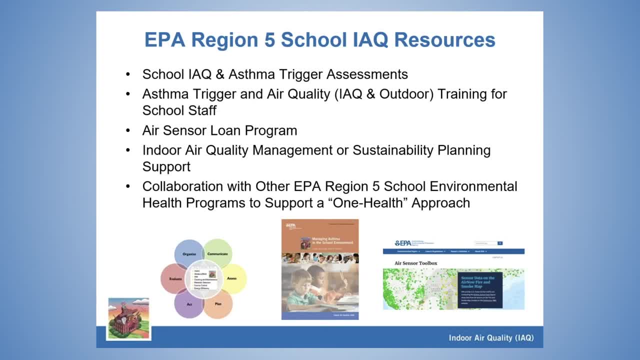 This is a list of the offerings that we have for schools. We conduct indoor quality assessments focused on asthma triggers and buildings, with a modified walk-through checklist to help identify better ways to manage indoor quality. We have focused on asthma and providing recommendations on preventative maintenance. 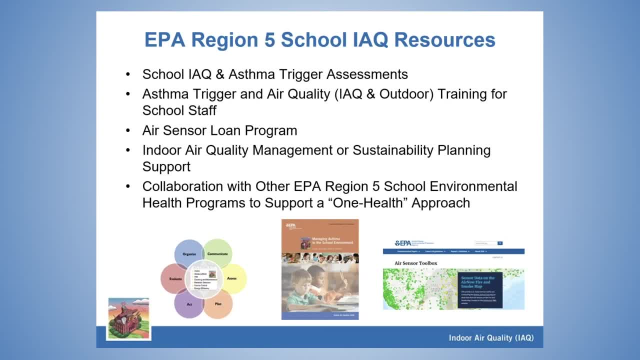 preventive maintenance practices, low-cost, no-cost solutions. We just conducted assessments in Flint and would like to do more in Michigan. We conduct training- train-the-trainer trainings- on different indoor quality topics- radon, mold, asthma triggers- and these could be customized for. 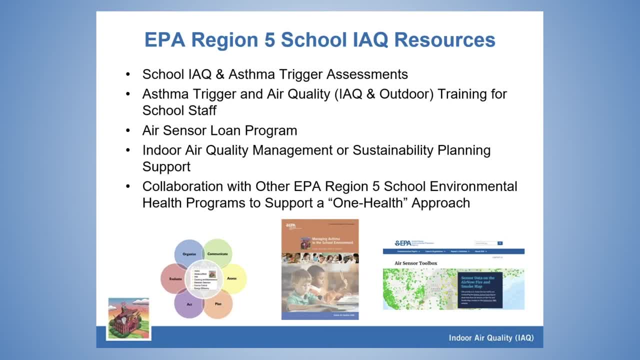 the different school audiences: school nurses, teachers, facilities and others. We also have our air sensors loan program, where individuals can borrow our sensors for up to a month and use them in different projects. We can help you create an indoor quality management plan working with. 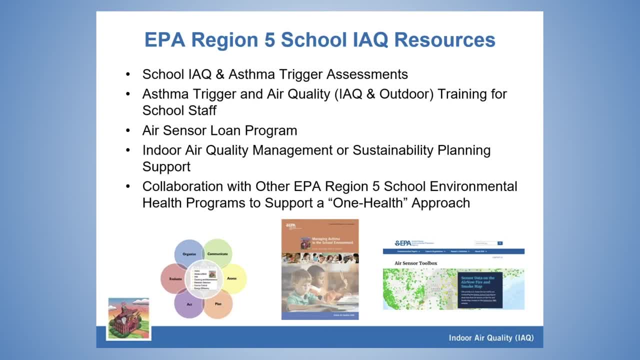 you on key drivers and technical solutions. We don't do this alone. We have a one-help approach where we can work in Region 5 with other staff working on school-related programs. These are some of the programs that we have for outdoor air: the FLAG program, where FLAG is raised. 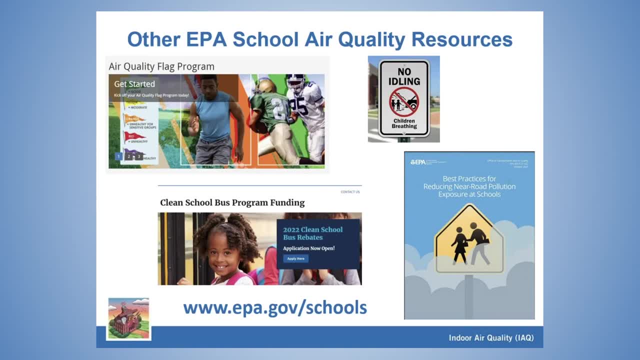 based on the Air Quality Index to inform the community at large. clean school buses that provide funding to retrofit and purchase fuel-efficient buses, and best practices for near-road schools. As you can see, some of these, even though they're outdoor, it can have an impact on indoor. There are other environmental health. 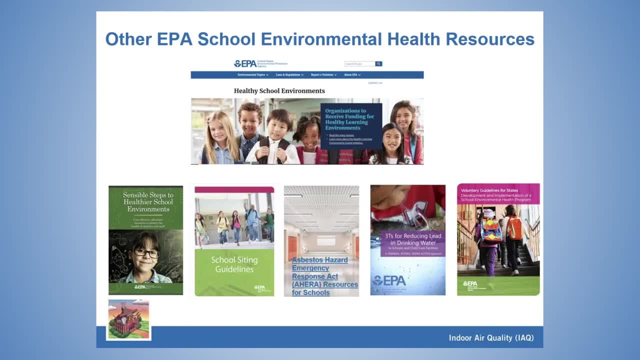 resources addressing different topics, such as integrated pest management, drinking water, lead and energy. The Sensible Steps documents that you can see in the picture in the slide has a checklist that was recently updated and could be filled in electronically that address your needs. Please check it out. Our environmental education resources include student awards. 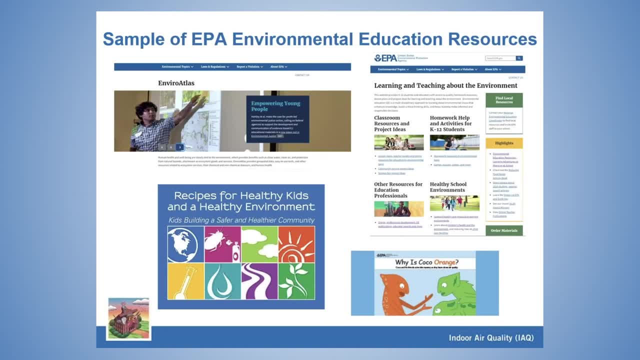 grants for projects, lessons plans and lots of information for students. As you can see, there are many, many resources, many topics, and we can help you navigate the many resources to fulfill your needs. You will be receiving a certificate of completion for attending. 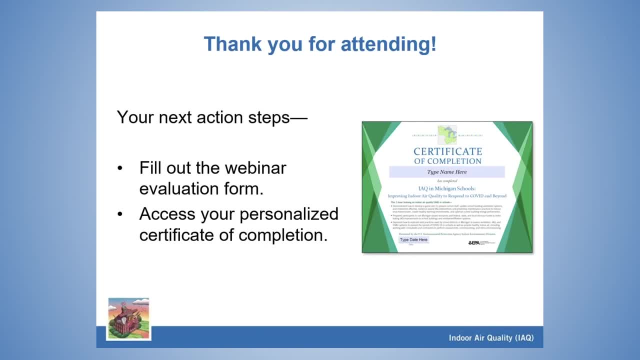 today's webinar. My final request is for you to fill out the evaluation form to help us better serve and support your students. Thank you so much for attending today's webinar. My final request is for you to fill out the evaluation form to help us better serve and support your students. 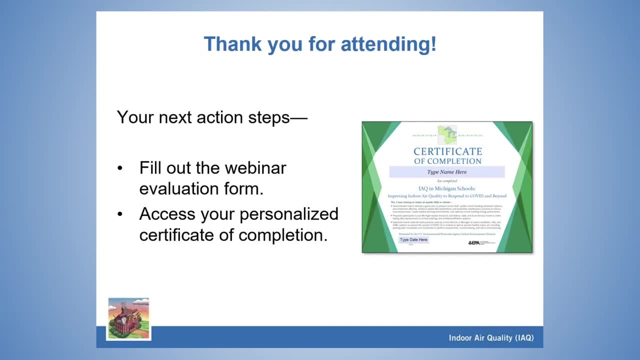 We created a questionnaire that will help you assess where you are and take advantage of our Region 5 offerings. We want you to develop a game plan to manage indoor quality. We want you to use Michigan-based resources and be able to replicate best practices. We. 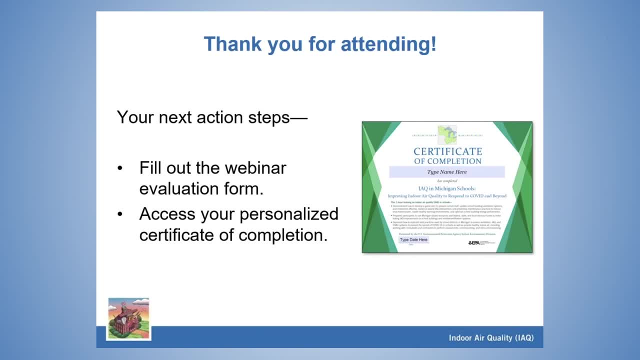 anyway, that will be available and if you don't have it you can also collect it from us at the Department of Dr Junkers told us that the budget might be reduced to about 45,000 dollars off the drug market, such as fivek, to send service to the Indian community. 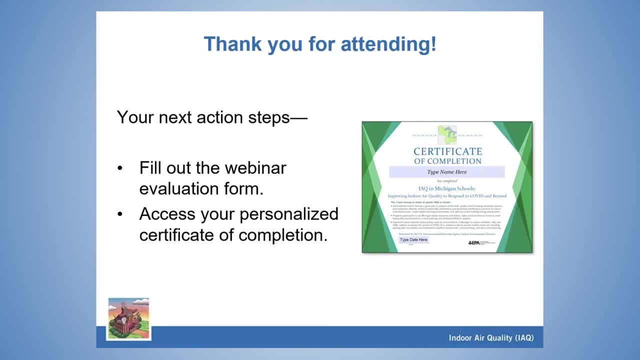 at the local level. Next day we'll show you how this strategy can be implemented better. Please complete the form to let us know. Thanks so much for attending. We've been here the whole country, So write in this things at the Department of Drug Safetyoton. We'll leave it at that. 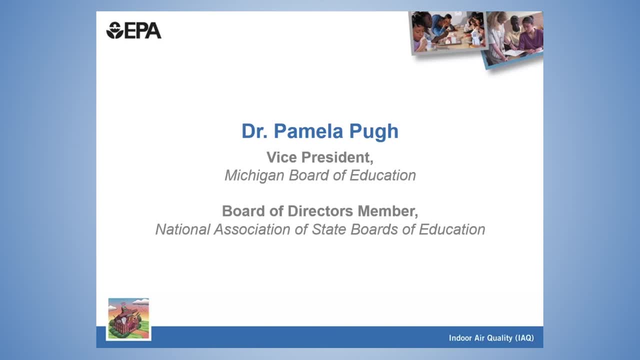 portion of the webinar. i will invite now my colleague, tracy washington anchor, to join us to facilitate the qa session. thank you, and thank you, uh, jeanette, and and thanks to all of our speakers. um, we had a robust slate of speakers here and um and a robust set of 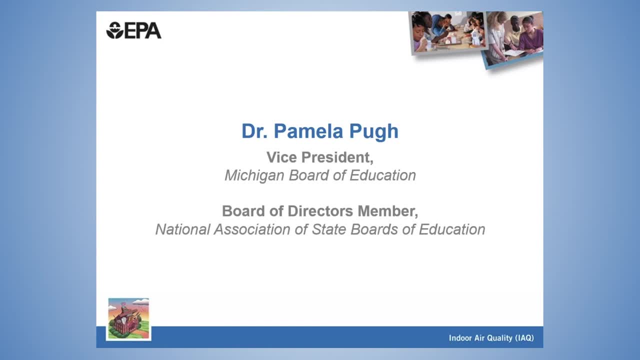 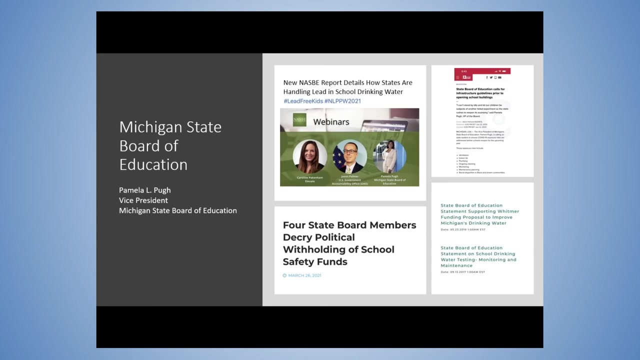 information and before we we conclude, um just want to say that many of your questions were actually addressed during the, the content of the, of the presentations and the webinars, but i do want to invite um dr pam pew to give some, uh, some closing remarks for us here. pam is the vice. 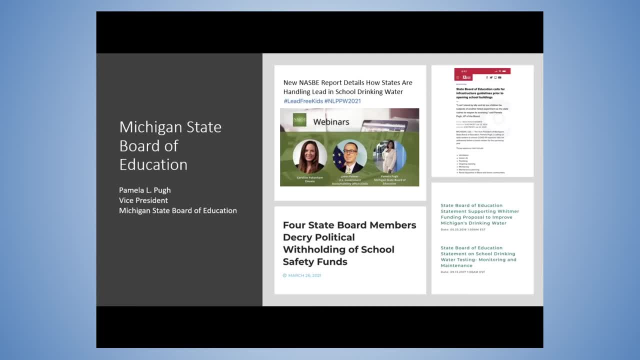 president of the michigan state board of education and um, and such a tremendous champion, so, pam please. good afternoon, and what a great set of panelists. um, and i really am um happy to hear all of the work that is going forward and i truly um and i'm appreciative to mike and don and 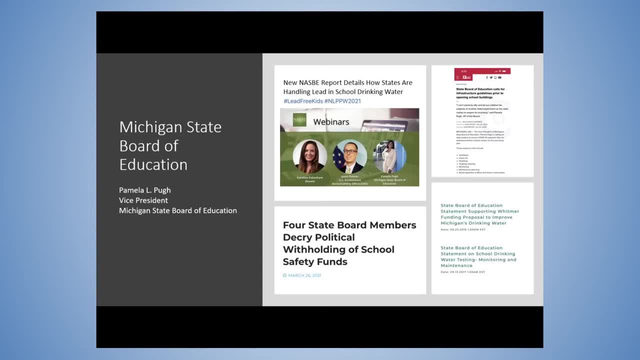 peter, who are on the ground making sure that our children um are safe. but we know that we need real solutions. we need coordinated solutions, we need adequately funded solutions and we need this type of tech support that the epa provides. so, as mentioned, i am an elected board member to 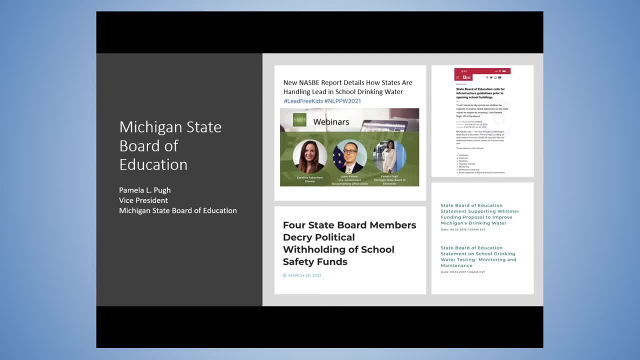 the state board of education. michigan is unique in that we elect our members of the board statewide and we are responsible for leadership and over oversight of schools- all schools, public education in the state of michigan and some of the things that we've been working on. we learned a lot. 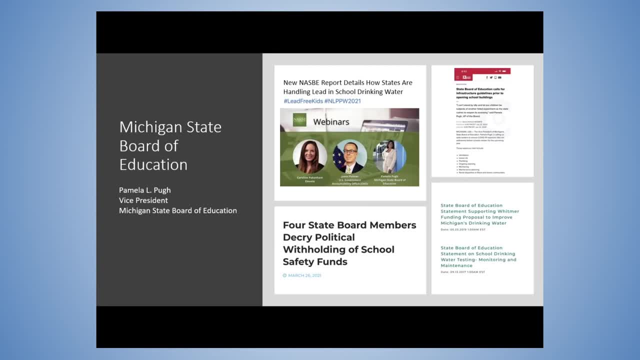 um at post the flint water crisis. uh, back in 2017, we came back as a bipartisan body and we really talked about a comprehensive approach, uh to addressing drinking water. we learned a lot, i think some of the things that came up is that you can provide money, but if you don't have the 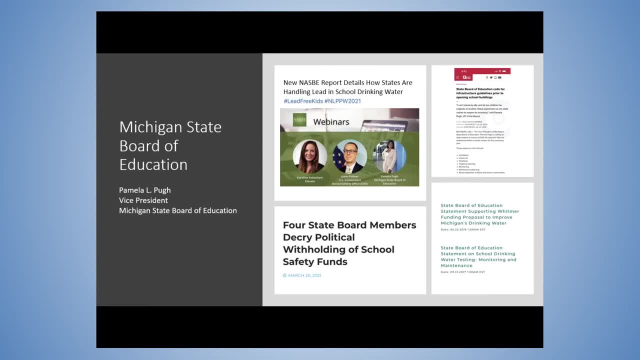 technical support, uh for that, for those funds to be adequately used. um, then it then it's hard to spin up that funding, so we will be advocating, as we started two years ago, uh, the state board of education. my, uh, some of my board members and i have a lot of experience with the state of michigan and the state of flint water crisis. 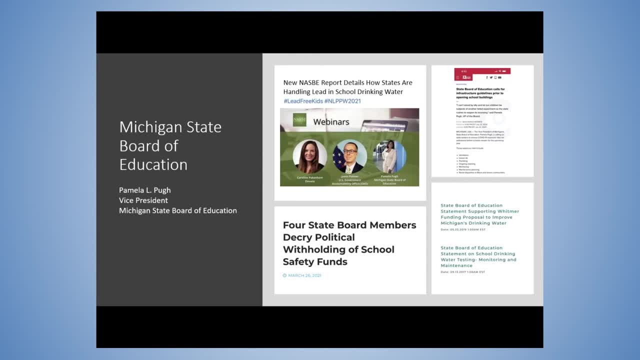 and we're really looking forward to working with the state of michigan and the state of flint water crisis to really look at how we can provide funding for that, and we're so happy, uh, that the governor did provide funding for that and, uh, we're also advocating for adequate funding. 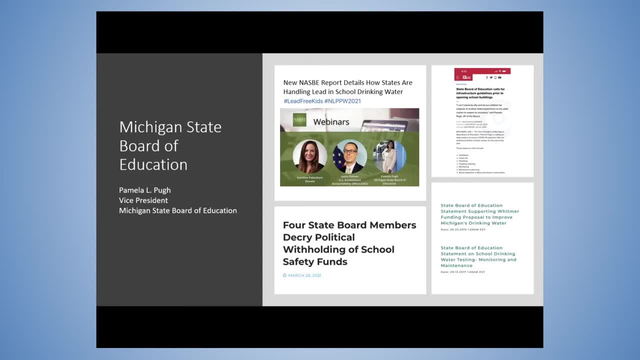 uh to to carry on, just uh. as i believe it was mike said, we have to be able to uh make sure that we have the time to spend this funding. as regina mentioned, uh, we don't have to have um all the parts. uh, we don't even have um all of the expertise to be able to do all of the. 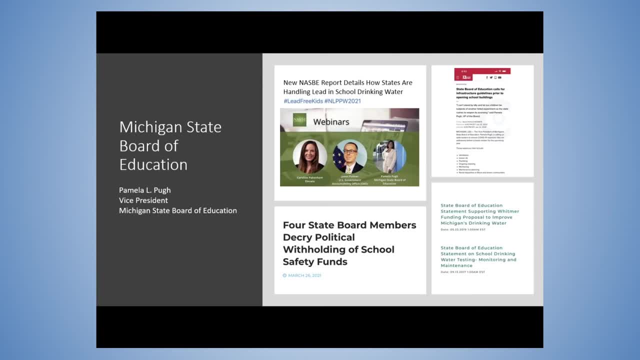 work um that the funding provides us to do so, we're we will advocate for um the adequate time for that funding to be spent, but, as um the governor has put in in her budget um opportunity for additional funding to address, uh, some of these issues that we're talking about here today, we will 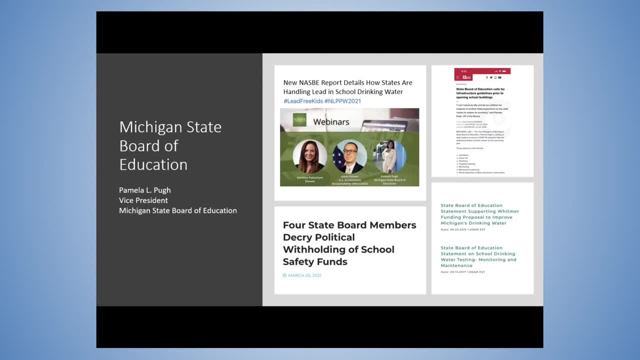 continue to advocate and advocate uh with uh folks across the state and our legislature to do that. but i just want to thank um the epa, because we know, with your 20 decades of experience, we need to make sure that your voice comes across loudly and clearly in this space. we know that we have. 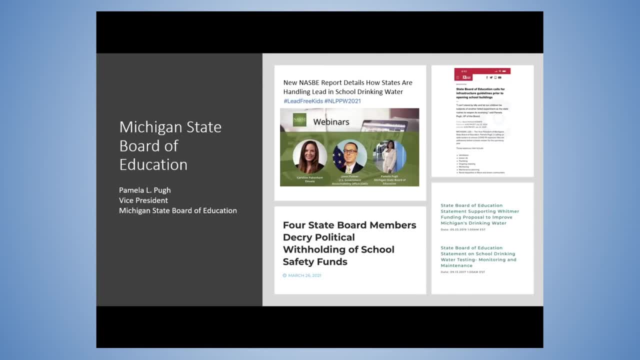 centers for disease control. we have the us department of ed, but without the epa providing support for the health and safety of our children. uh, that's what it is, um, that's what we're doing to make sure that all of our children are safe. so i just wanted to thank you guys for the support. 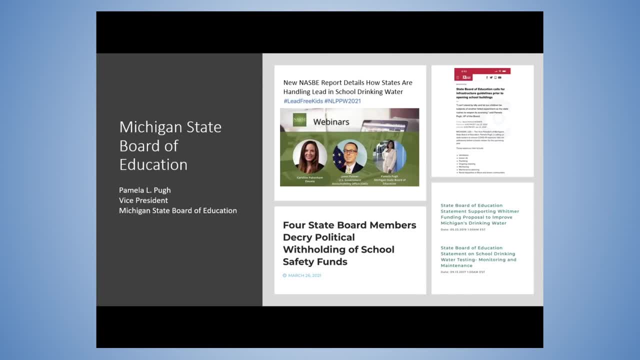 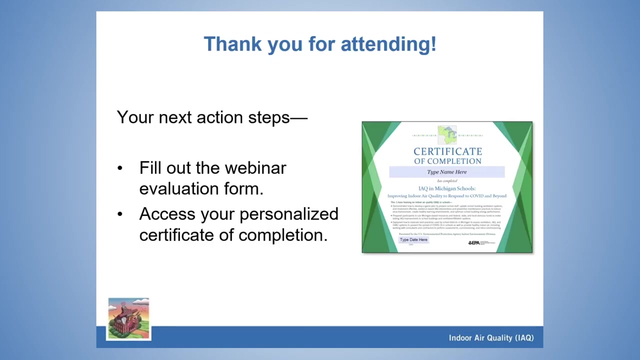 and i had a couple more questions that come in and those questions as well. so we are in the current crisis, they're starting to bounce off the And thank you, Pam, and thanks to all of our speakers, And I just want to reiterate: definitely. 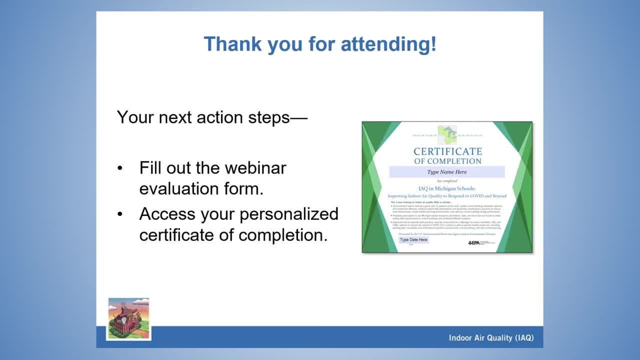 here at the Environmental Protection Agency and, as you have heard throughout this webinar, along with our friends at Department of Energy, who are providing all kinds of on-the-ground technical assistance to help with indoor air quality improvements and energy efficiency, through both the access to technical subject matter experts. 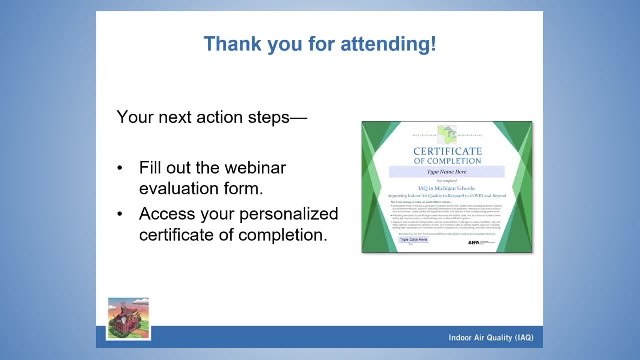 as well as grant funding, And so there are links in the chat where you can get more information about that, along with our friends at Department of Ed, who are also putting that funding out there and providing that kinds of support, and at CDC, But really it is our regional staff. 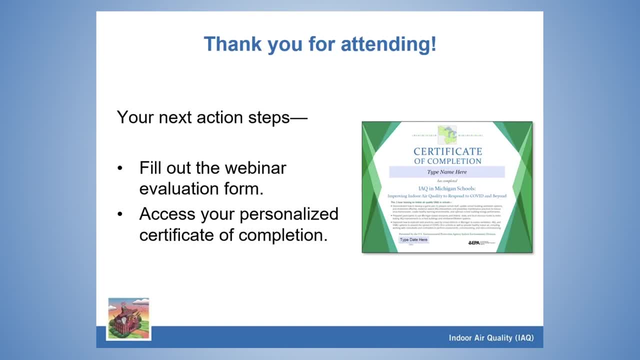 with the partners that you've heard them working with here at ASHRAE and at University of Michigan, and certainly the amazing leading champion school districts who joined us today to share their stories and their support and their mentorship. That is what really makes this program continue to work. 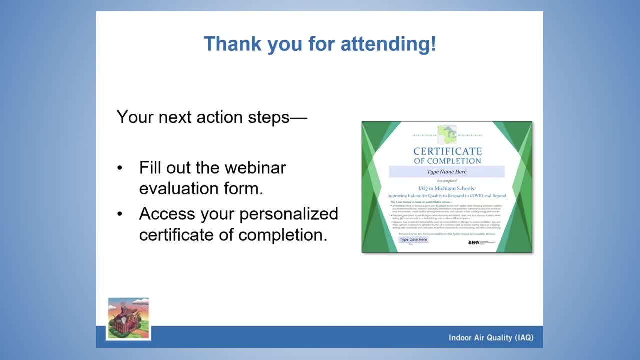 And so I would just implore you to avail yourself of these partners, of these assets and of these resources that are available there in Michigan, especially our friends at Michigan Eagle who are providing that kind of assessment, especially our students who are providing that kind of assessment. 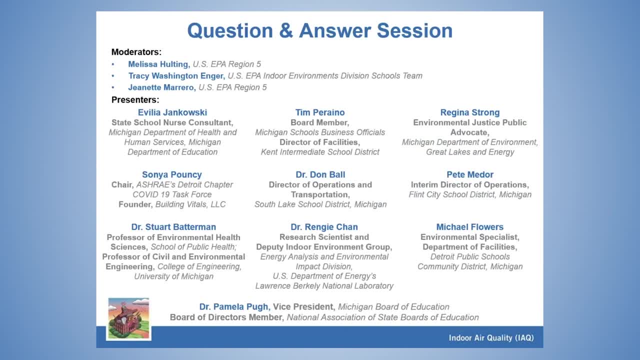 And so you know, one of the questions that we had from Mike Flowers there in Detroit was: how often should we be doing this? How often should we be doing these IAQ assessments? You know, previous to COVID, people were doing them on an ad hoc or ad needed basis. 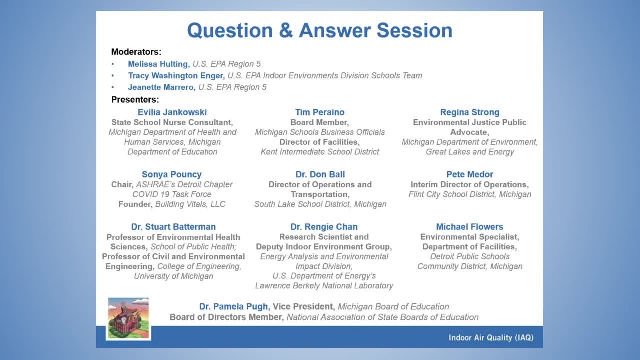 But what have we heard so clearly about the importance of preventative maintenance and proactive activity? If you can build in those annual overall assessments of your facilities, then it will have you poised for the next event that comes up, because we know COVID will not be the last airborne challenge that we have in our schools. 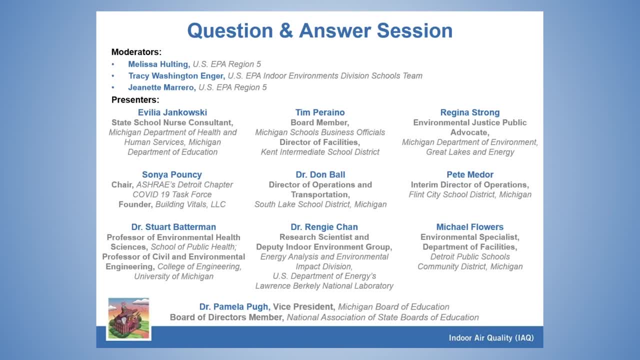 It wasn't the first and it won't be the last. So, as I've been saying, you know, these last few months, this is a moment that we have, that has come Thanks to us by COVID. this moment is turning into a movement because of all of the actions that you are taking within your schools and your school districts. 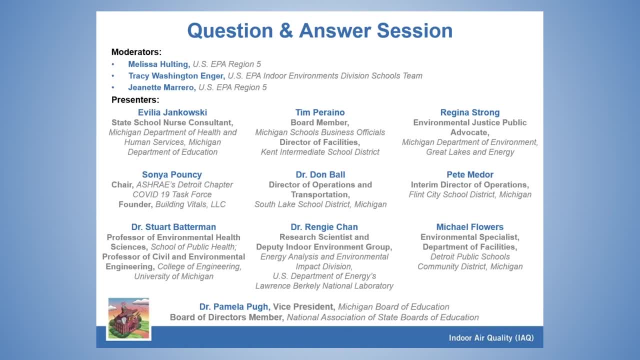 But we can turn it into a monument of improved indoor quality, improved health and performance for all of our staff and students. Take this moment, this thing coming in movement, and let's make it a monument. We can do it And with the support that you have there in Michigan to do the assessments, do the planning, prioritize these efforts.